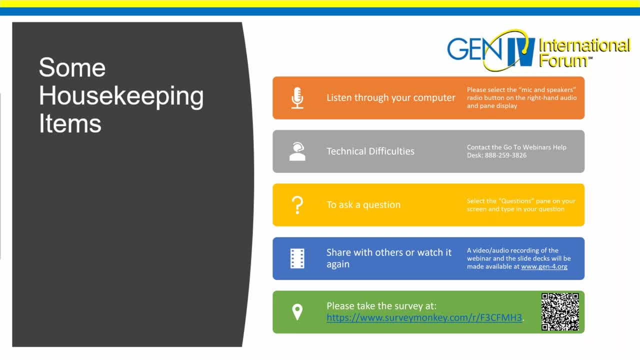 GIF webinars and the upcoming webinars through November 2020.. So an information brochure for you. Last but not least, on the screen is a link to SurveyMonkey, a brief survey. There's also the QR code for people on mobile devices. It's a little easier, perhaps We. 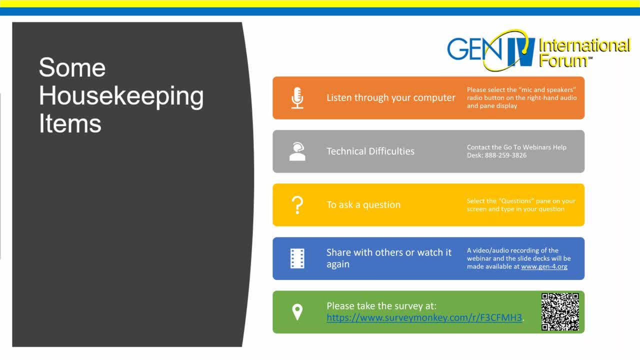 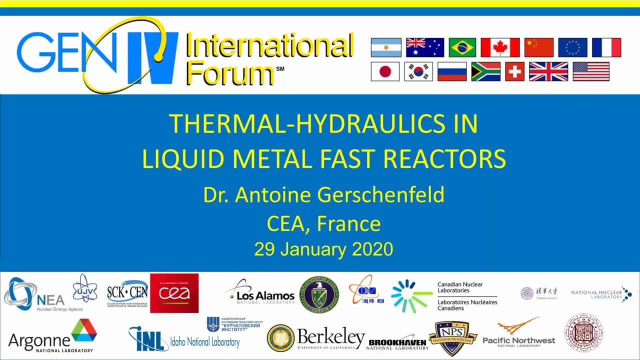 do appreciate your feedback and requests. If you have any questions, please feel free to reach out to us. If you take just a few minutes following today's presentation, it helps us improve the webinars and get your input. We do take your input very graciously. 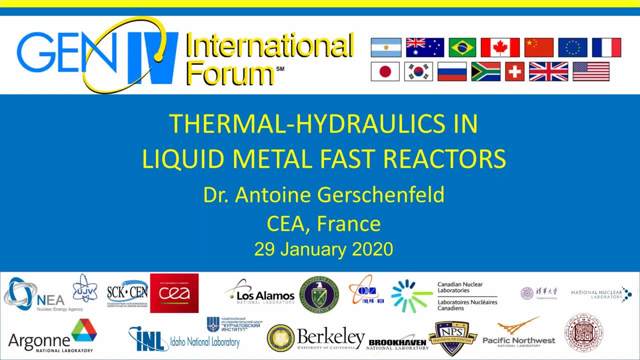 Doing the introduction today is Dr Patricia Pabier. Patricia is the Technical Group Manager of the Radiological Materials Group in the Nuclear Sciences Division at Pacific Northwest National Laboratory. She's also the Chair of the GEN4 International Forum Education and Training Task Force. So without further delay, I give you Patricia. 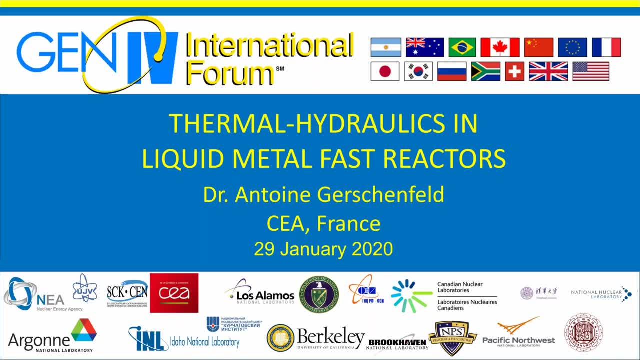 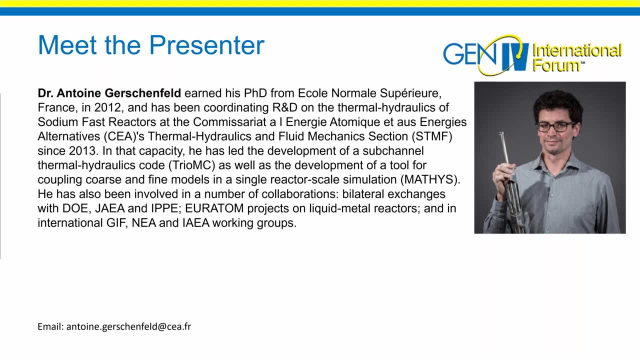 Thank you so much, Bertha. Good morning everyone And good morning Antoine. Thank you again for volunteering to give this webinar. So Dr Antoine Gershenfeld obtained his PhD from l'Ecole Normale Supérieure in France in 2012,, and he has been coordinating R&D. 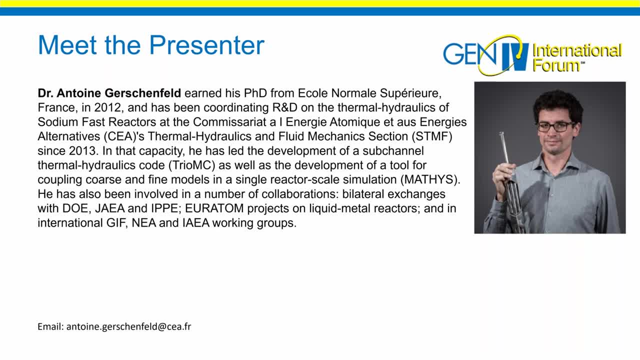 on the thermal hydraulics of sodium fast reactor at the CEA Thermal Hydraulics and Fluid Mechanics Section since 2013.. In that capacity, he has led the development of a sub-channel thermostatic reactor. He has also been involved in a number of collaborations, bilateral exchanges with projects on liquid. 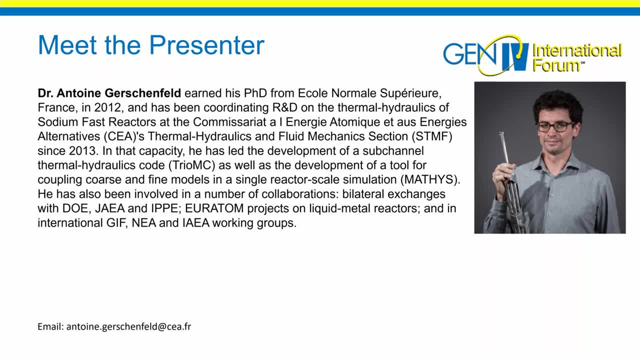 metal reactors with the DOE, JAEA, IPPE and Euratom. And finally, he's very involved in international working groups, including the International Working Groups and the GEN4 International Forum, the Nuclear Energy Agency and the International Atomic Energy. 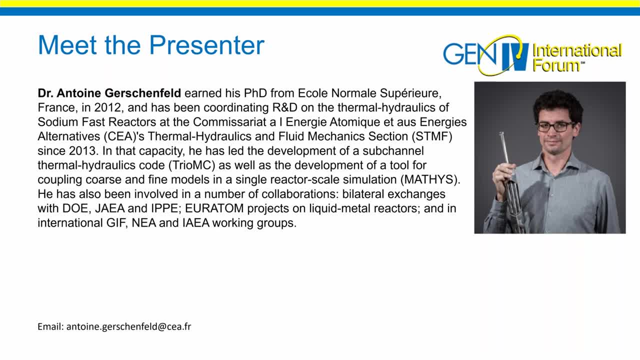 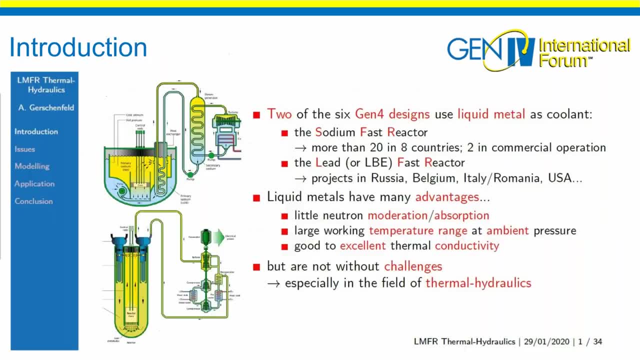 Agency. Thank you again, Antoine, for volunteering to give this webinar And, without any delay, I give you the floor, Thank you. Thank you, Patricia, for this very kind introduction And good morning everyone, And thanks for connecting to this webinar on sodium fast. 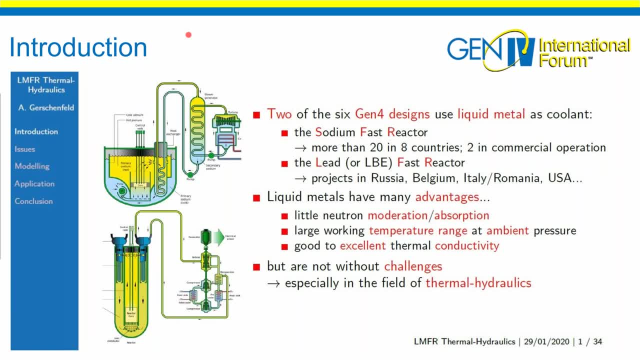 reactor from l'Ecole, And so I'll start immediately. So this webinar will be about the energy, and immediately so. so, as many of you probably know as well, one third of all of our sixth generation for designs in the generation 40, in the generation for 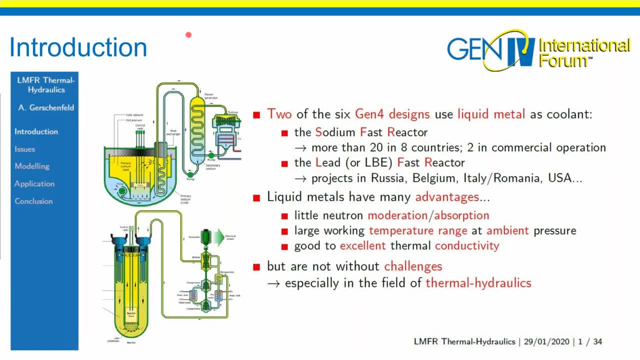 forums actually use liquid metal as a coolant. so one of the two is the sodium fast reactor and this is actually a design that has been tested and put that and put into practice as in at the industrial scale a number of times. so there's: there have been 20 years efforts in as much as eight countries. 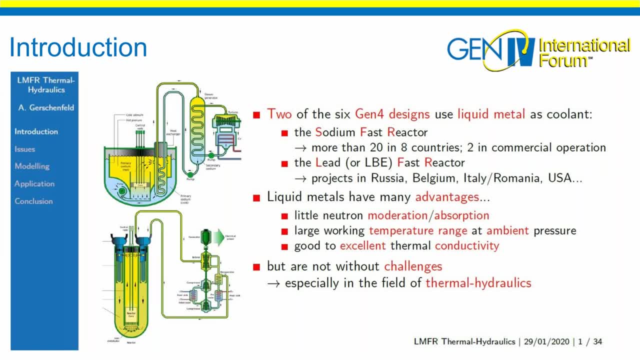 and currently we have two in commercial use in Russia and the second gen for design that uses the queen metal is the lead fast reactor, so the LFR and this one as active project in Russia as well in Belgium and in collaboration between Italy and Romania. and, of course, the reason that we have two designs using 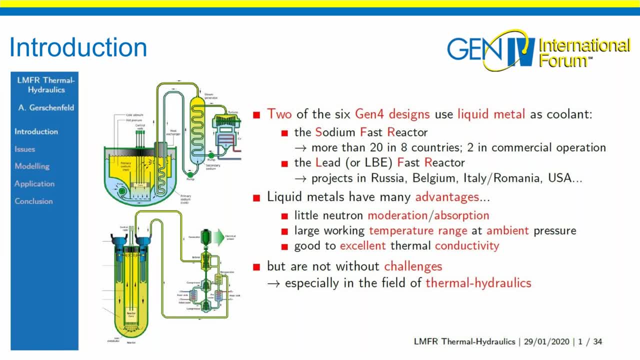 liquid metals is that they have a number of advantages over, for instance, water. the first is that they have a number of advantages over, for instance, water. the first one is that they have good new 20 properties for fast reactors, so little little moderation, small absorption. the other thing is that they have a very 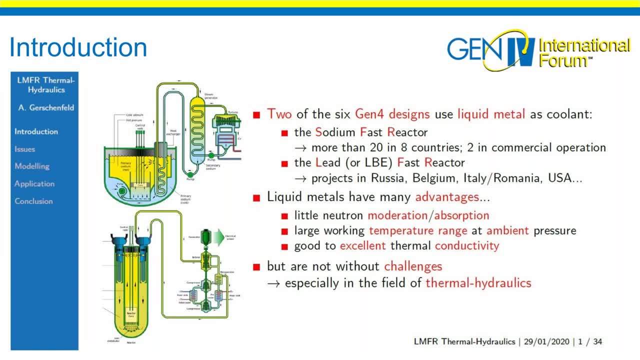 large temperature working range at ambient pressure. so usually they, for instance sodiums, become, becomes liquid at around 100 Celsius and remains liquid until around 900. so we've got 800 degrees of temperature range and with that it's even better. and the next thing is that they are very good thermal conductivity. so they are. 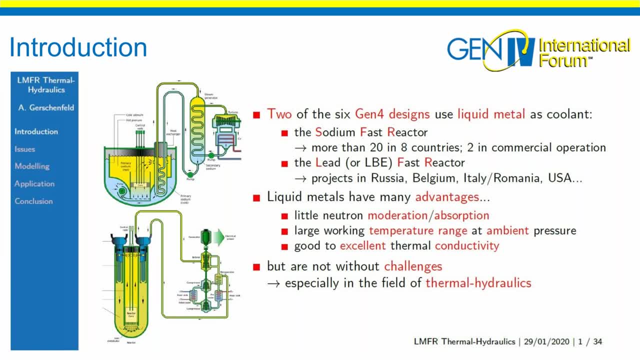 very useful as heat transport through. but at the same time they come with their own challenges and one of the regions where where the where they are specific challenges is in thermal hydraulics. so the behavior of heat and heat and momentum transfers in the field. so first, what is from what is from an 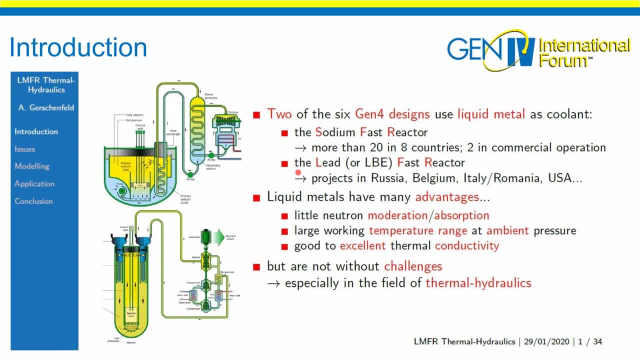 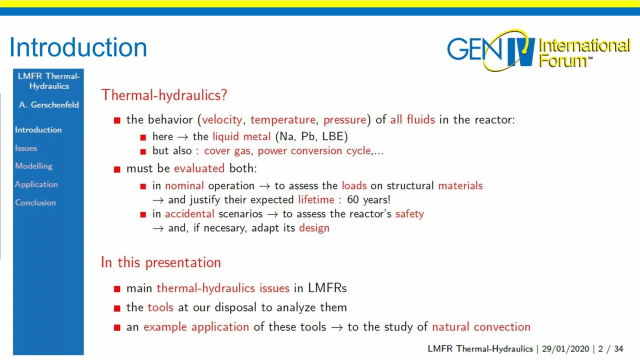 hydraulics, exactly. So it's almost working. let's see to advance the sides. So this, can you advance me better? sorry, Yeah, And Thank you so much. So, thermal hydraulics, that's the behavior of the fluid in the reactor, more or less. 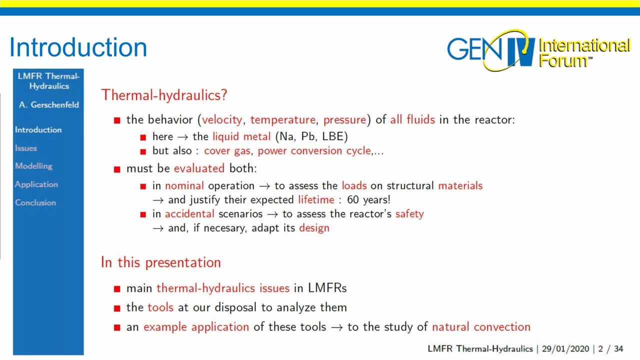 So what it deals with is what's the velocity in the fluid, what's the temperature and what is the pressure, And here, in our case, we're mainly going to be concerned with the liquid metal in our liquid metal fast reactor. So maybe we'll have either sodium lead or let's just go to eutectic. 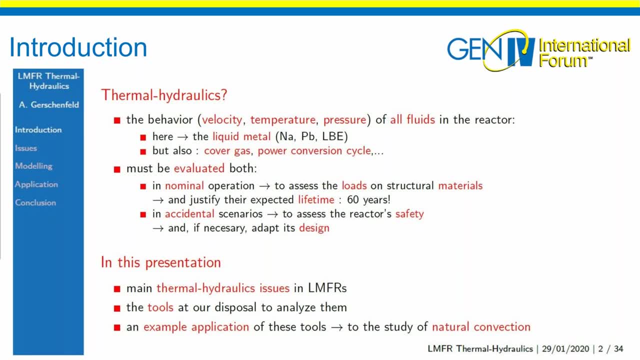 But also in the package we also need to cover gas in the reactor, for instance argon at the top of the primary circuit, or maybe the power conversion cycle which could use steam or nitrogen or another thing. And it covers also two very different types of calculations. 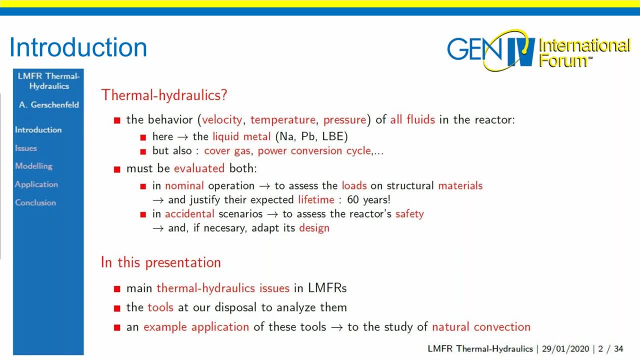 One is for the normal operating state of the reactor, So it's going to be a steady state in normal operation, And the goal in that case is going to assess the loads imposed by the fluid on the structural materials of the reactor. And the main issue with that will be that we will need to justify that these materials 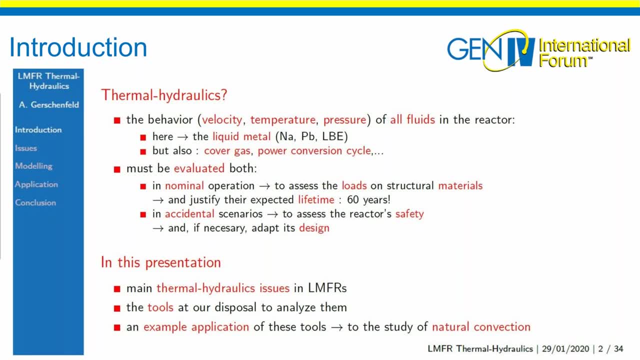 can last the expected lifetime of the reactor, So, for instance, 60 years for the structures. And also we need to deal with accidental scenarios, And in that case the goal will be a much shorter term, but it will be to assess a transient. 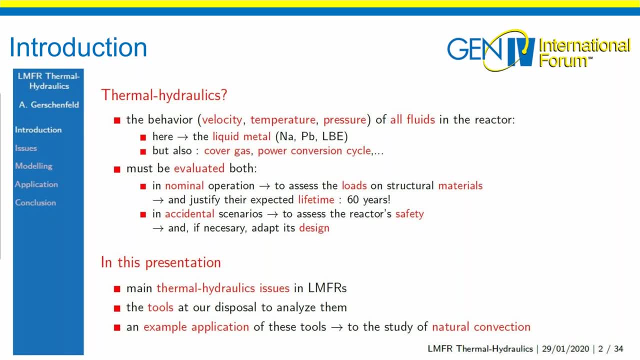 And we want to know if the reactor will be safe in, for instance, in the event of an unprotected loss of flow. And if we see that maybe we've got a problem or two, maybe we'll need to adapt the design of the reactor as well. 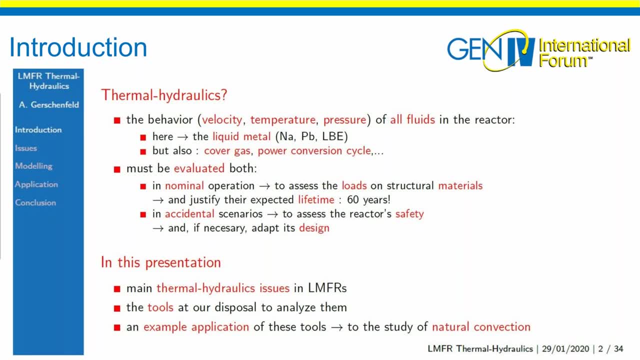 So what I'll be dealing with in this presentation is first a little overview of the main thermal hydraulics issues that we encounter in liquid metal fast reactors, And then I'll talk about the types of tools that we have at our disposal To analyze these issues. 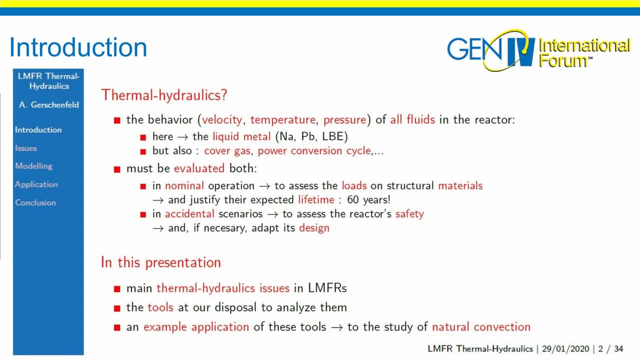 So the more mainly simulation tools and experiments. And then I'll give you an example of an example application of this to a practical case- And it's going to be something very fashionable since the Fukushima accident- which is the study of natural convection, passive decay, heat removal in a reactor. 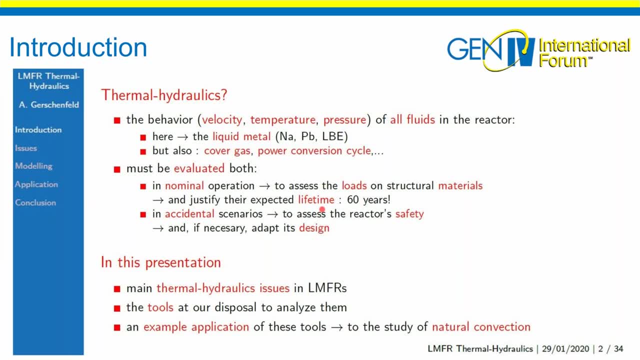 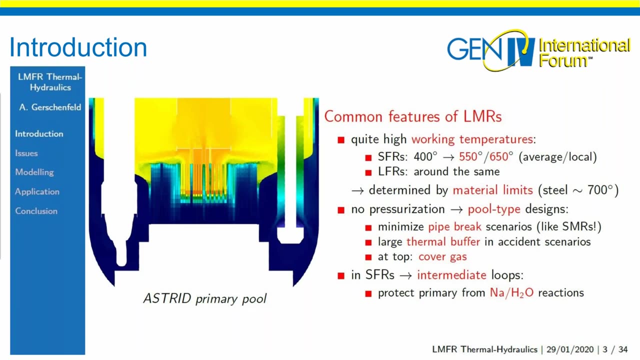 So, oh, I've got the problem again. Sorry, Sorry, Sorry, Sorry, Sorry again. Yeah, Thank you. So the main features of these liquid metal reactors, as I said, is that first, they've got high working temperatures. 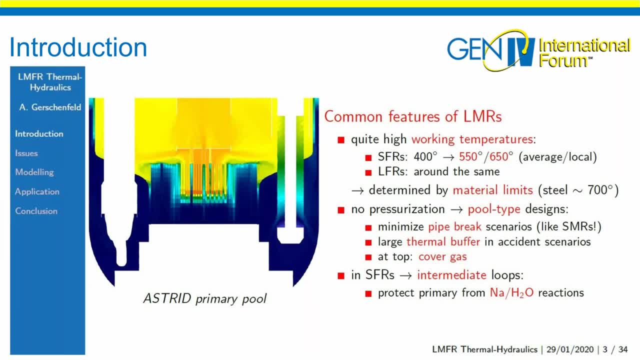 So in sodium fast reactors we usually have a cold temperature of around 400 Celsius And we go all the way to 500 Celsius, 150 for the average hot temperature and the local maximum temperature will be a bit higher even, And in lead-fast reactors they end up being around the same. And the main reason for this. 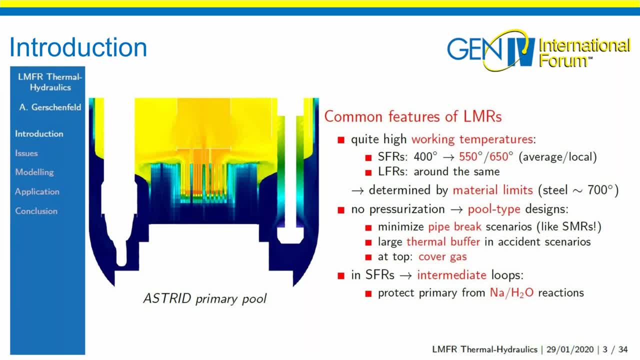 is that the main thing that limits temperature in a liquid metal reactor is related to the materials, Since it's somewhat hard to justify that common steels can resist long-term temperature, which long-term- for instance four years or maybe 60 years for the structures- at above 700 degrees. 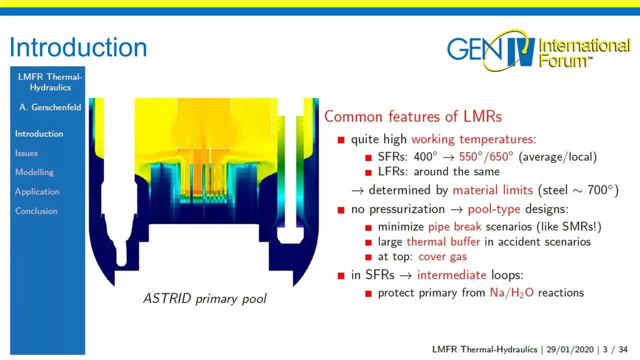 we usually limit ourselves to something like 650 degrees, And then, in order to reach these temperatures, we do not need any pressurization, And so we can rely on these pool-type designs. So we put all the primary circuit in one big pool, and this allows us to minimize. 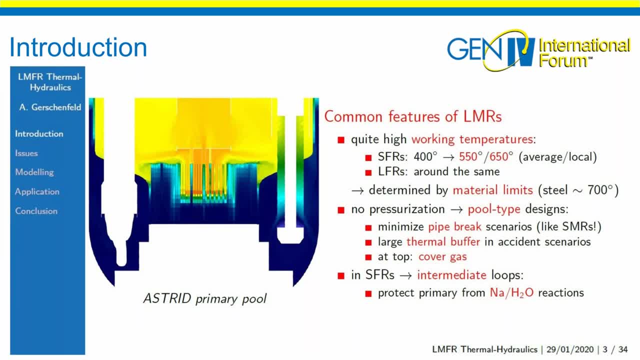 the consequences of a pipe break, And this is very useful for a sodium reactor where breaks and leaks could have chemical consequences, But it's useful in general to minimize the consequences on cold cooling. It also gives us a very large thermal buffer in case of an. 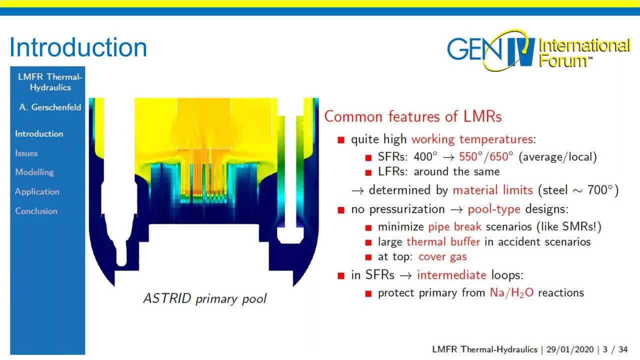 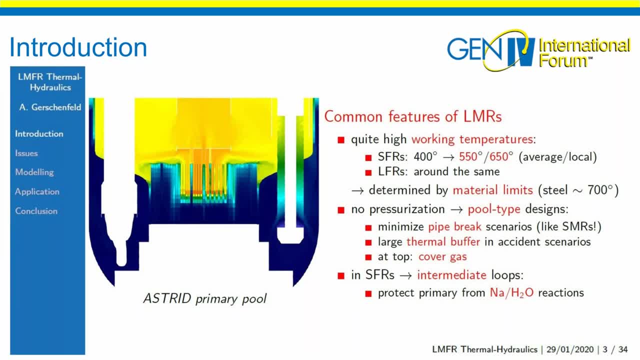 And then at the top of course, there will usually be a cold-cooling. So if we want a thermal expansion of the liquid, we can use a thermal gas to allow for thermal expansion of the liquid, And then so the fluid in this primary circuit will move the heat from. 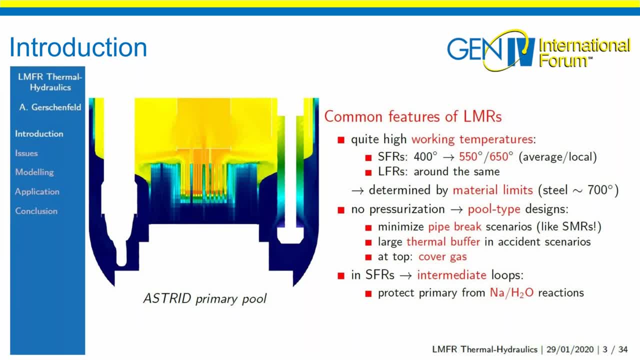 the core in the middle to the heat exchanger. you can see on the right And in sodium fast reactors. usually we have these exchangers go to intermediate loops that are also in sodium and this is to prevent a possible sodium water reaction in the exchanger. 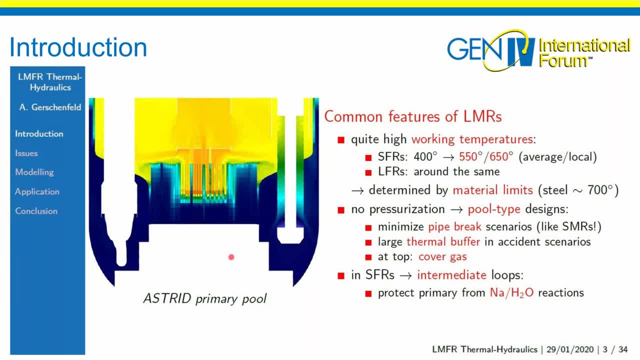 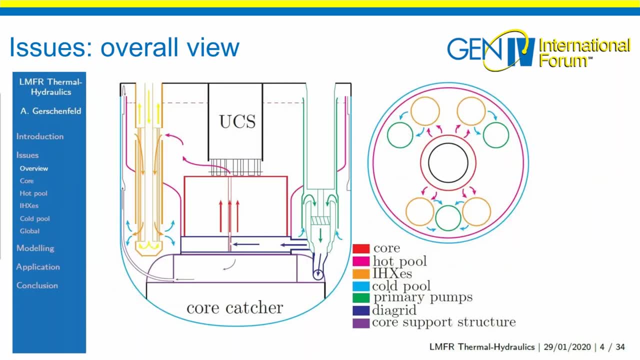 reactor, you could have a direct exchange to steam, for instance. So, moving to the next slide, Thank you. So this is the overall scheme of a common sodium-fast reactor. Sodium-fast reactor and lead-fast reactors look about the same. 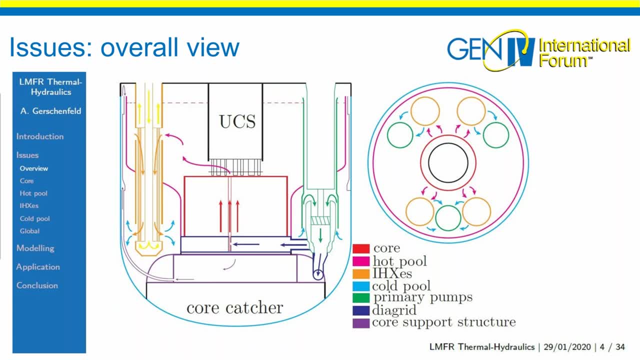 So you have the core in the middle with a number of sub-assemblies all in parallel. The liquid metal goes in forced convection from bottom to top And then it exits at the top in this purple hot pool. you can see, which is delimited by this inner vessel in purple. 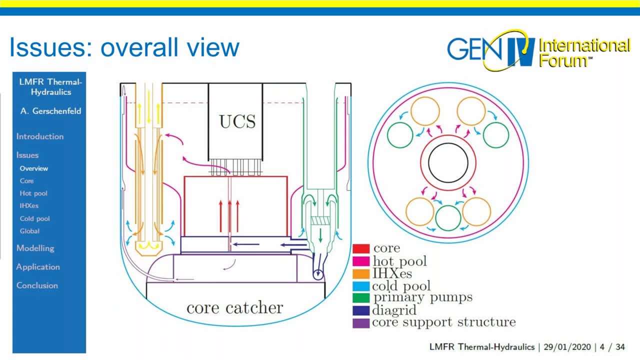 It goes straight into what we call an upper core structure, a structure that is above the core and that includes some instrumentation and maybe the drivelines of the control rods, for instance, And the hot pool goes, hits. this UCS goes to the outside radially and enters these intermediate. 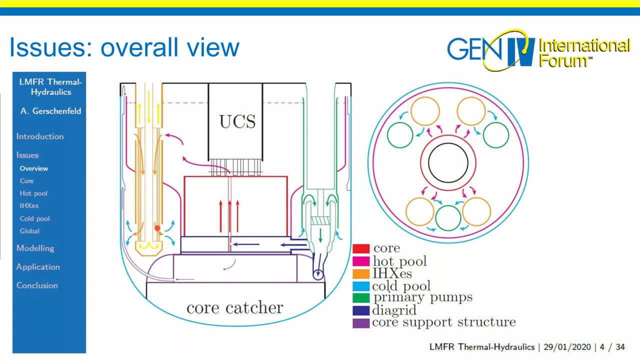 exchangers right there. From there it gives away its heat, ends up in this cold pool here at the cold temperature of the reactor, so 400 degrees from sodium, And then it ends up going around and moving all the way into these primary 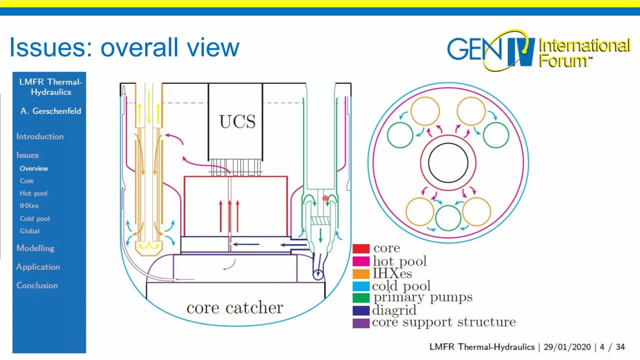 pumps here that are going to pick it up and pressurize it a bit In order to compensate for the pressure drop in the core. So usually the whole pool is at hydrostatic ambient pressure And right after the pump you may have something like three or four bars of added. 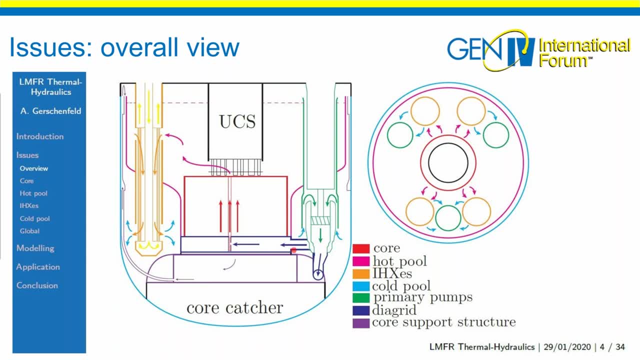 pressure to push the liquid into the core. And then you end up in this diagrid pressurized structure under the core and there are some holes at the bottom to allow the liquid to go back into the core and we do a complete turn like this: 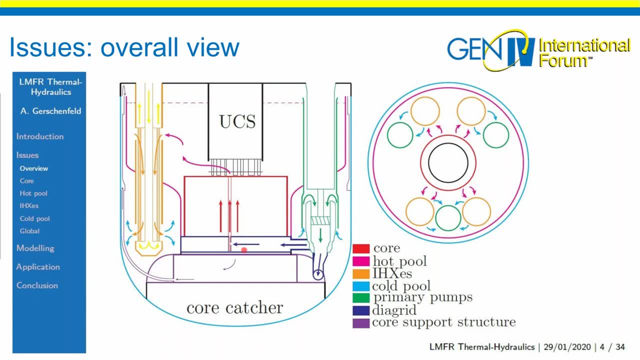 And then there is a little auxiliary system you can see at the bottom, which is something you need to prevent this main primary vessel on the outside here from heating up at the top. So at the top you have hot fluid in the hot pool here and it's beneficial to have. 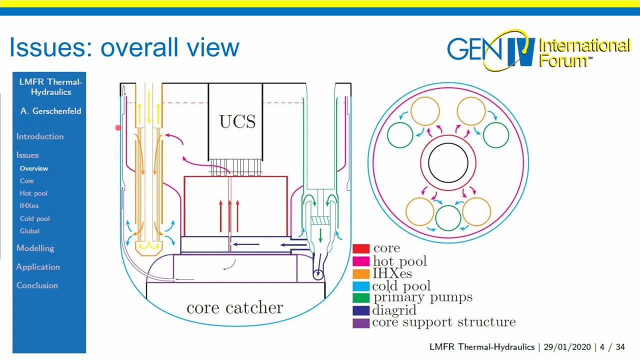 this main vessel here at the coldest temperature possible, And so what is usually done is that you pick up a little fluid that would otherwise go into the core And you inject it in an area of space all the way around the pool. 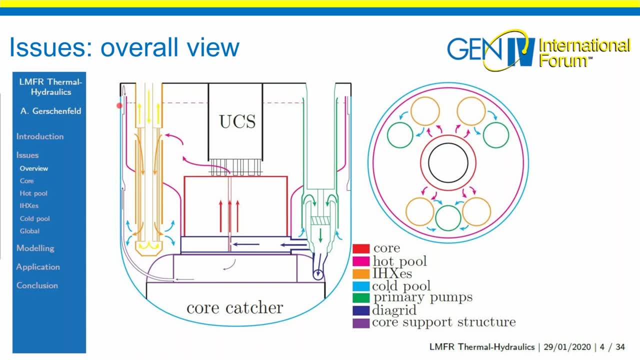 So this is going to cool it down at the cold temperature. So 400 in sodiums and maybe a little less for lead. It's going to go around and come back into the cold pool. So this is the vertical view. 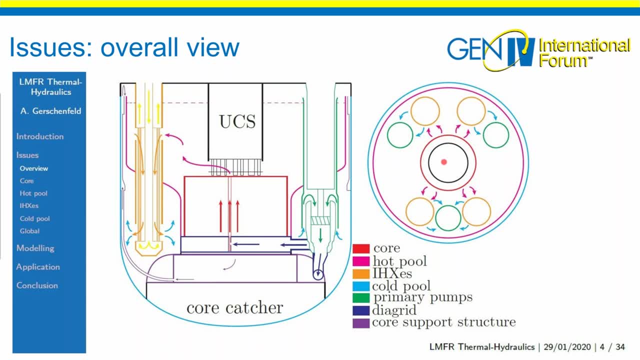 And then on the side view you can see that everything is usually distributed radially. You've got the core in the middle: liquid coming into the heat exchangers on the hot pool side, Coming down And then coming from the heat exchangers to the pumps on the cold side. 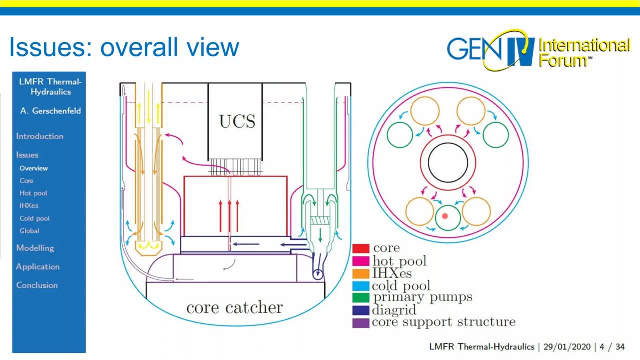 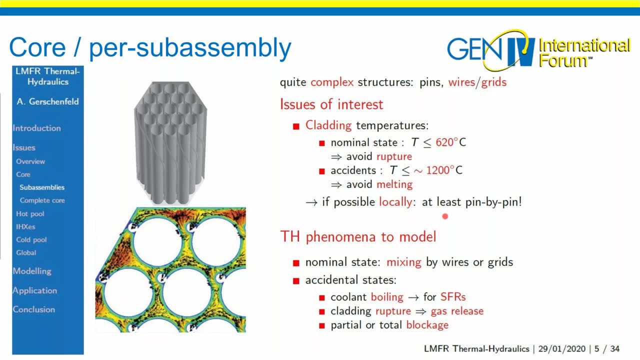 So next slide, please, Thank you. And so, from this overall view, let's begin our little, let's say- journey through each element in the reactor. So the first thing we encounter, starting from the The core, is the inside of the core sub-assemblies. 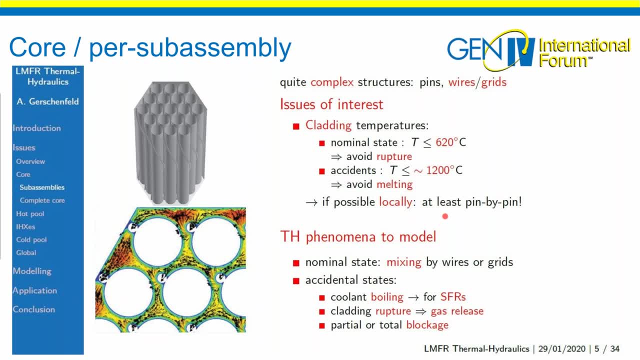 And actually the sub-assemblies in a liquid metal reactor are usually quite complicated, So you've got very tightly packed, pure pins like this, And this is because we want to minimize moderation or absorption by the coolant. And so, since they are packed so tightly, usually we use these wire spacers, right. 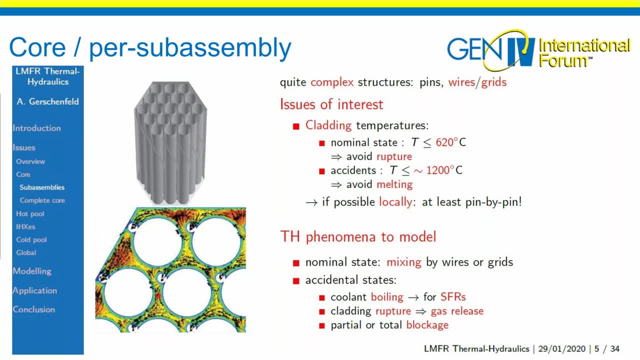 here. So this is common in almost all sodium-fast reactors and in around 50% of lead-fast reactors, And using this And using these wires means that there will be some non-trivial coolant mixing effects And they are going to be very important when we want to compute the nominal state of the 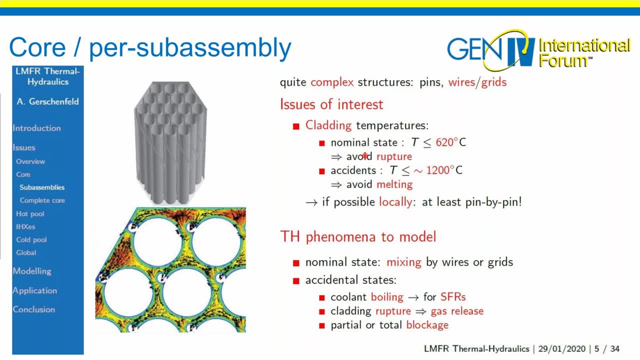 reactor. So usually material specialists from irradiated material studies will give us a goal on the maximum temperature of the fuel cladding And they will tell us that if we manage to stay below a given temperature, like 600, 650 degrees, then there will be no cladding rupture over the lifetime of the cladding. 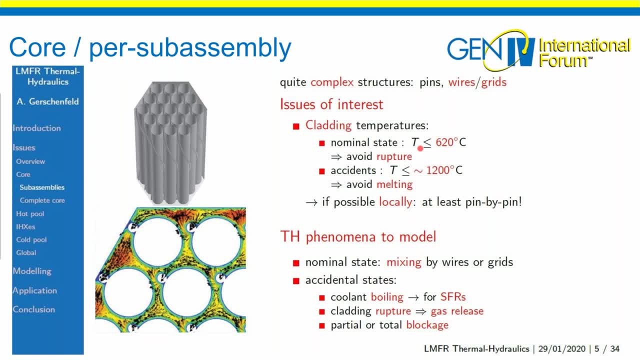 So this will be very important, Thank you. So we need to know the boiling time of the fuel, And so we need to do the friendly at EuroLeaks computation to guarantee this point, And then, during an accident, the goal will be much shorter-term and we need to check. 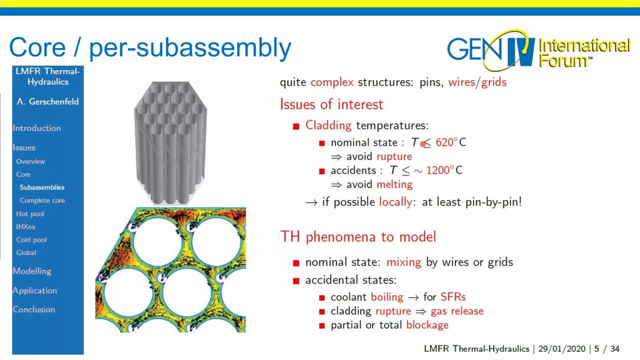 that the cladding will remain below its melting points and we will not have a transition to a severe accident scenario, for instance, where the core would be disrupted. And we need to know this at a local scale and at least we need to have it for each of. the pins in each sub-assembly in the core. So, as I've said before, and certainly a few years later and then, if we're going to take a look at the half-life in the back, we need to have a look at that as well. 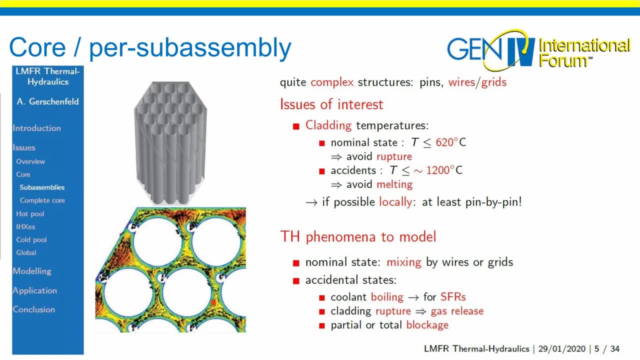 So these sanae will be used, which is to say they will actually work within a large, As I said, in the nominal state. the main issues in this thing are going to be taking into account these mixing effects by the wires or by the grease that you could have in a 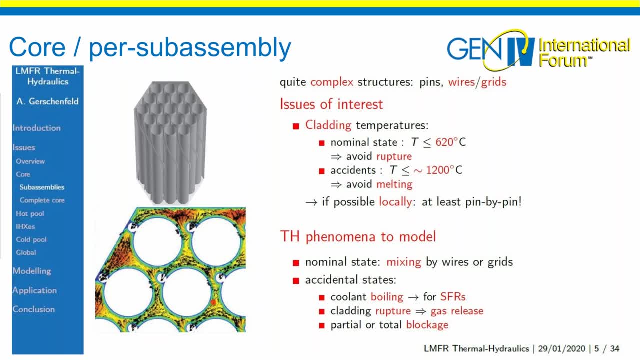 lead-fast reactor and then in accidental conditions. So in sodium-fast reactors, there is the possibility that the coolant will boil before the fuel melts, because the melting temperature is 1,200 degrees and the boiling temperature will be around 900, so you could have sodium boiling before the cladding breaks down. 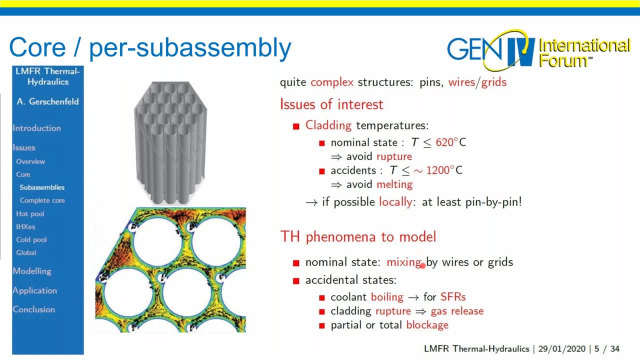 Of course, then you could have a cladding melting and possibly rupturing before and releasing fission gases, and a common problem both in sodium and lead-fast reactors is what could happen if you have a blockage inside the fuel assembly and, in this case, flow. 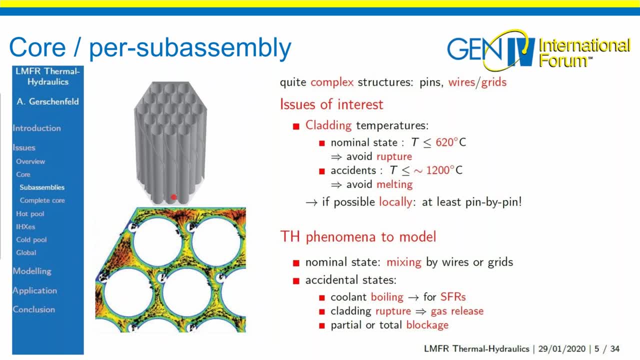 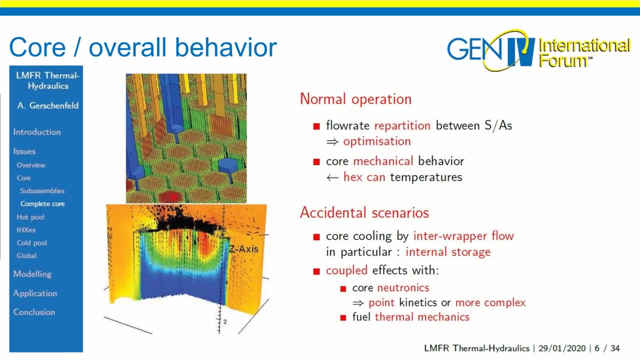 will be disturbed, cooling will be disturbed as well, and the local temperature will increase, and this requires thermo-hydraulic computation. So moving on, Moving to the overall core. so first looking at each sub-assembly separately and then to the big overall view. 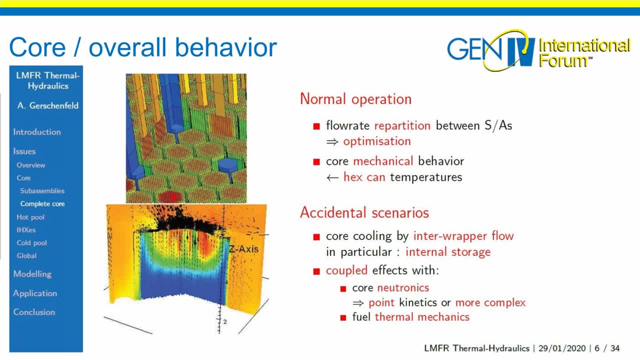 So, when you consider the core in its entirety, another thing that happens is that with these fast-reactor sub-assemblies- usually the sub-assemblies have hex cans around them. They are isolated from each other from an hydraulic point of view and you can choose. 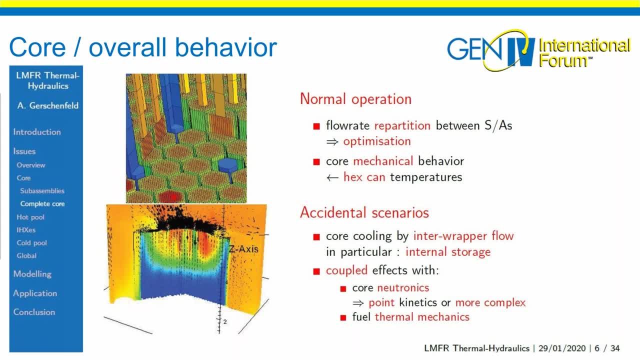 for each sub-assembly what the flow rate will be in normal operation. And normally in the core you would have a power distribution with more power in the center and less on the outside, And so if you want to have an optimal cooling of the core, it's beneficial to have more. 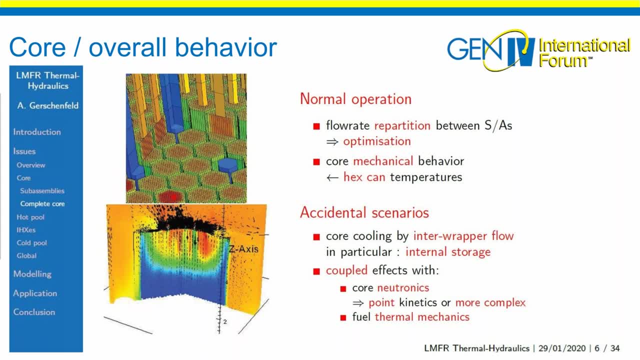 flow rate going into the middle than in the outside, and this is something that's done by allocating different flow zones in the core, and this is actually rather complex optimization problems. So how to allocate the overall flow between the sub-assemblies of the core is primarily. 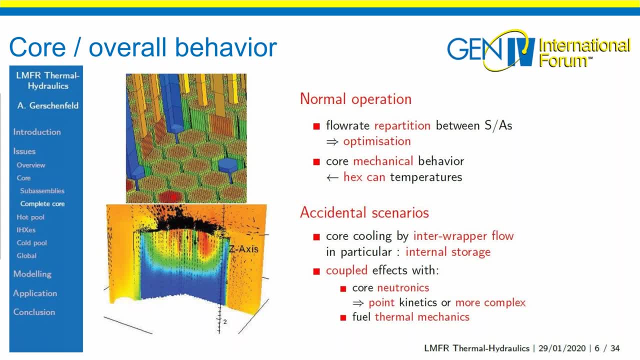 optimization problem. and then you've got all. you also got to account for the, the mechanical behavior of the core, and this will be many, many determined by the actual temperatures of the hexagonal cans around each of assembly. and so if you, if you want to know this one, you need to compute the thermal hydraulics. 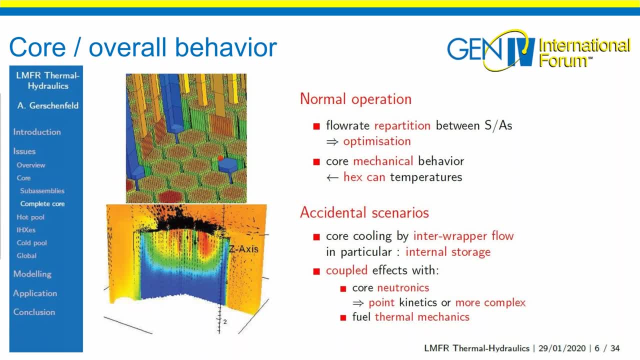 in the whole core. they choose the hex can temperature by accounting for conduction and then do a calculation of the mechanical equilibrium of the core. there's also some interesting problems in accidental scenarios. the first one is that on top of the flow inside each of assembly- because we've got this X can- 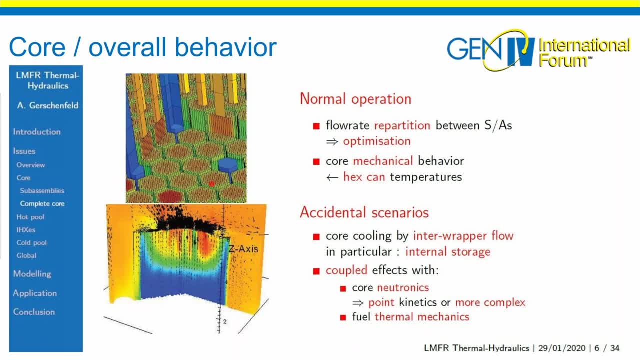 separating sub assemblies from each other, you can have cool. you can have cool on coming down between the sub assemblies and this is something called interwrapper flow and can have a very strong effect when you are in natural convection, decay, heat removal mode and, in particular, it can completely cool for 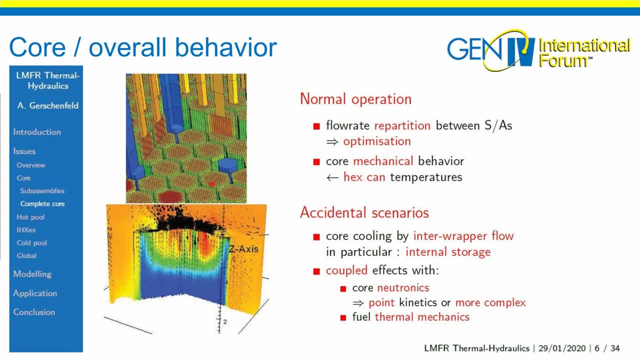 instance, if you are the, you can have a very strong effect when you are in natural convection, decay heat removal mode and in particular it can completely cool, for instance, if you are the subassemblies in internal storage so used of assemblies that you store on the. 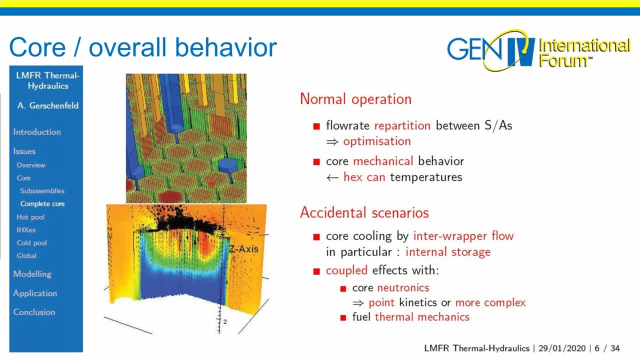 outside of the core at the end of a cycle and they can be completely cooled down by this mechanism. at this game you can also have copper defects, which for instance the neutronics of the core. so usually we use a thermal hydraulic specialist, we use a very, very simple point, kinetics models. but you could 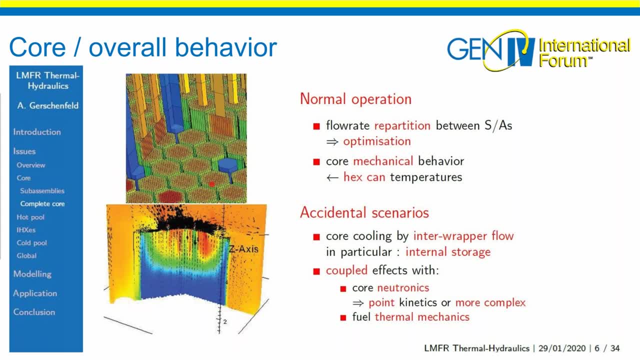 also use 3d kinetics, for instance. also related to this is the thermal mechanics of the fuel, because the thermal mechanics of the fuel is very, very. the thermal mechanics of the fuel is very, very, very. Now here you can can see one is because the Previously, the thermal mechanics of the fuel is very. this is because the 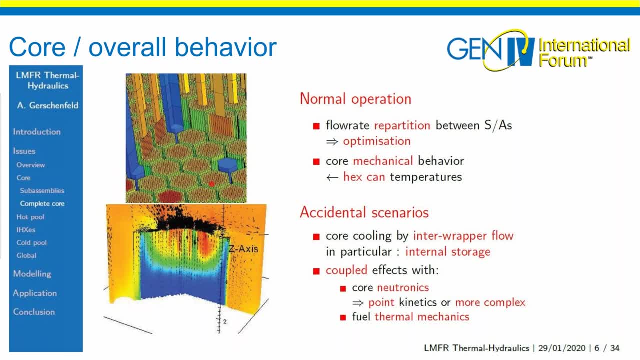 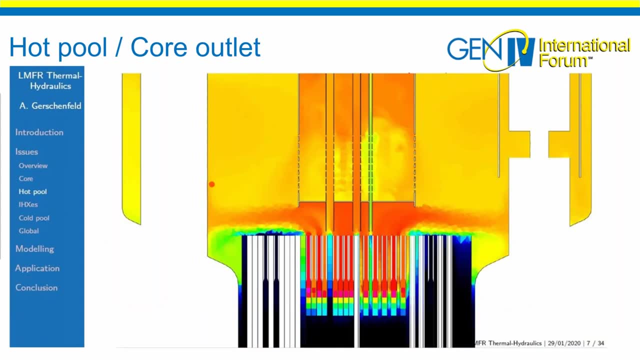 neutronics is strongly influenced by. neutronics is strongly influenced by Doppler effect, which depends until efter effect, which depends until temperature ficiente ohne temperature itself. 2 depends on the thermomechanical properties of isty. This level you can have a coupling with somatonix. 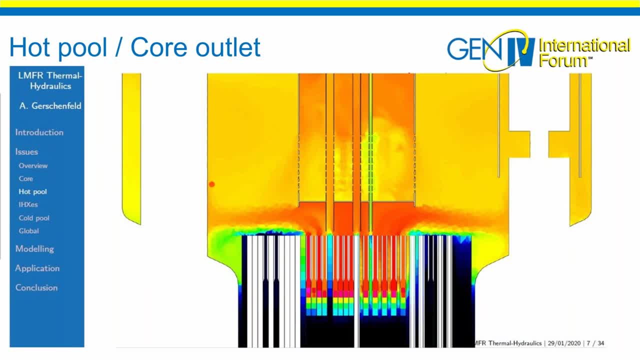 At this level you can have a coupling with Somany. moving out of the theory, encountre the hot pool, and here you can see another history of the hot pool of a liquid metal fast reactor. so you've got. this is the temperature, normal operation hitting this upper core structure and here you can see some control rod driveline. 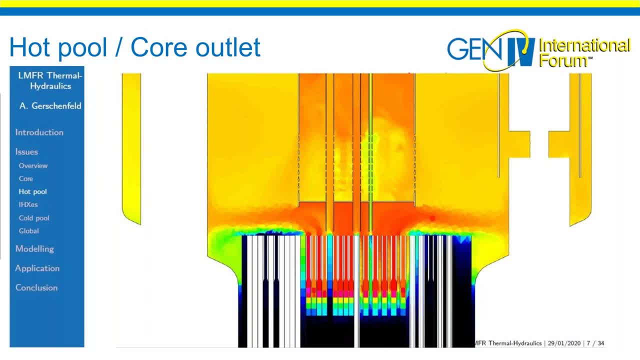 mechanisms at the top and you've got a jet of hot liquid coming out almost horizontally, hitting the first things it comes in contact with, so in this case the heat exchanger, and coming into these intermediate heat exchangers and then down, and so this is the temperature. 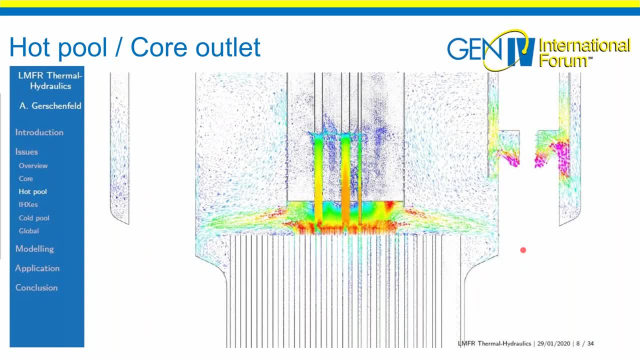 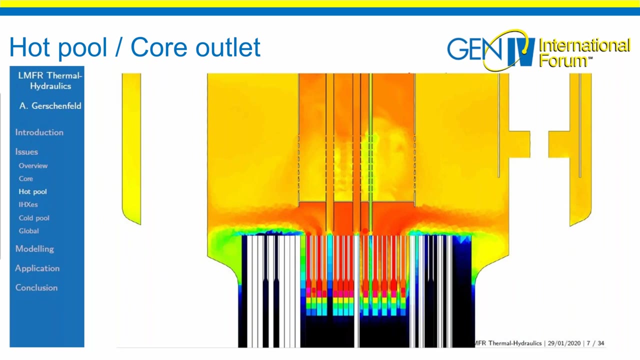 profile. and now you can see the velocity profile and you can see, similarly, this very strong jet coming out and at the top you've got this nice recirculation, recirculating flow patterns like this. coming back to the temperatures, you can see here that you have some temperature heterogeneities. 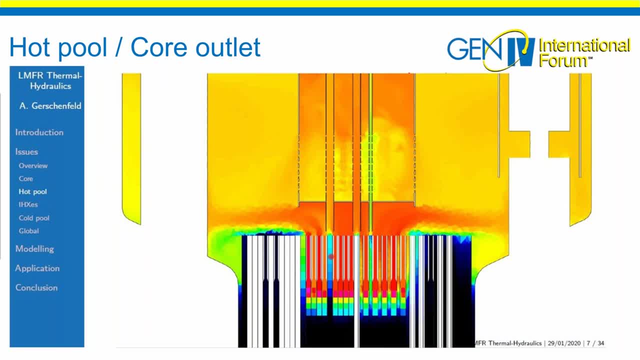 here because, for instance, this is the sub-assembly position for a control rod, for a control rod, and so there is no fuel in this, in this position, and so the temporary, there is also much less heating, and so you have a cold jet coming out in parallel to. 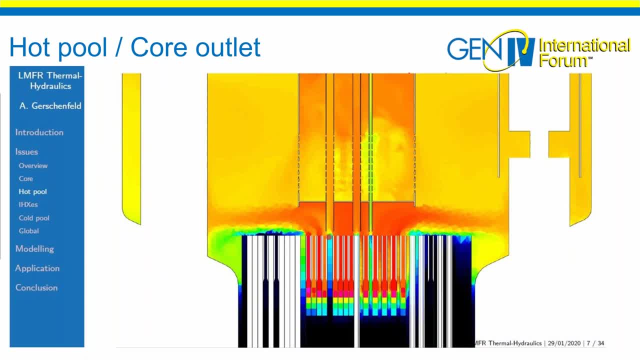 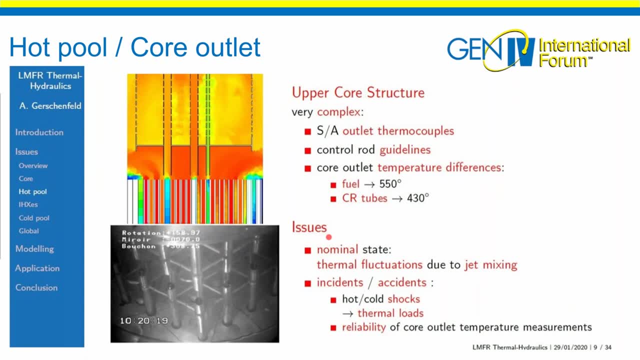 all the hot jets of liquid metal coming out of the sub-assemblies- and this is actually one of the first thermal hydraulics issues that we encounter coming out of the core. so the so talking about this upper core structure. so the first thing is that it's a 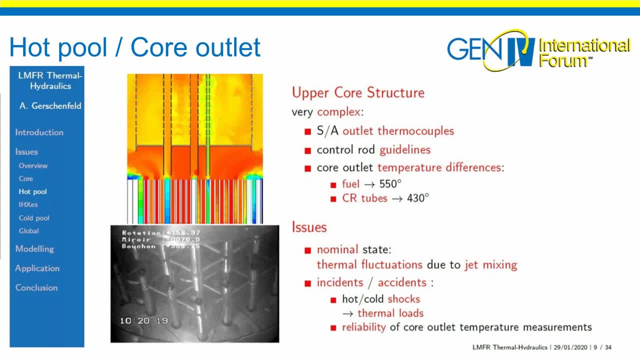 very complex piece. it's a very complex piece of equipment. you've got usually thermal couples coming down above the upper core structure and then you have a hot jet coming out of the sub-assemblies of each sub-assembly to monitor your temperatures. you've got these control rod drive lines here. 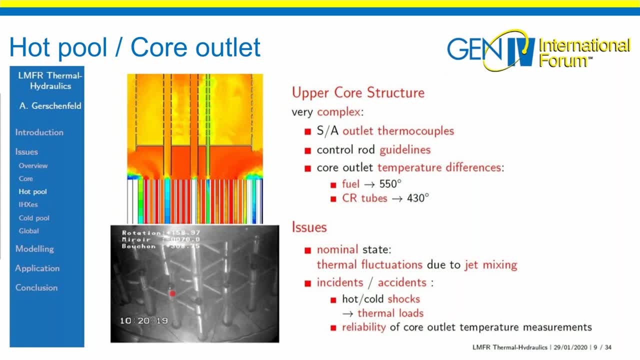 here you can see the the outlet thermocouples for the phoenix reactor and you've got this strong temperature difference between control rods and the narrowing fuel sub-assemblies. so in nominal state this is actually the source of the first main issue for the thermal hydraulics, if you have cold coming out here and hot liquid coming out right there. 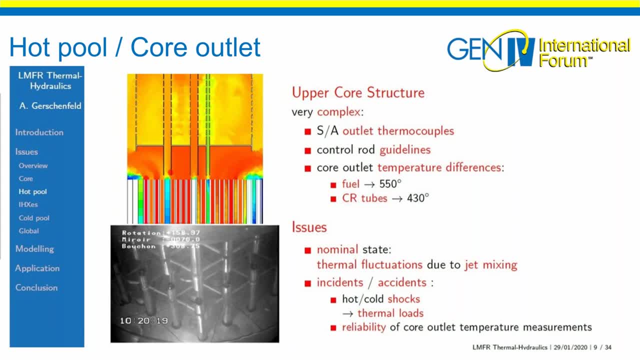 in practice you will have turbulent from a turbulent temperature fluctuations right at this position and this can be very damaging to the materials of this control rod ride. so this jet mixing effect has to be taken into account. and then, when you study incidents or accidents in the reactor, one of the first thing you could have is that if, for instance, you scram the reactor, 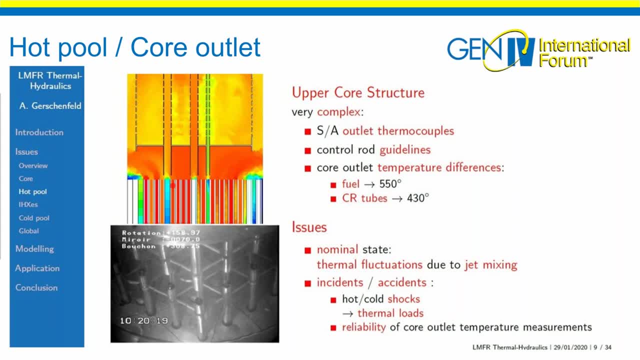 the power will go down very rapidly and you will have a cold shock on the UCS. If you have an unprotected transient, you will get a volt shock instead. Another issue you could have is that, because you have a jet coming out of the core and then sideways, it's not actually obvious that the measuring positions of 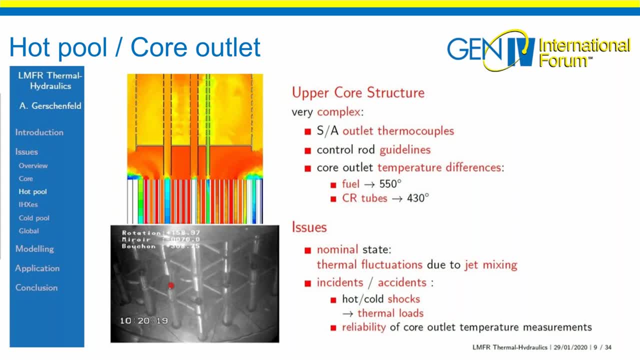 the thermocouples here will give you the actual outlet operator of the subassembly. below You will see some mix of the actual subassembly operator and its tables, And this needs to be assessed in order to interpret correctly the measurements from these thermocouples. 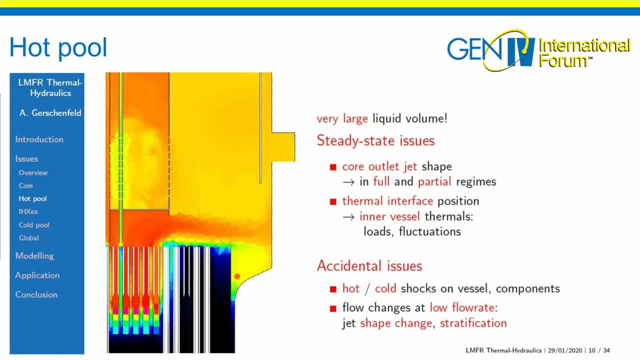 And then coming into the rest of the hot pool. So the hot pool is of course a very large volume of liquid metal. So in the Astrid reactor project in CEA, for instance, it was more than 1,000 cubic. 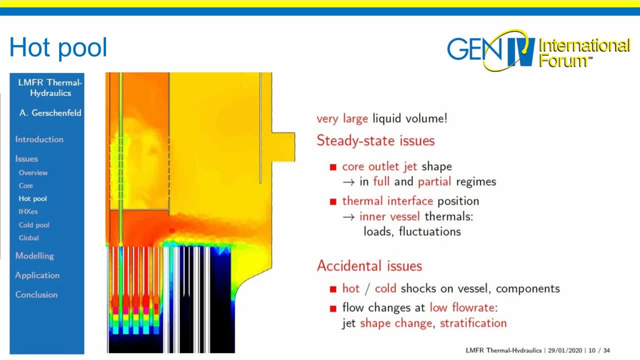 meters, And so for this, well, you've got some issues as well. So the first is: where is this outlet jet actually going? So in normal power operation with strong pump speed, it will usually go horizontally, like this, And on the other end, if you have a slow flow, so for instance, 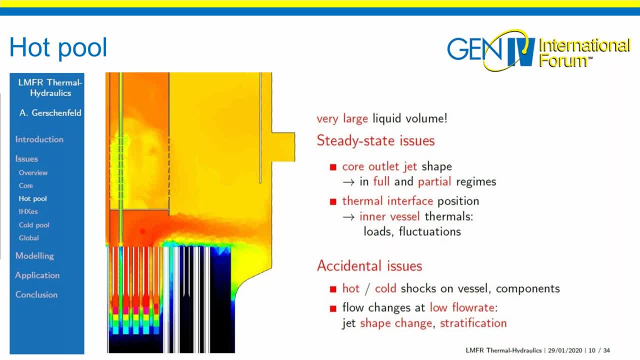 natural convection or something like this. instead of going radially, it's going to be moved by a very buoyancy forces, the fact that hot liquid is a bit lighter, and it's going to go up instead like this, And this can be an issue for. 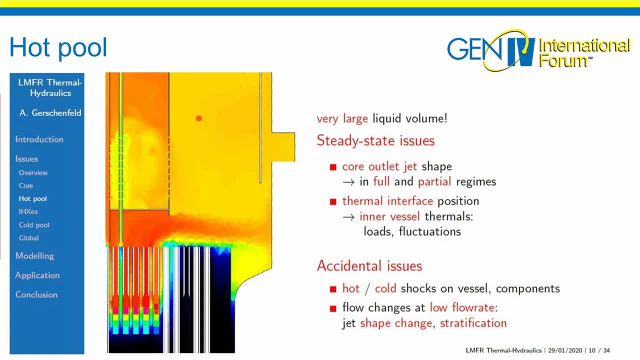 For reactors that want to do partial power regimes, for instance 50% power, 50% flow rate, all velocities divided by two, and this jet might not go in the same position as in normal operation. Another issue is the position of this thermal interface right here. 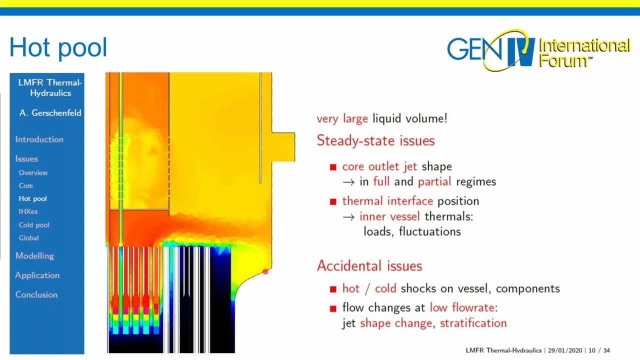 So this is an issue for the steel structure, the inner vessel that you get here. It's going to see If it sees thermal fluctuations or a very strong temperature gradient. it may have mechanical issues, And so this needs to be assessed from the thermal algorithm's point of view and checked. 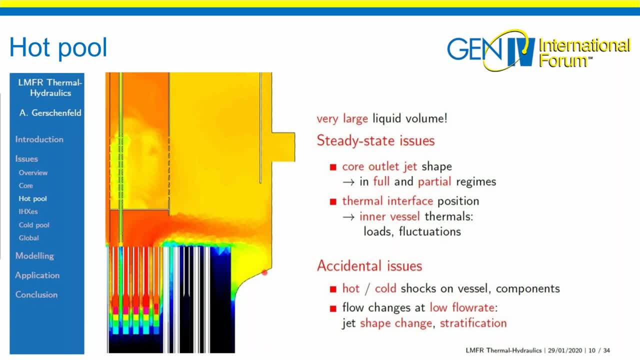 to ensure that the design will last for its 60-year lifetime. During accidental scenarios you can also have- Well, if you have hot shocks coming into here, then they will also be propagated all the way there, So you can get hot and cold shocks on the vessel and on the components in the vessel. 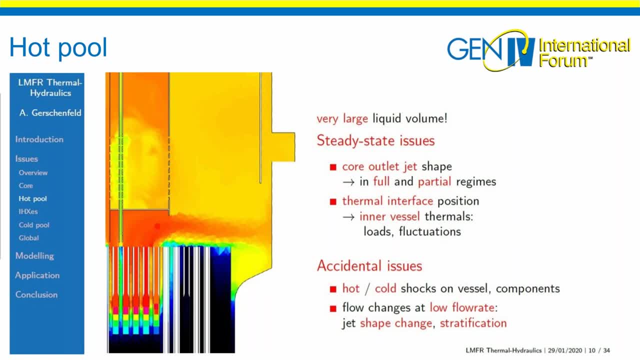 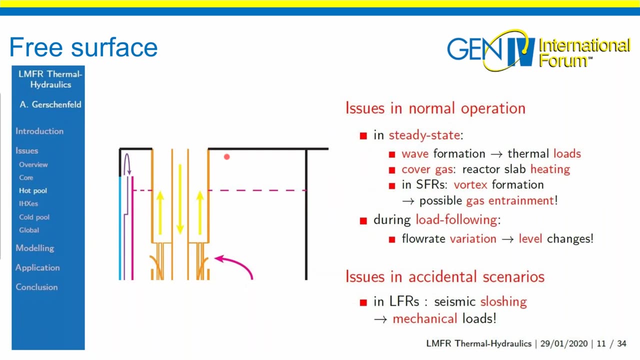 And then, During a transient, if the flow gets lower and lower, then this jet will have a very different, a very, a very different direction and stratification might also occur, and this is something we will see in more detail later. there are also some specific issues at the very 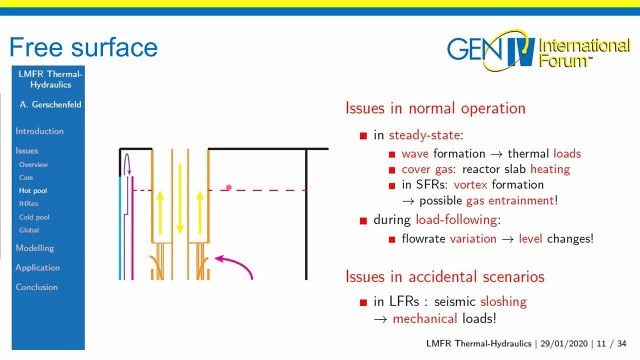 top of this pool. so, as i said before, in these big pull type reactors we need to have a cover gas with something like argon at the top in order to absorb the volume changes of the liquid below, with temperature, for instance. and if, if we have a free surface like this, well, one thing you could. 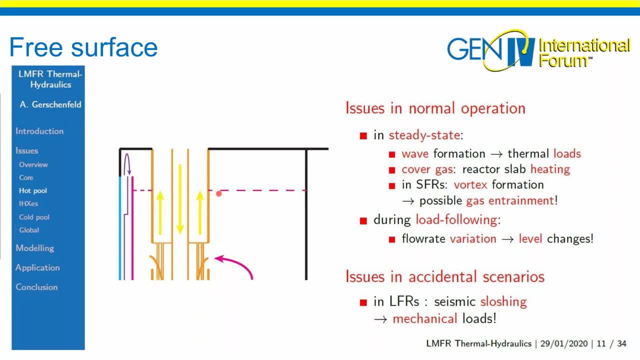 get is some wave patterns right here, some oscillation of the free surface, and this, of course, can cause thermal fluctuation on the structures at the outside and maybe from my damage. so we need to check for waves. another thing we we need to check for is the thermal 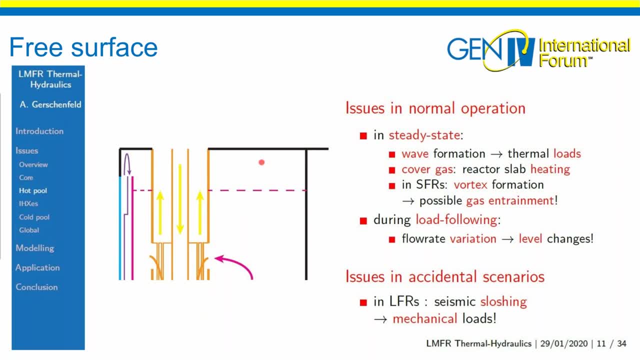 constant between the liquid metal and the reactor slab at the top, because this this will give you the amount of cooling you need to add to the slab in order to keep it at the temperature you want in normal operation. another thing that can happen- and this is mainly a problem for sodium paste reactor- is 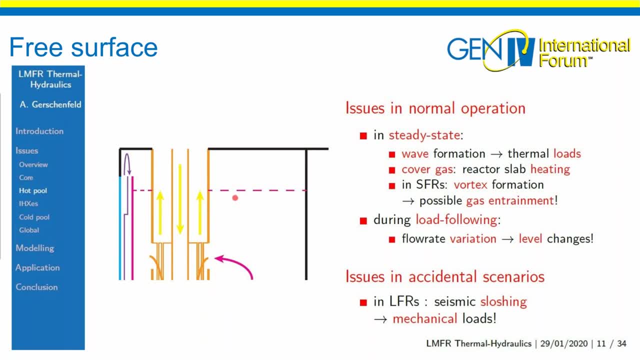 that if the liquid velocity is high in this region, then it's possible that vortices could form, like in a sink in your bathtub, for instance, and this can lead to vortices going down into the hot pool and possibly entraining some bubbles of gas into the complete primary circuit. and this is 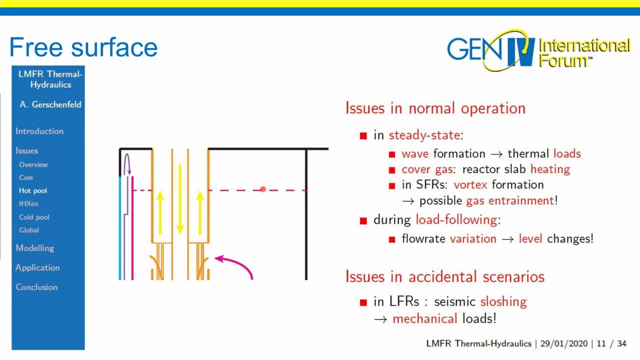 something that could have consequences later. if you have a load following reactor. usually when you change the power- the power of the of the reactor and the flow rate at the same time, this free surface will change its level and this this can lead to thermal stresses on the vessel right here and finally in with. here we've got a in. 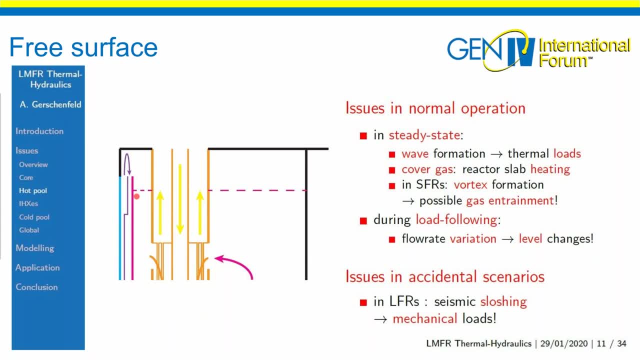 an accidental scenario where you can have consequences in that fast reactor. so if you have, for instance, an earthquake, then the earthquake can cause sloshing in this pool and you, so you, you will again have waves. and if you have a lead fast reactor, lead has a 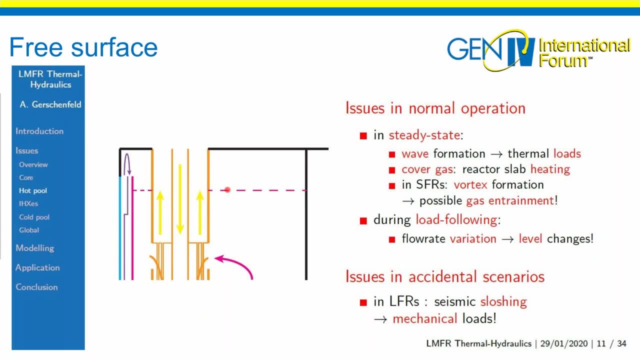 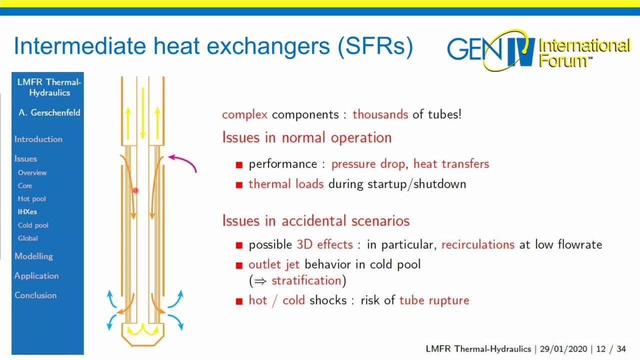 very high density right around 10, and so it can lead to mechanical constraints of on all the structures right here, and this is this is something that is not too important in sodium fast reactors but becomes more important if you apply. so, moving into the heat exchangers, so the heat exchangers are actually some. 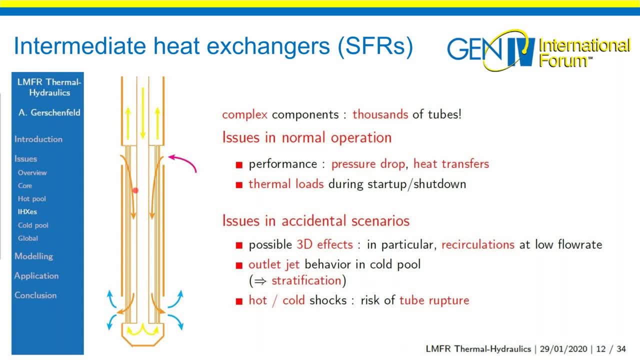 very complex, complex pieces of machine, of machinery. they've got thousands of tubes. usually they are straight tubes like this and the first thing that needs to be assessed in normal operation is: what is the actual performance of this heat exchanger? so what is the pressure drop on both the primary side going? 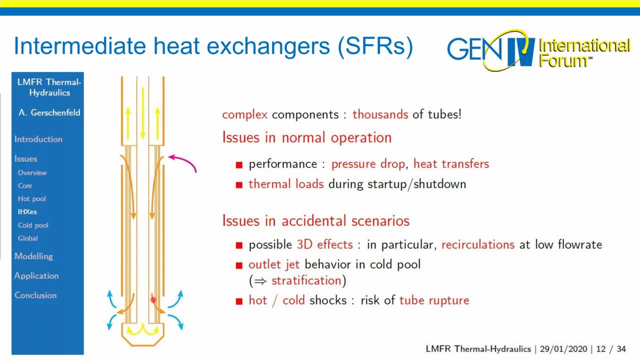 around the tubes and the secondary side going inside the little tubes. so what's the pressure drop? what? what is the actual heat transfers and also what thermal loads are going to be experienced on the tubes during a normal start-up and shutdown. and this actually was the source of many problems on the 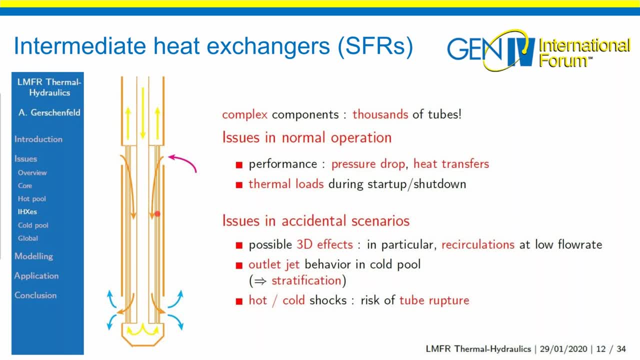 Phoenix reactor in France. because of that differentiate from ideation of the tubes and the rest of the exchanger. during normal, during move from stop state. with normal operation these exchangers are to be replaced many times and then in accidental scenarios you can also have additional things. so one is that at very low flow rate you 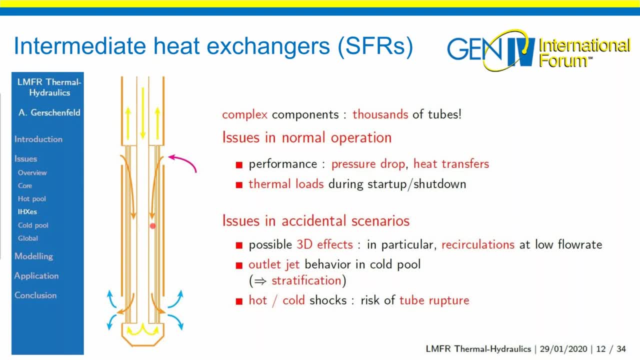 can actually have some complicated flow patterns inside the exchanger, so, for instance, a recirculation between the inside and the outside. the shape of the jet coming out of the exchanger is also a particular interest, and this is this is something we see just later in the cold pool. and finally, 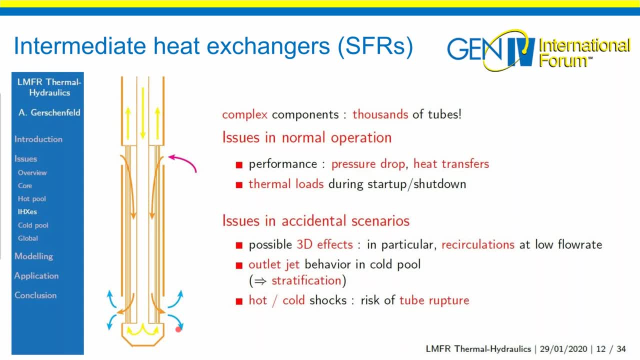 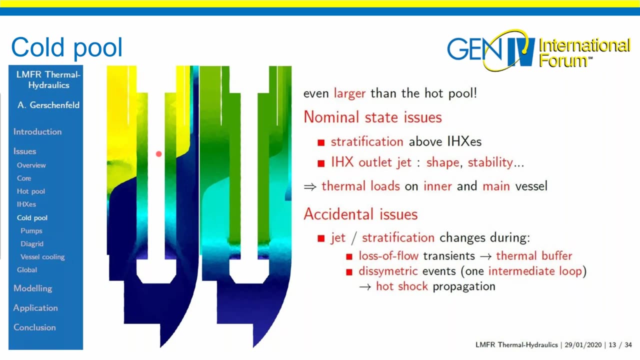 if you have hot and cold shocks, for instance, if you're screaming the reactor or doing an unprotected transian, then you could have some tear repair problems, so going into the cold pool. so usually the cold pool will be even larger than the hot pool and it's going to be a very different process from the 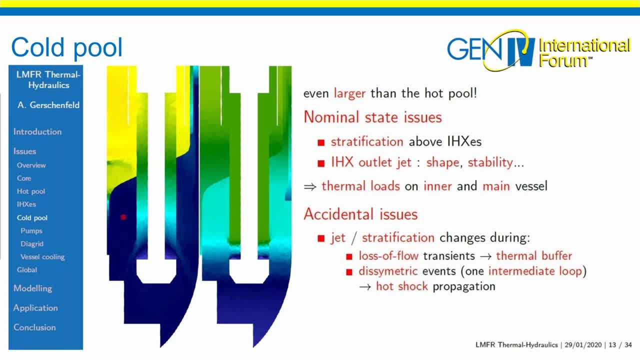 to have some very different temperature profiles in normal operation and in, for instance, low flow natural convection. in normal operation the cold pool will usually be very homogeneous and completely at the cold temperature, with some profiles at the top where you have the vessel cooling system on the outside and coming back down and you are, you will have this outlet jet. 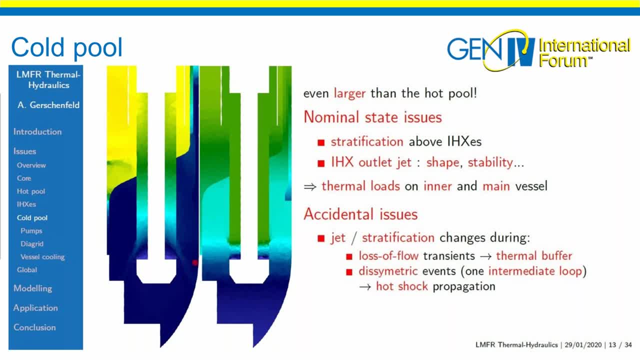 from the heat exchangers right here and so in normal operation. what we want to know will be the shape of this jet, for instance. it could, you could have some. so, as you can see, this jet will usually not be at a homogeneous temperature. there is a little hotter part at the outside. 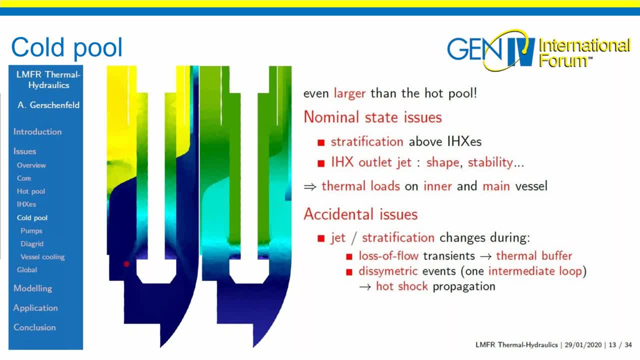 and the colder part at the inside, and this little temperature extension into the cold pool can actually hit some structures right in front of it and potentially cause formal damage. so we need to know where this heat exchanger water jet is going, and one of one thing that 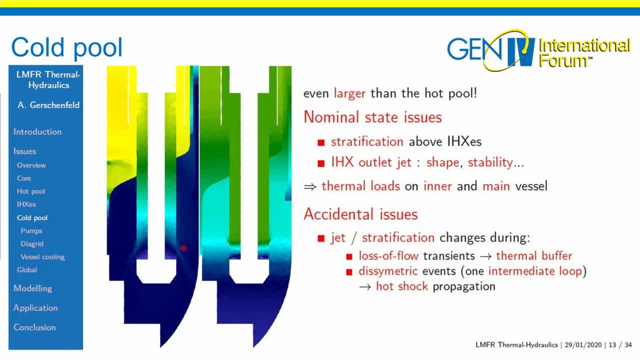 can happen is that if the flow gets a lot lower, then this jet will go straight up like this and contribute to stratification in the cold pool and maybe thermal loads on some other structures, and so that's actually the what we need to compute for in case of an accident. so where? 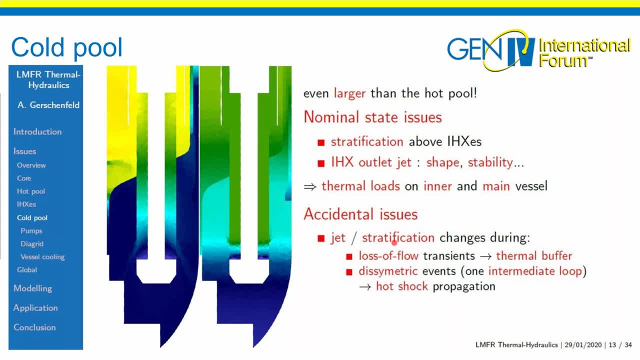 the jet is going and what thermal certification will be. and this can be important both during loss of flow transients, so when we lose the pumps. so this is what is actually pictured on this right figure, and another thing of interest is what we call this symmetric event, for instance. 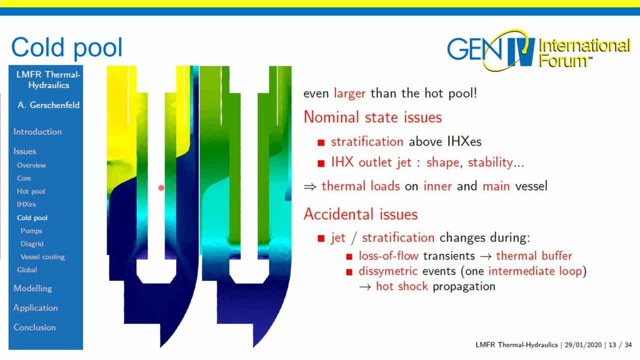 if the reactor is operating and then one of the intermediate loops trip, then cooling will be removed from this exchanger and suddenly you will have hot liquid coming up, coming down on one side of the of the cold pool only. so you will have a hot shock in the cold pool. 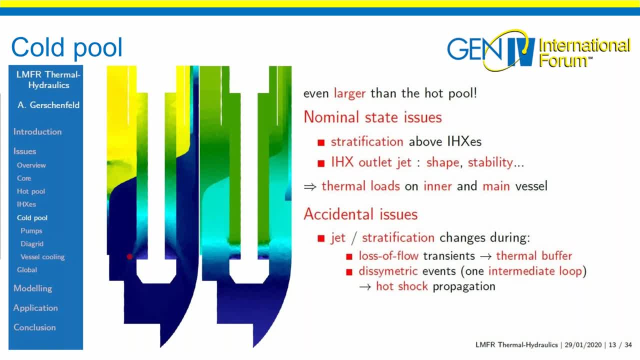 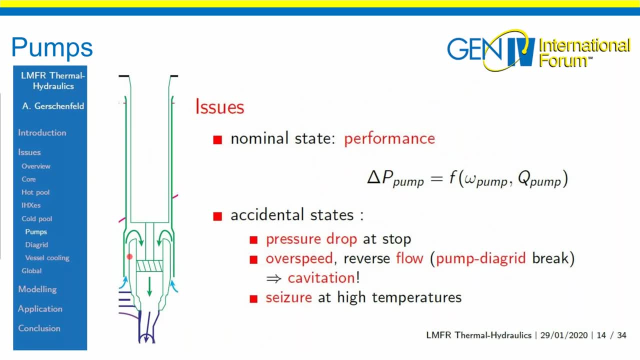 on one side and then it's going to propagate in the cold pool and this can be actually quite interesting to model. so then, coming out of the cold pool, you've got the pumps. so in the pumps the main issue in nominal state. so they're going to pick up liquid from the cold pool and inject it back into the core. 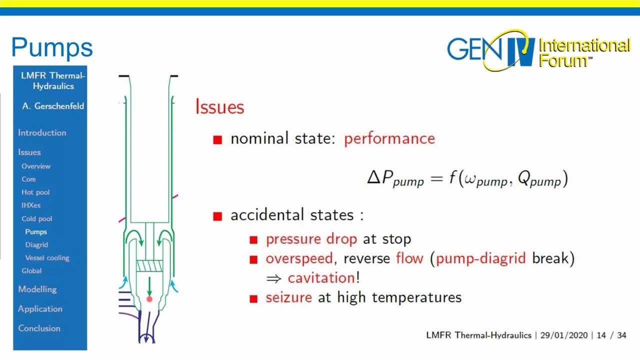 and the main issue is going to be their performance in normal operation. so so their full characteristic. so this is the. so this is the data p: the pressure difference provided by the pump for a given rotation speed and a given flow rate of liquid metal. and in normal operation we will. 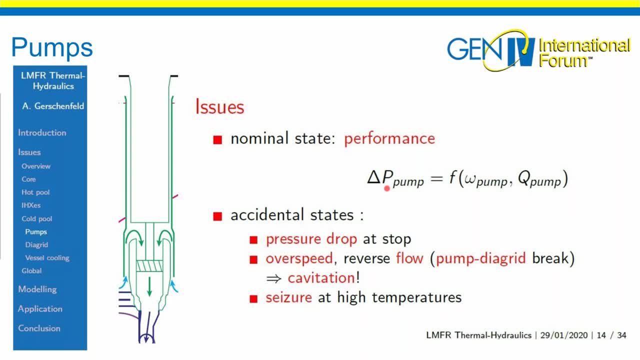 only be interested in the normal operating point of the path, but then for accidental scenarios, we'll be interested in a lot of other values of this function. so, for instance, if we are modeling loss of flow scenarios, then the pumps will be stopped and we will need to know the pressure. 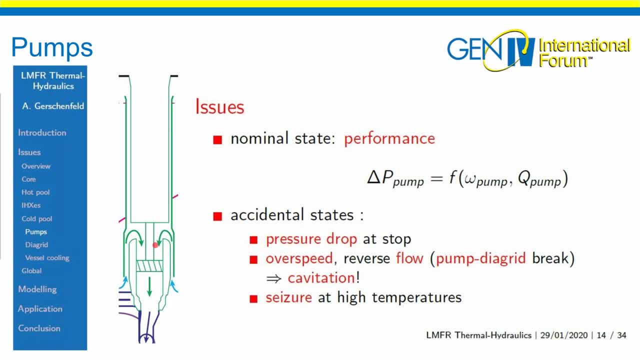 drop of the pumps when it is stopped. if you've got an event where one of these pipes at the outlet of the pump and before the diagram breaks down, then the pressure in the diagram will drop and the other pump, the other pumps, may go into over speed and this can lead to cavitation inside the 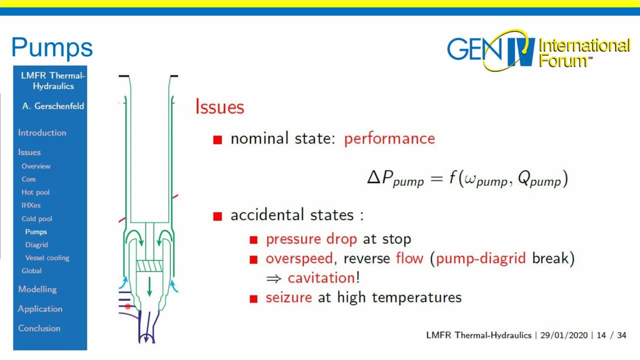 path in. in some cases, for instance, if one of the pumps stop but not the user, you may have reverse flow in one of the pumps and some other complicated problems. another thing we will not be interested in is the definition of the pressure drop in the pump. 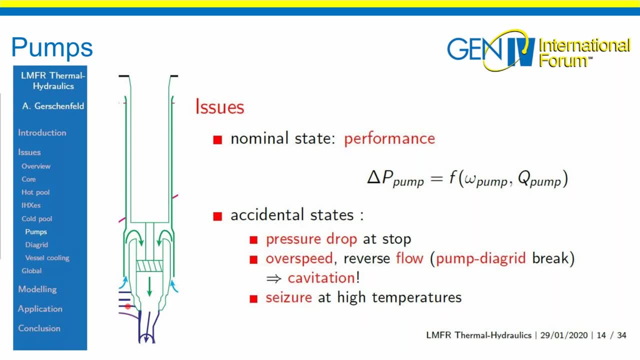 we have to use more complicated room to account for this negative flow in one of the pumps and some other complicated problems can happen. if you have a trend, if you have a transient like loss of heat, a loss of heat sink, then you may have the pumps operating but the temperature in the whole, in the whole pool, will. 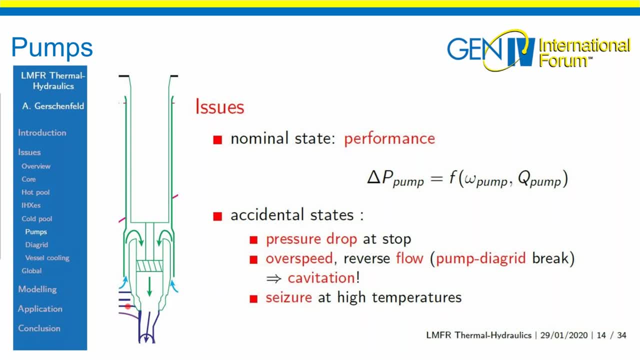 go up little by little and at some point the temperature may be so high that the thermal dilation of this rotating part may make it contact the outside. and then you will have scissor of the pump at high temperatures and you will go into a loss of flow scenario on top, on top of your loss. 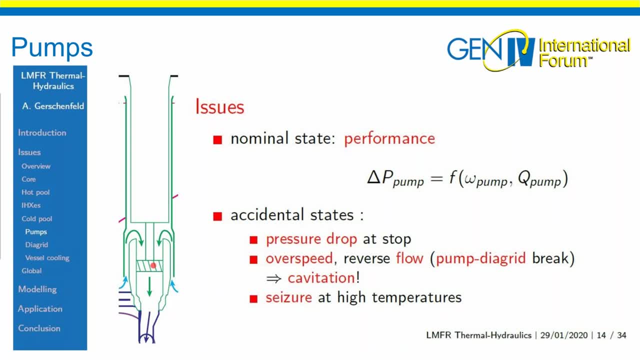 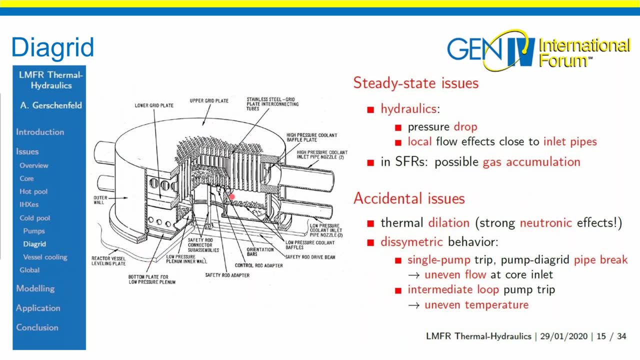 of heat, so this will. this is also something that needs to be watched out for. so then, coming out of the pumps, we've got the diagram, and this here is- this is actually a picture of the ebr2 diagram on the reactor on the same name: in, in, in, in, in and so the. so there are two things that we need. 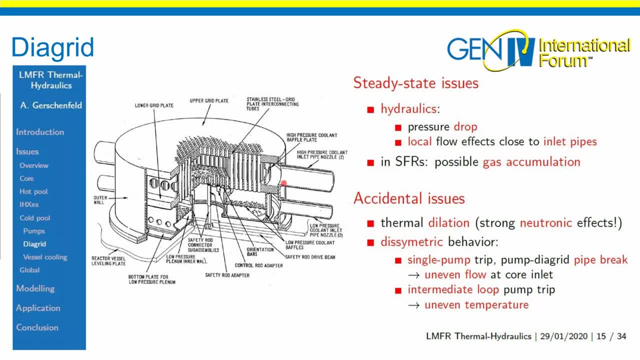 we need to model in this diagram is: first: it's actually a quite complicated structure, so you've got lots of tubes going around because they are going into the sub-assemblies and so on, and so the pressure drop of this component is actually not obvious. you can also have some local flow effects, for instance at the parts of 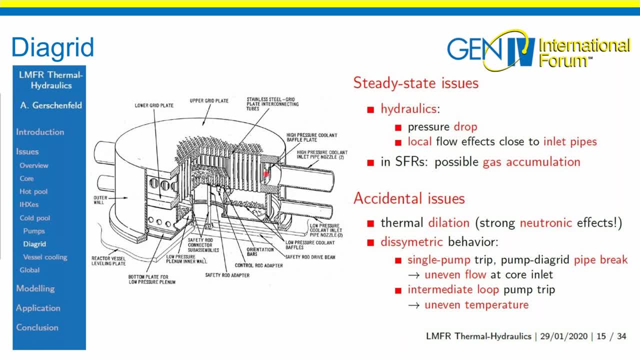 the diagram that are closest to the inlet pipes, for instance. here the flow will not be homogeneous, and so typically this is something that needs to be computed to know if you may not have what you expect in the sub-assemblies that are closest to these inlet parts. in sodium fast reactor we 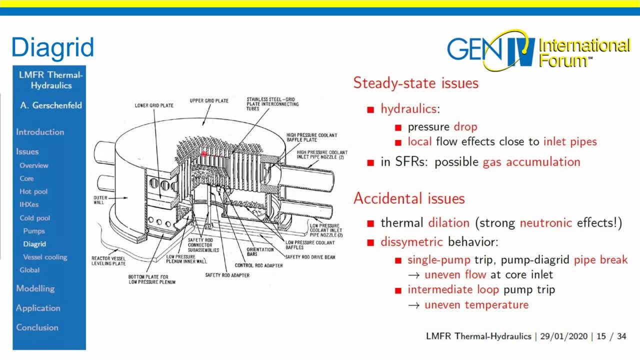 have the potential for gas accumulation in this diagram to watch out for, and this is something i'll elaborate a bit on later. and then we've got the accidental issues. so the first thing is in: in all liquid metal reactors when you have an unprotected accident, the delay, the firmware deletion of the diagram is actually the source of one of the strongest. 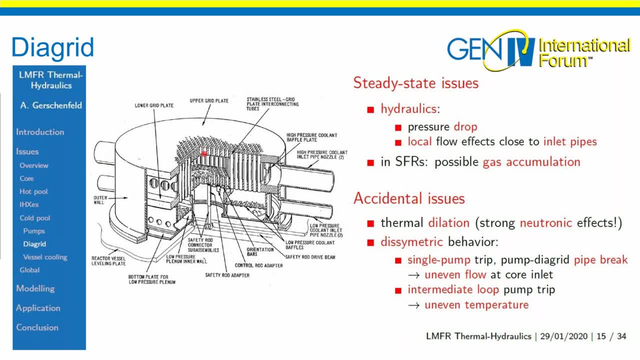 neutron feedbacks the reactor. if the diagram heats up- it's up- then all the sub-assemblies will be drawn apart, the complete core will dilate and the neutron reaction will will slow down more and more. so this is something that is actually very important when you want to model an unprotected 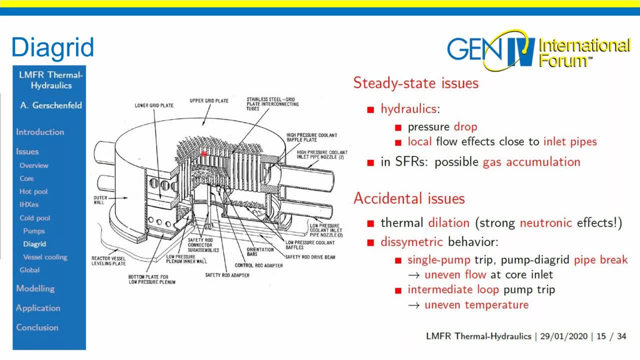 transient. another thing of importance is for all these dissymmetric transient, so for instance, trip of a single pump or the breakdown of a pipe like this, then you will have usually uneven flow at the core inlet. if this pipe breaks down and the lipom contributing in this one, then the sub-assemblies of this on this side will. 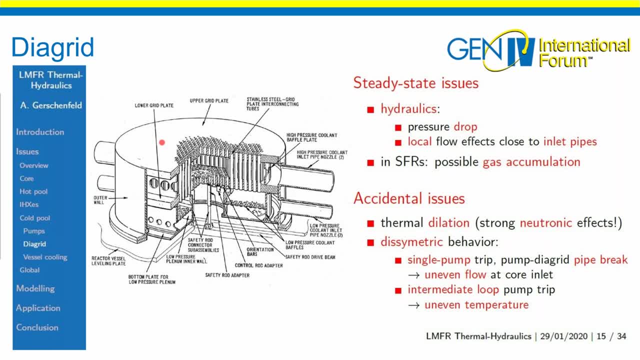 have more flow rates compared to the average, and this is something that can be important to model. same thing for these intermediate loop transients. so if you have one of the heat exchangers losing its heat removal power, then hot liquid will come out into one of the pipes before the other and 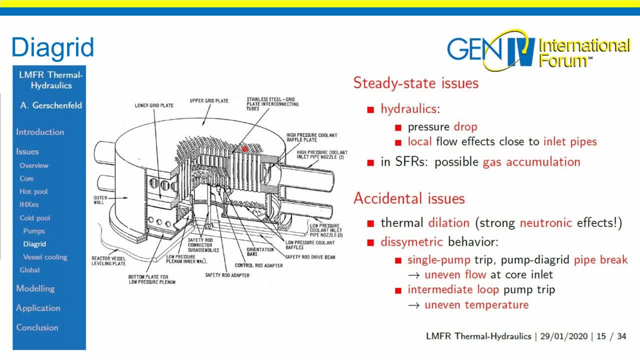 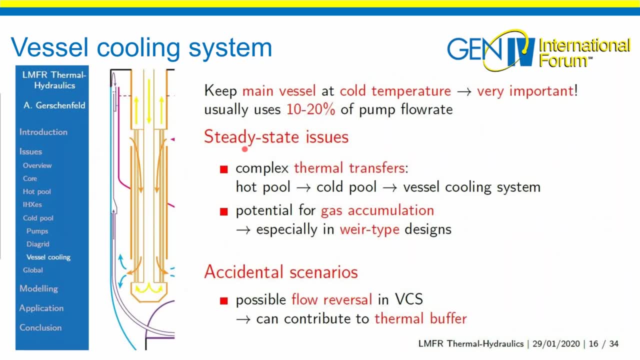 one part of the core will receive hotter liquid before the other, and this is this is also the same thing that you may need to model, and so, finally, the only thing we we still need to look at is this little vessel cooling system here. so this is sodium that you pick up. 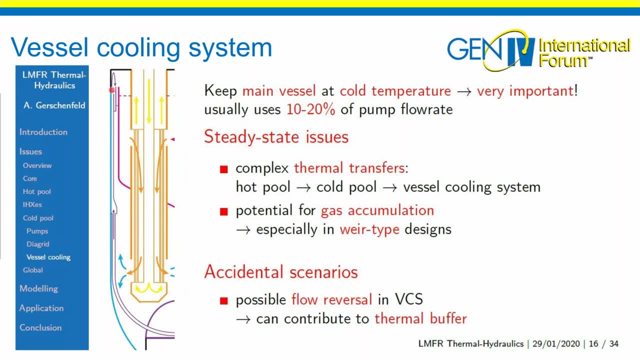 from below the core and you inject on the outside of the main vessel to cool it down. it's not so little actually. usually it's 10 to 20 percent of the flow rate provided by the pots. and so for this one, well, what we need to model is the actual thermal transfer from this. 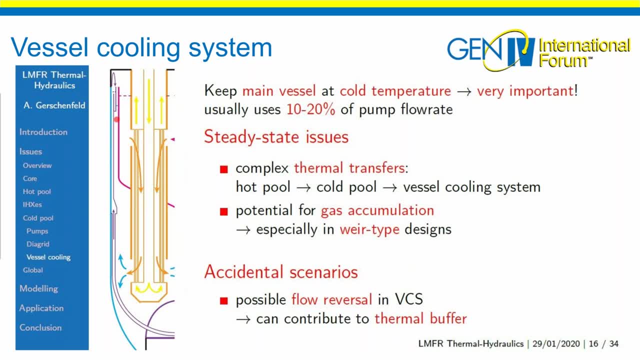 liquid to this liquid in the cold pool, which may be a bit colder to the liquid from the vessel cooling system. and so we need we need to model it in order to know if our vessel cooling system has the right uh, at the right size. and then if you use a system here where you have, where you 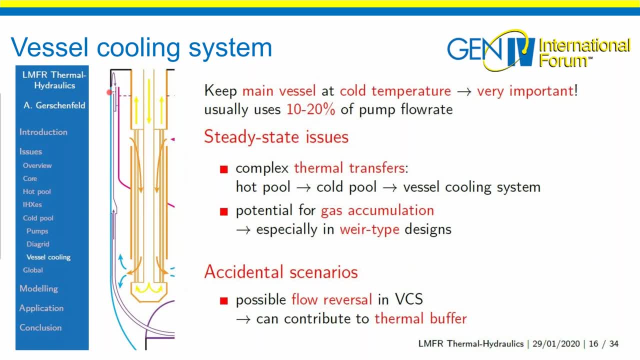 have liquid metal falling down like a fountain from the vessel cooling into the cold pool, then you may need, you may have, bubble entrainments at the bottom of this wheel type design, and so this is a there is a potential for gas accumulation right there. a final thing that can happen is that in an accidental scenario where you have what we 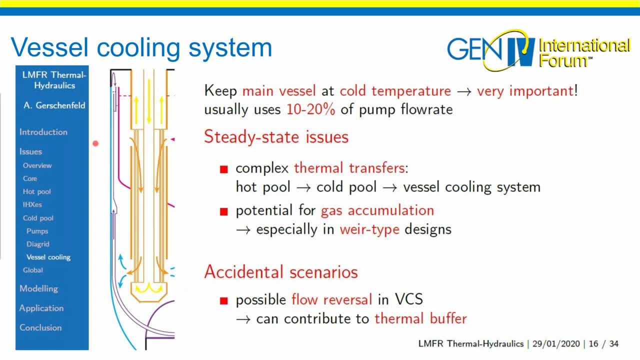 call a reactor vessel cooling system. so you've got a cold source here, then you could have cooling of this vessel cooling system and you can have liquid metal going this way, cooling down and going straight below the core and contributing to the cooling of the core itself. so this is this can actually be a very good source of cooling. 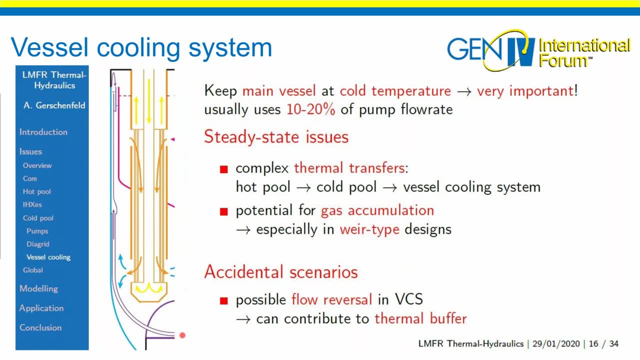 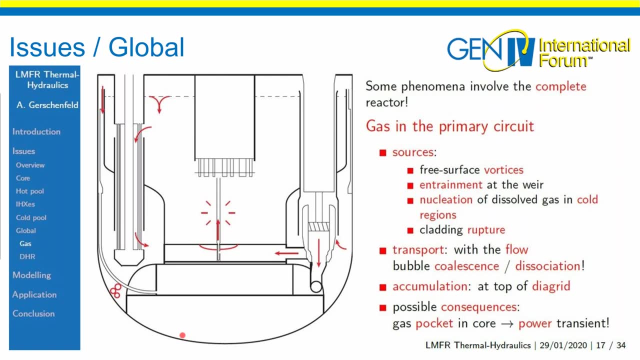 in a liquid metal fast reactor. it's the flow reversal in this kind of cooling system. and then, before we move on to the modeling i'll show, i'll talk about two issues that involve the complete primary circuit. so first one is this gas entrainment problem in sodium fast reactors. so 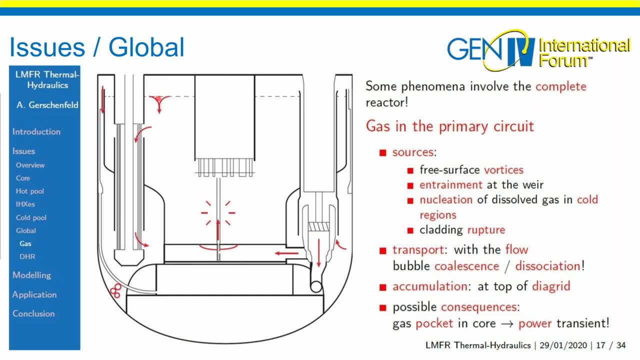 what can i? what can happen with this gas? you can have vortices forming at the top of the hot pool here and entraining bubble into the primary and then the flow of sodium will touch these bubbles and move them down into the rest of the circuit. you can also have, if you have a weird, a kind of wear at the top of the vessel. 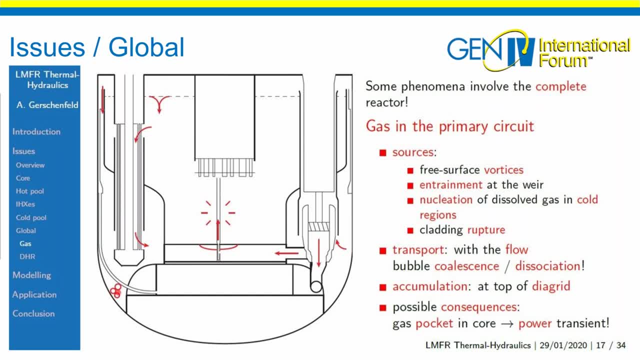 cooling system. you can have gas coming down from here, and also here you could have. these are dissolved gase nucleating in the coolest part of the reactor. so Here you will have hot liquid metal and so a higher solubility threshold for gas, And here, because the temperature is lower, this dissolved gas may nucleate and give you additional bubbles. 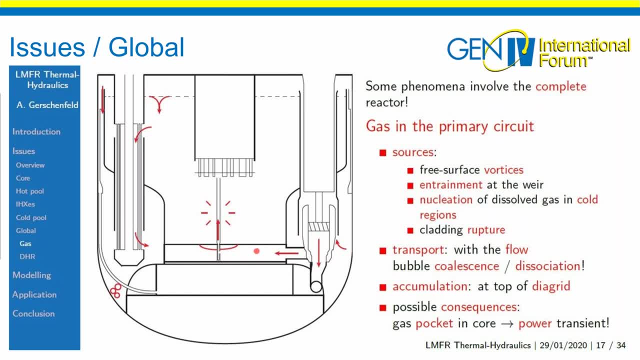 And then all this can be moved around and potentially accumulate at the bottom of the diagrid right here. So because usually the inlets of the sub-assembly will be in the middle, there is some kind of dead zone at the top and you can have a pocket of gas accumulating in this somewhat dead top part of the diagrid. 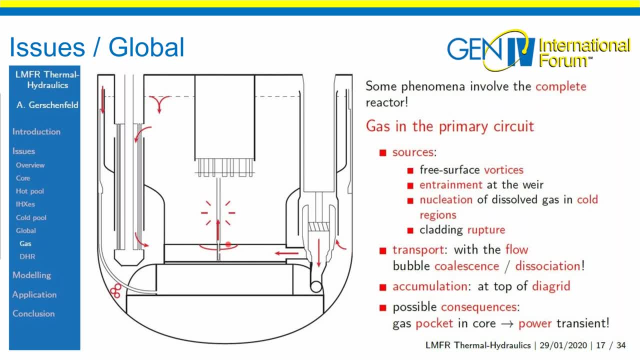 And then the worrisome consequence would be that if you change the speed of the pumps, for instance, you could have this pocket that had accumulated in the past moving all at once into the core, transferring into the core and causing positive reactivity events. 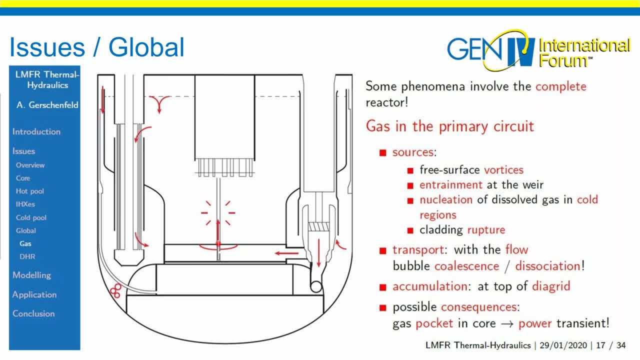 So we need to assess that no pocket large enough to disrupt the core can accumulate, And in order to do that, we need both to control for all of these sources and then use specific systems to ensure that no large pocket can form below the core. 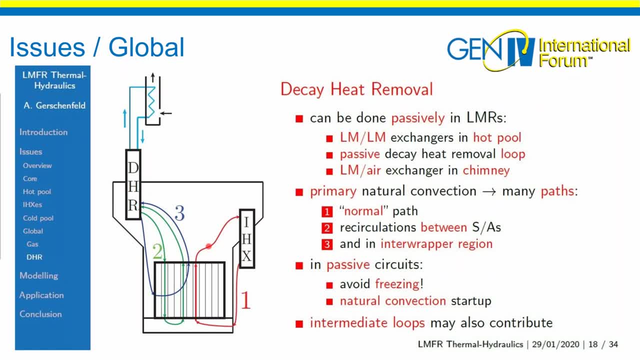 Another issue that I'll cover in more detail later is the decay heat removal modes in liquid metal core-type reactors. So a big advantage of this liquid metal reactor is that it can be used in a variety of ways. One of the advantages of the liquid metal reactor is that we can have completely passive decay heat removal. 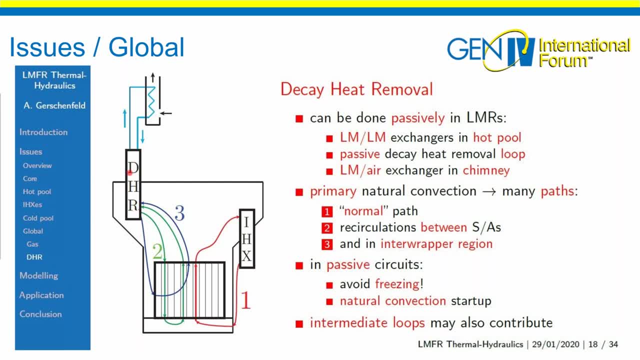 Usually what we do is that we insert a specific heat exchanger in the hot pool at the top and we connect this exchanger to a liquid metal circuit that can operate in natural convection. So we connect the other end to an exchanger in a chimney like this that will actually be cooled down by air. 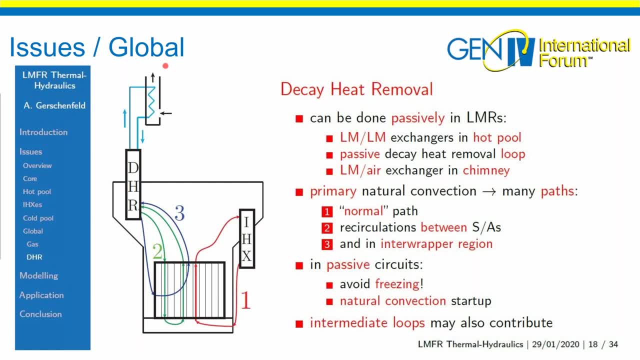 And so air will be our final heat removal source, And this never goes away. So we connect the other end to a heat exchanger in a chimney like this. That would actually be cooled down by air goes away, and so you will have cooling here, natural convection in this circuit. 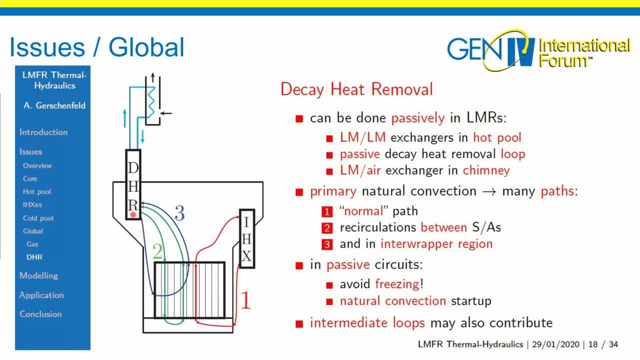 and cooling will be providing at the top of the pool like this. and then the question becomes: how does heat go from the core right here to this exchanger right there? and the answer is that in a cool-type reactor it's quite complicated. you can have the normal flow path like here's, like this. so path number one is liquid. 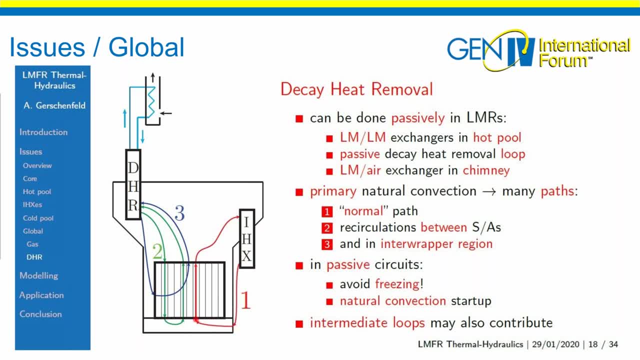 metal coming down into the cold pool, into the pumps below the diagram and moving up in the core doing the normal path. but you can also have cool liquid metal coming down at the outside of the hot pool, coming down in the cooler sub assemblies in the core, doing a u-turn below and coming back up. so this is a 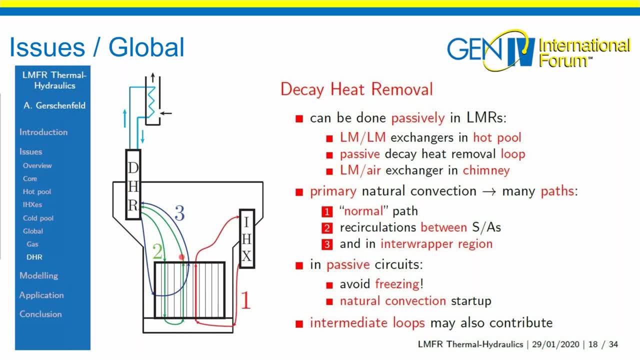 recirculation loop between sub assemblies. the final thing you can have is that this same, this same cold liquid metal can actually go down on the outside of the core and then move around between the sub assemblies in this inter upper region like this, and then it can cool subassemblies from the 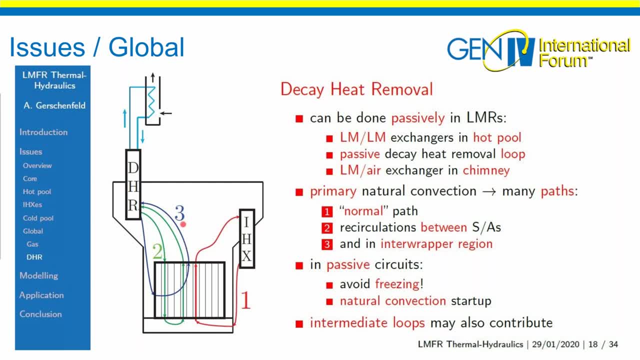 outside, heat up, come back up and contribute to core cooling. so this, so the first challenge is to model all this flow path correctly, to know what's going to happen at the level of the core itself. another possible issue is in this circuit, right here, because usually this: 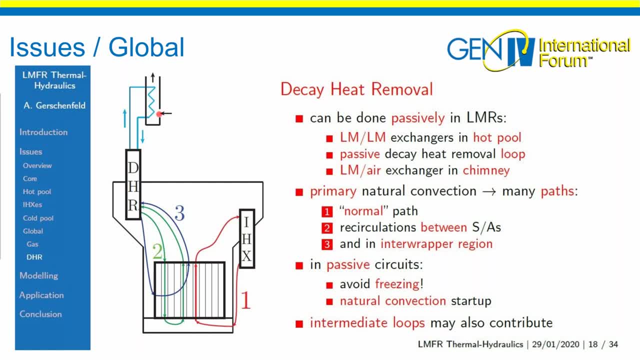 will be stopped in normal operation, and then you will have to start it when a loss of heating happens, and so the first issue is that you need to ensure that, during startup, the temperature will not go down in this part too fast, and so you will not have freezing in this part, which would 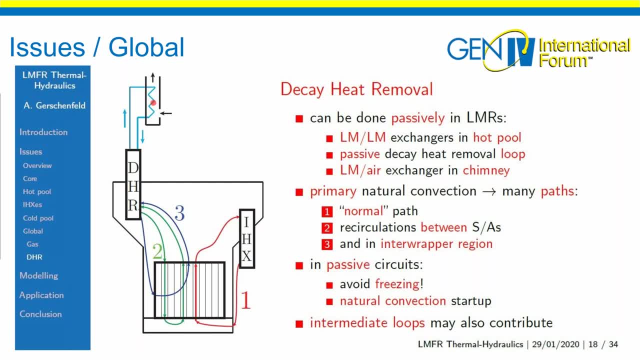 completely stop the overall flow. and then another thing you need to ensure is that the natural convection like this will start up on time and will not have trouble. also, a potential interest is that the intermediate loops connected to these exchangers may contribute to the removal of decay. 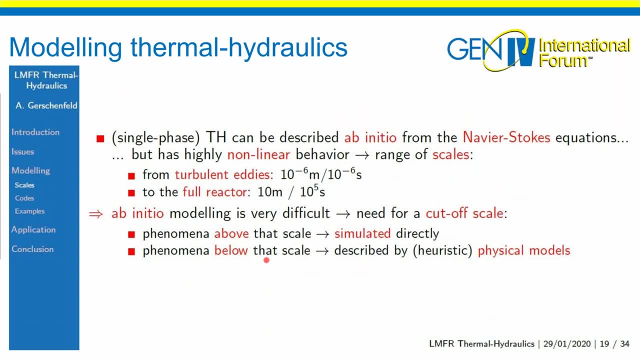 heat, at least at the beginning. all right. so now that we've seen all these interesting from algorithmic problems, one thing we need, we need, what we want to know is how do we describe them, how do we model them, and there is both good news and bad news. the good news is that 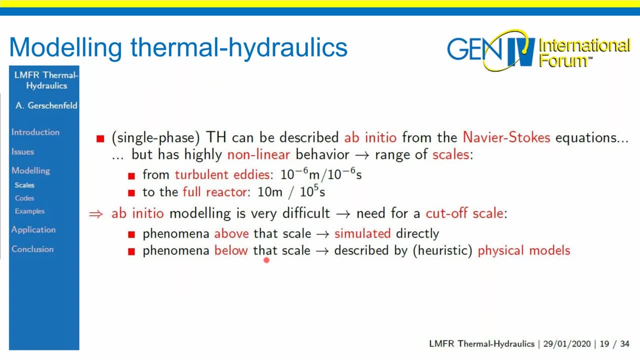 for formal hydraulics, especially in single phase. so if we don't have to deal with liquid metal vapor, then we've got the Navier-Stokes equations which can describe, or which can describe, what is going to happen ab initio from first principles. the only problem is that these equations are not 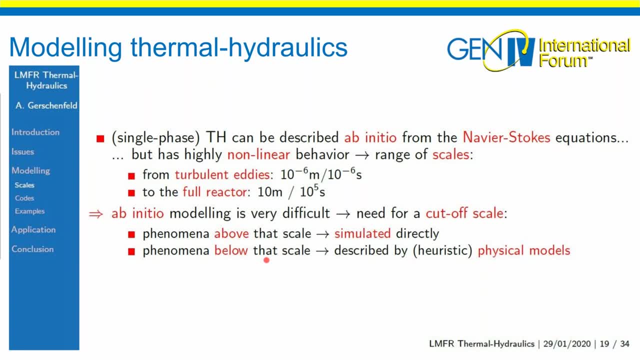 linear and they induce turbulence. they induce a lot of small fluctuations. it do so typically. if we want to do an ab initio simulation like this, you will need to go all the way from a, the small turbulent fluctuation in the reactors, which will be of a scale around one micrometer, and 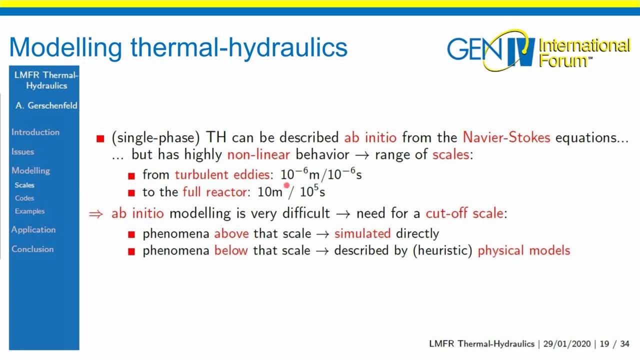 around one microsecond all the way to the complete reactor itself, which will be over around 10 meters big, and maybe you will have to simulate something like 100 000 seconds a few days. and this simulating from this scale to this scale maybe may be possible before I retire, but is not very likely. 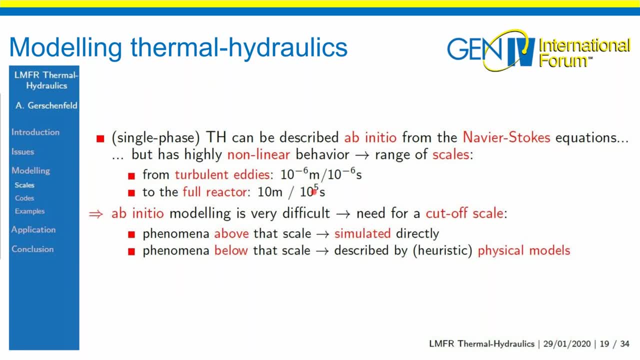 and so, because the this ab initio modeling is very heavy on the confusion on the computational side and not not practical in a real situation, we need to do something more, and what we do is that we introduce what we call a cutoff scale, so we we fix ourselves a given scale and all phenomena above 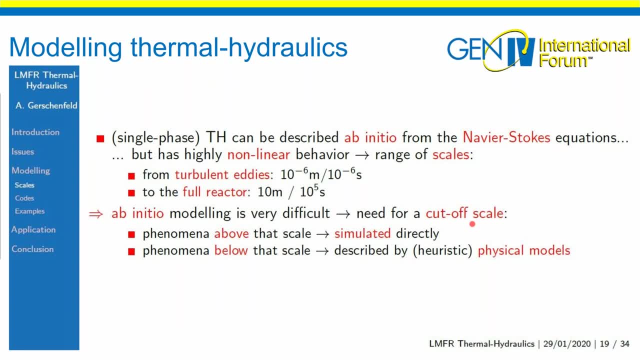 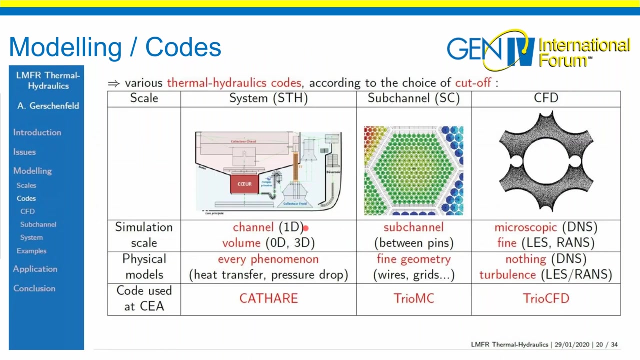 that scale. we will aim to simulate directly by simulating the equation with computer programs. okay, so everything that is smaller then we will not be able to simulate directly, and so we need to introduce what we call physical models or correlation to describe this phenomena and introduce them into what we have to we can actually simulate. so when we, when we go into 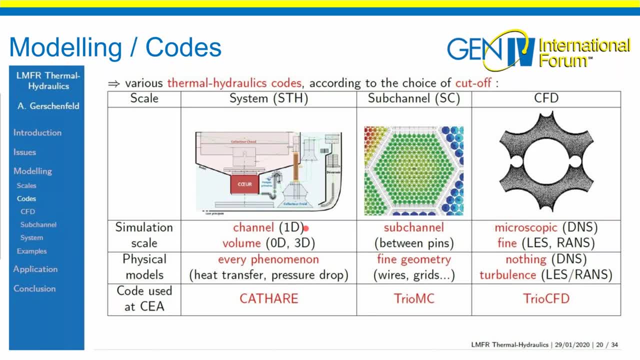 actual practical application. what thermal algorithm specialists did is that they chose different values for this kind of scale, the smallest. the smallest scale on the right is you have a very small or no cutoff, and this is if, if your cutoff is so small that you can describe the exact geometry of the reactor, so, for instance, the little wires between all of the of these pins. 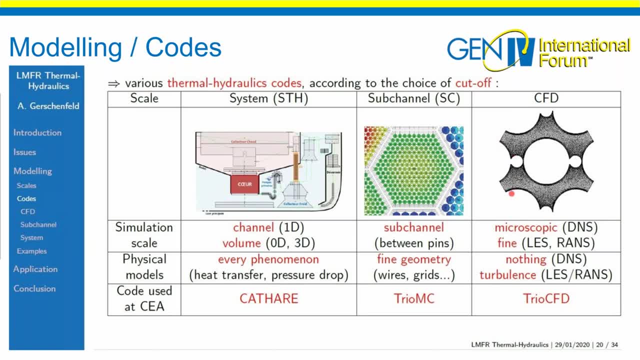 in the sub-assembly. then you will be doing what we call computational food dynamics of cm, and in this case the simulation scale will be very small. you will have a few physical models, not too much, but the computational cost will be very high. on the other hand, here this is what happens when you 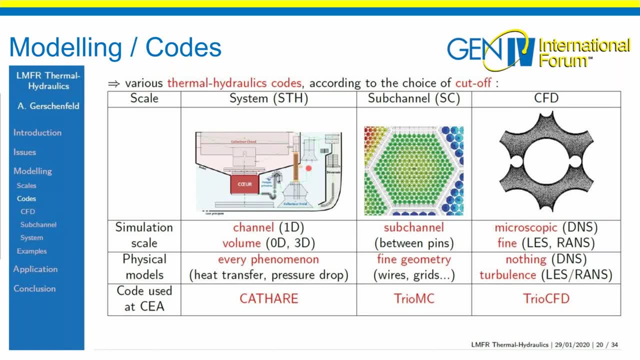 choose a very large cutoff scale. so here we have what we call the system scale or sth system from hydraulics, and this is a scale where, for instance, for the complete hot pool like this, you will have one big average value. in a little one, in a model like this for an exchanger, you will have 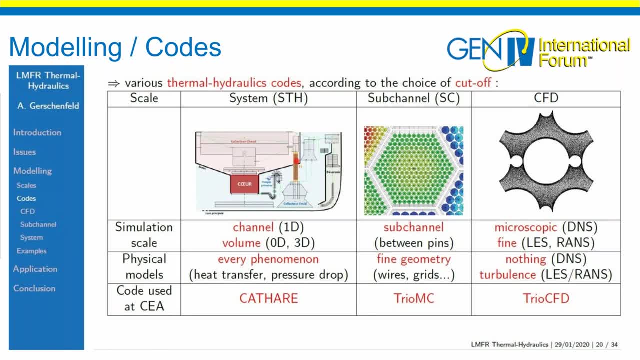 one average value in the 1d profile. so the computer, the computational cost will be very low, but on the other hand you will need a lot of physical models, actually for every phenomenon you need to model, and then sometimes you get something in between like this: so this is what happens when you are, when you, when you want, for instance, the local temperatures around. 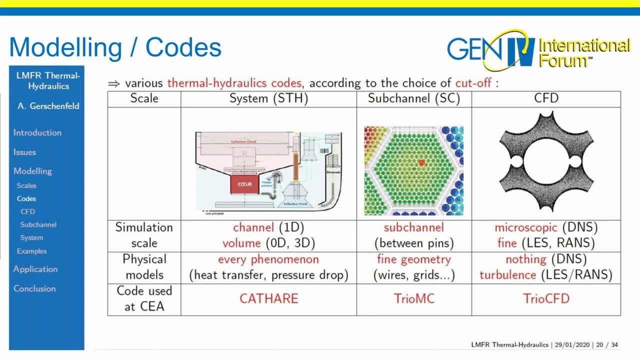 each fuel pin, and so you end up with something that is 3d, and this is what we call in this case the sub-channel scale. so you will have one temperature value between each trio of pins, and here you will need model for all the fine geometry that you cannot have. so, for instance, 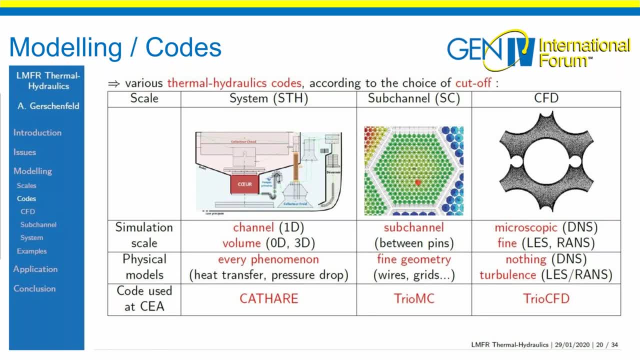 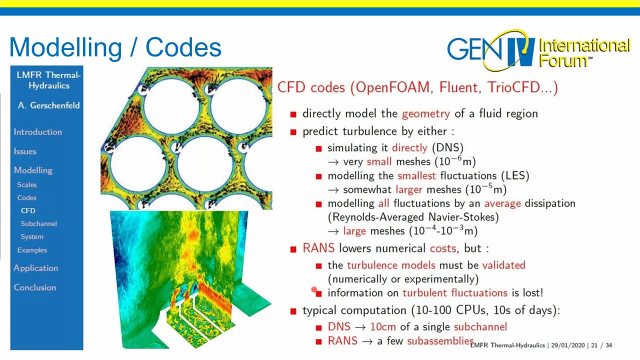 at this scale you cannot have see the wires and you will need physical models for the wires. and here, just for information, and again, i've given you the names of the codes we use at cea for liquid metals. so, going into a bit more detail we've got. so first, going from the finest to the biggest, 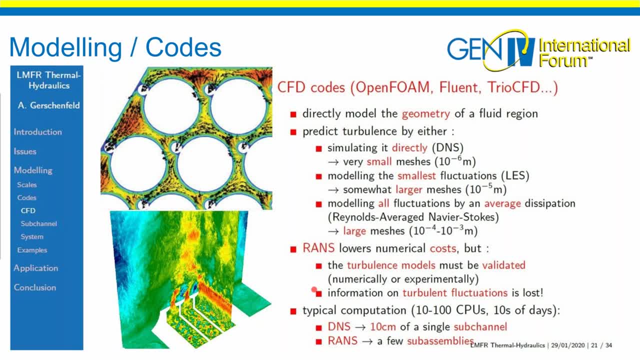 first we encounter cfd. so, as i said, cfd is when you model all the geometry of the reactor or of a local part directly. so the the geometry, you is above your cutoff scale. what is not above your cutoff scale is all these small turbulent fluctuations, and there you have pre-choices. the first one is you simulate everything. so this is: 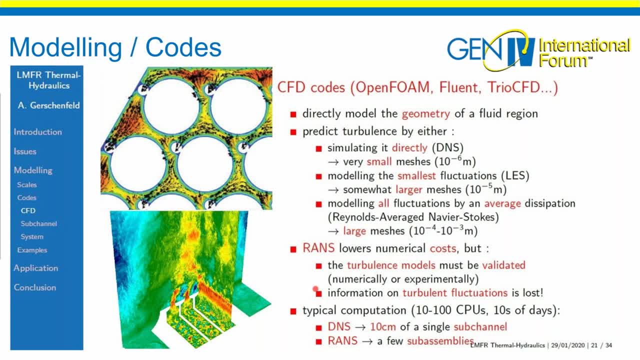 what we call direct numerical simulation of dns, and it requires some very small computational measures, one micrometer you can. also you can choose to more to model, so to not directly simulate the smallest turbulent fluctuations, and this is what we call less turbulent fluctuations simulations, and this can allow you to to have somewhat bigger measures, so you gain usually a. 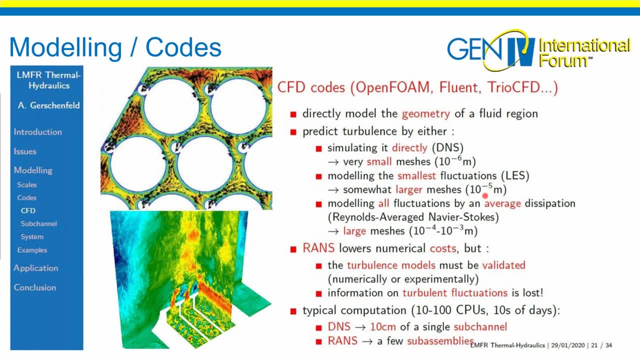 factor of 10 to 100, and this decreases the computational cost at the cost of a physical model for the small fluctuation. and finally, you've got the option of trying to have all turbulent fluctuations below your cutoff scale, so you need to model everything from turbulence. 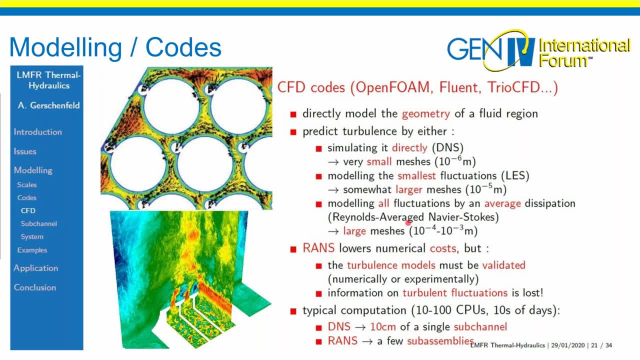 with a physical model, and this is what we call reynolds average navier stocks, and if you do this, normally you can use the mesh size that is only given by do family features. so this usually allows for meshes that are from 0.1 to 1 millimeter in size. so this rant lowers numerical cost, but 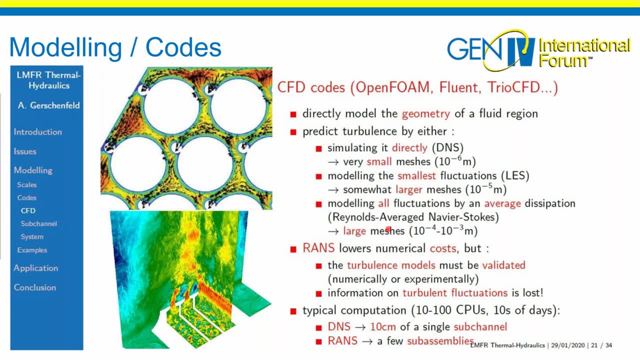 you have to introduce physical models, and this is mainly what we call turbulence models, and they will need to be validated, either against the final simulation that would go directly simulate the turbulence and not hurricane modulation, unless there is another cost- well, if you want to actually turbulence, or using an experiment, and, of course, if you do a simulation where the turbulence is. 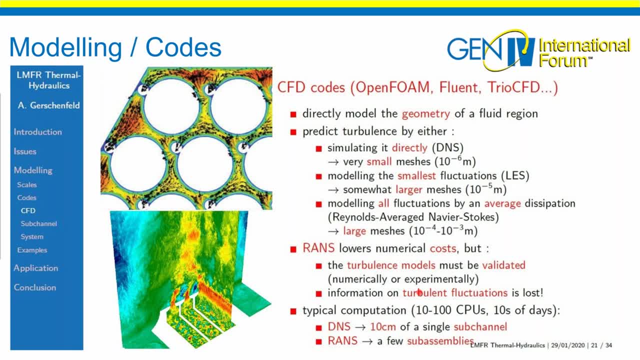 described by your model, then you will lose information on all the turbulent fluctuations like, for instance, in this picture, a Japanese experiment. so this is actually a nocillatory behavior between a hot and cold jet and if you do a Reynolds average Navier-Stokes simulation, this 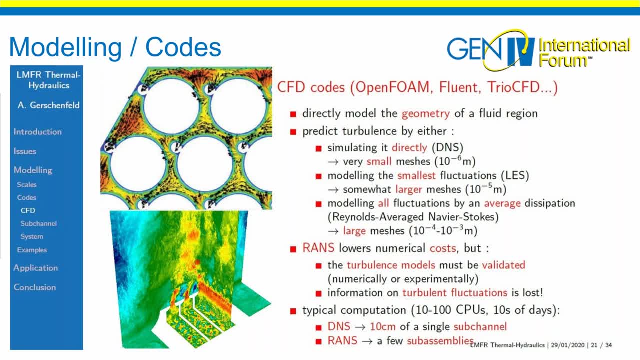 fluctuations will not be available to the simulation. so here are two examples of what we typically can do. if you want to do a direct numerical simulation, usually the best we can do is, for instance, a few like 10 centimeters in height in a single sub channel between three. 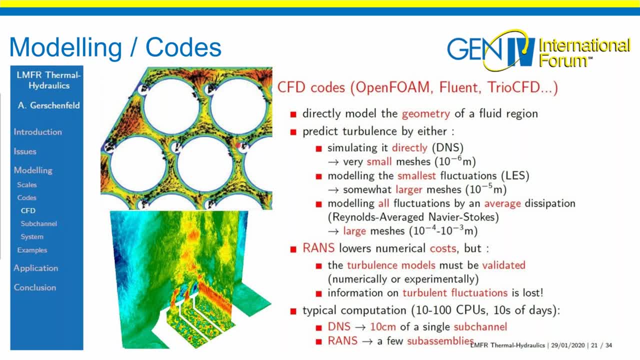 pins and the sub assembly. so this is very expensive and we can only do a small region and on the other hand, if you, if you use when the rents the Reynolds average Navier-Stokes, then usually the cost is so much lower that you can get to model. 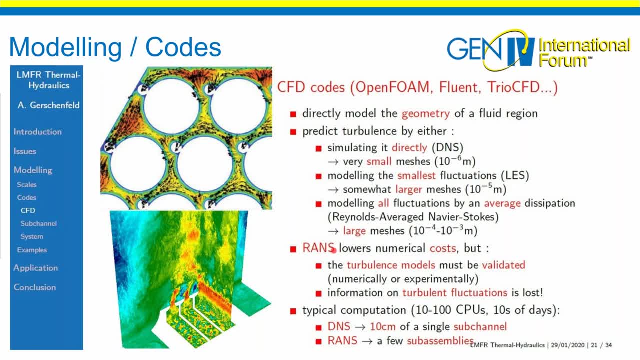 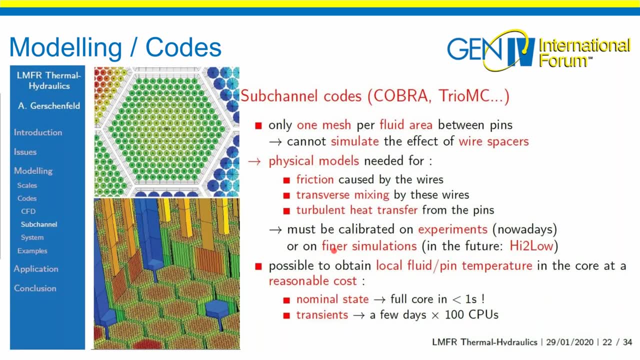 a few sub assemblies in their entirety so you can see the gain between direct simulation and the rents, then moving up in cutoff scale to the sub channel. so these are codes where you have one mesh, one computational mesh per fluid interstice between two pins. so this is something 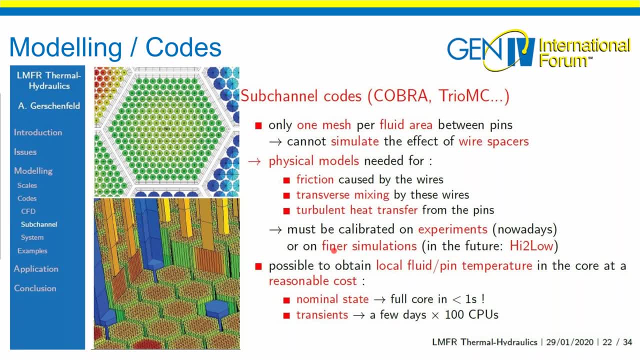 you can use to simulate the. so they both. they have a tendency to increase friction in the bundle, but they also induce mixing between neighboring channels. and the next thing you need to model is what the actual transfer- heat transfer- is between the pins and the fluid. this is something that we can do in the model. 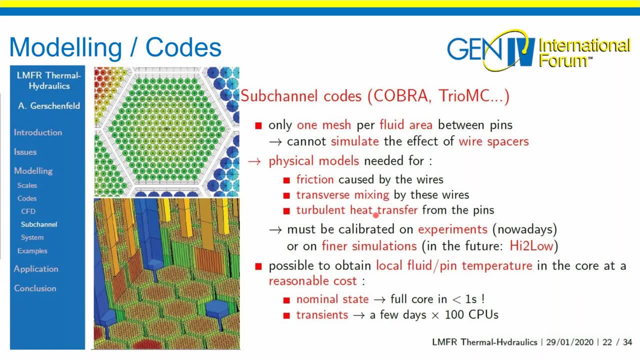 this is something that needs to be calibrated on experiments or, what's more, the most fashionable thing today is to do a fine simulations and use and use this to calibrate the coarser model. this is what is called high to low, and so the going to this course of spray, course of scale, has a very 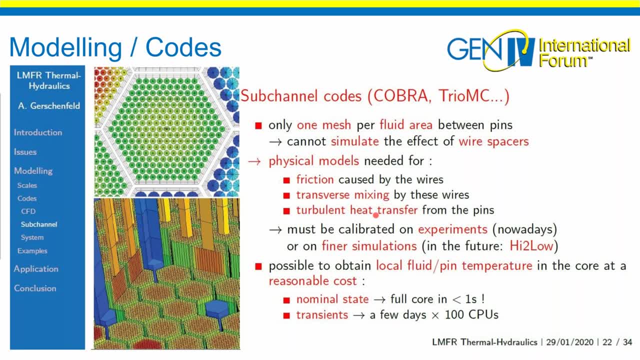 big advantage over CFD in compute in terms of computational cost. so, for instance, if you are only interested in in a steady state, you can usually use this curve to calculate the frequency of the transfer heat transfer codes to get the full steady state of your core. 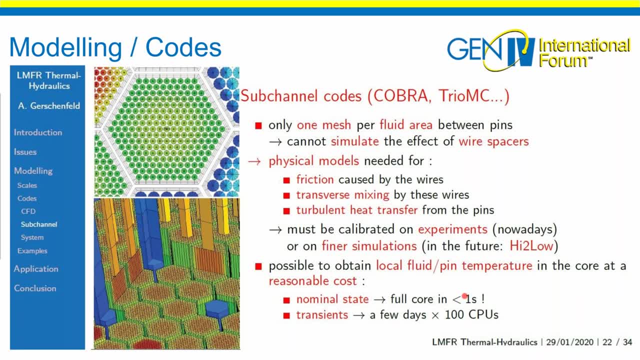 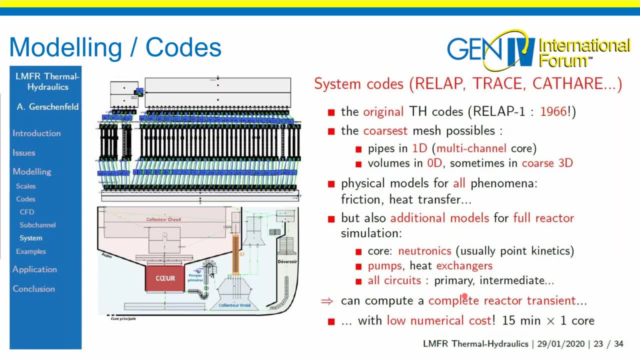 in less than one second, very fast. If what you want to compute is a transient state, it will take a little more effort, but it's perfectly doable. And then moving all the way up into the system codes. So first you should know that these 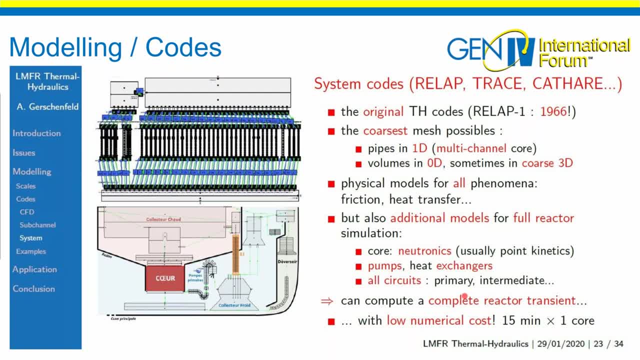 are actually the original from hydraulics calculation tools. The first one relapse. one is from 1966. They use the coarsest mesh possible. So you've got pipes like the heat exchanger here. You do them in 1D. 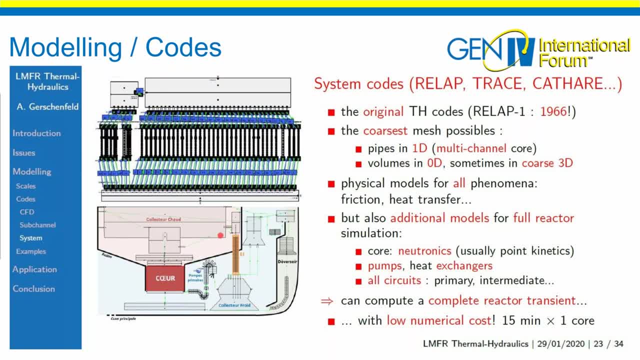 And big volumes. you do them with one big average value like 0D, or maybe sometimes a coarse 3D. You need physical models for everything so friction, heat transfer and so on, And also what's interesting in this code. 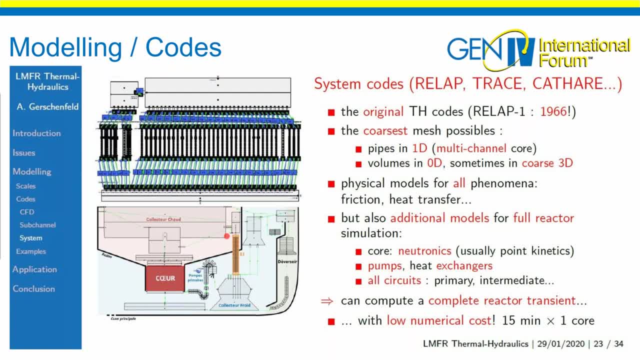 is that usually they include additional models for stimulating a complete reactor transaxle. So, for instance, they tend to have a model for the core neutrality. It works with point kinetics usually, but some codes have some 3D kinetics So you can compute the power, the evolution of the power. 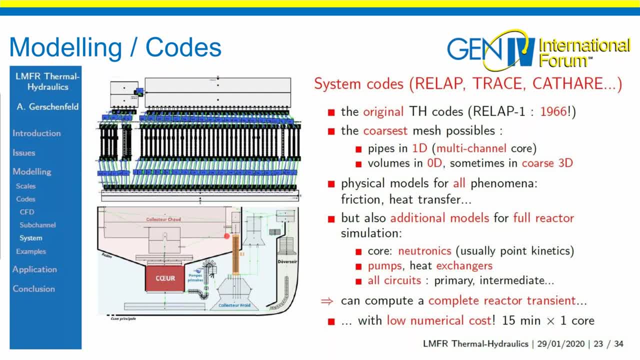 They have modules for pumps, for heat exchangers. And another interesting thing with this code is that they can simulate several circuits, So you can have, for instance, the primary circuit, the intermediate circuit and the power conversion system in the same simulation. 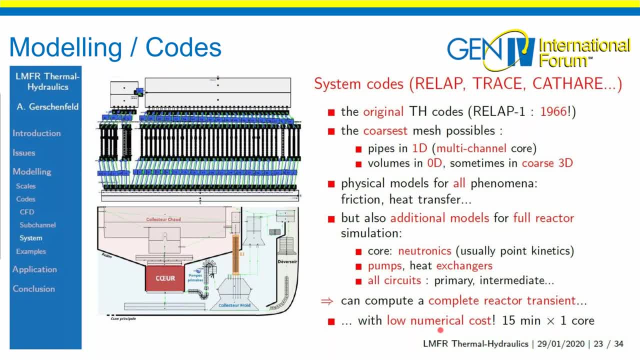 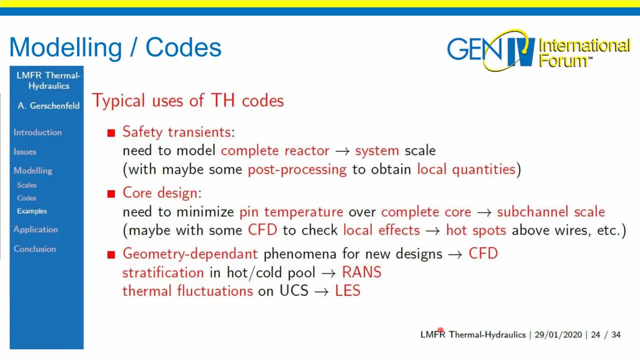 And they do all this with a very low numerical cost. It's very rare to have a system-scale simulation that is longer than 15 minutes on your own computer, And so when you look at the type of issues we have, usually what will happen is that, if you 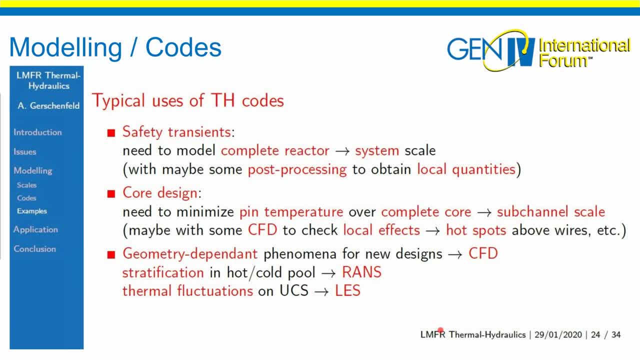 want to model a safety transient, an accidental transient where some pump stop or the reactor is cramped, and so on. you need to model the complete reactor, And so only the system-scale has all you need. They've got all the models and they. 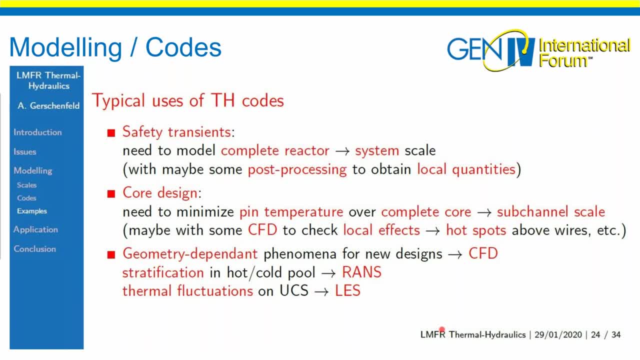 can describe the complete reactor at a low cost. So this is what you would typically use for a transient. If you want to do something like core design- minimizing the maximum pin temperature over the complete core- then a typical tool will be this sub-channel scale, because it's 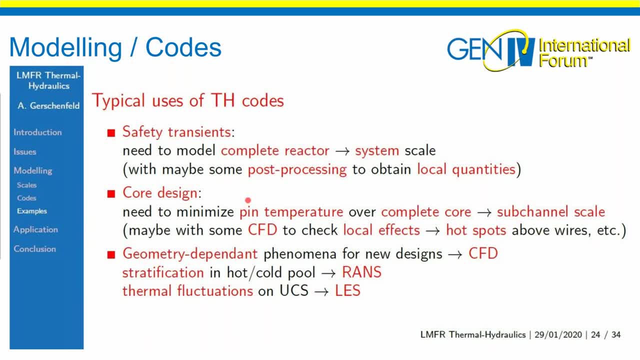 going to give you the per-pin temperature maximum for all of the core at a low cost, And sometimes maybe you will want to know some more about local effects, And in this case you can use CFD of some kind, Some specific faces. 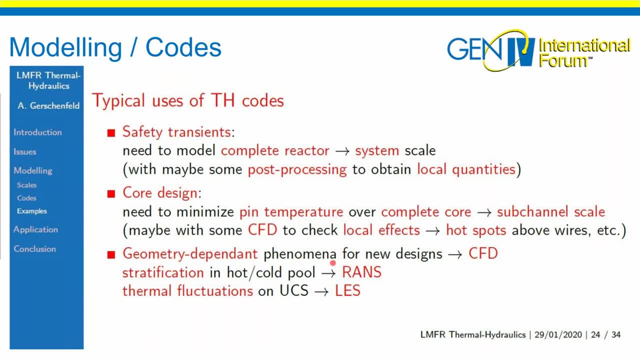 And then if you've got some more complicated geometry-dependent phenomena, then the typical tool of choice will be CFD. So if you want to model big 3D evolution in the big pools, for instance rents, so CFD that models turbulence. 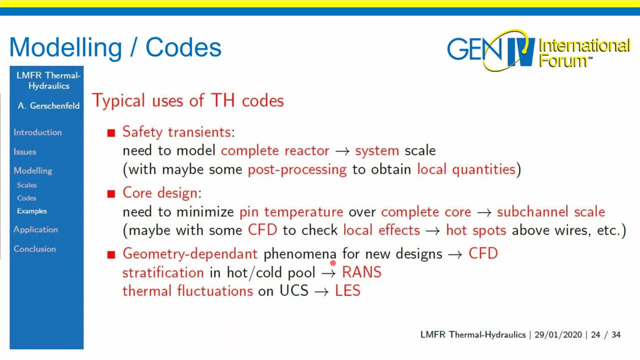 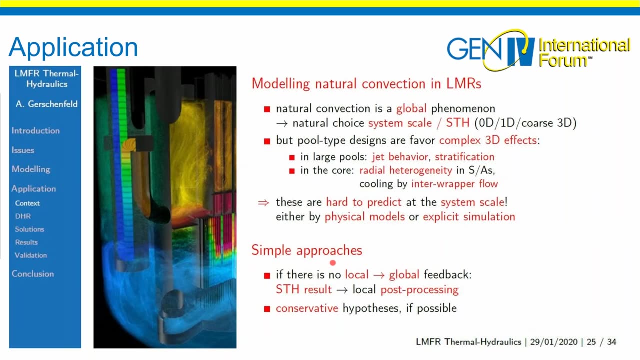 would be the tool of choice, And if you want to model something that will depend on thermal fluctuations, that are related to turbulence, then the typical tool would be LE, And then you've got some cases where nothing works. So this will be actually my example applications. 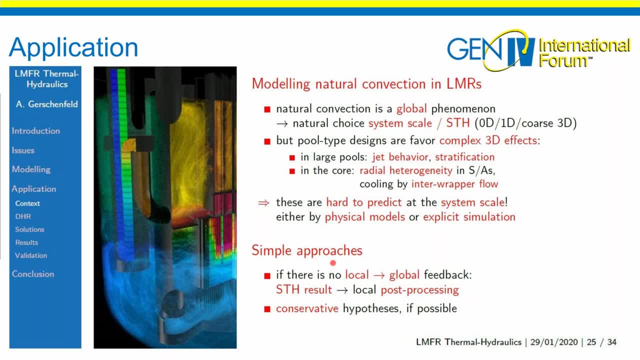 for all of this And it's going to be the modeling of natural convection in nuclear metal reactors. So natural convection, by essence that is a global phenomenon. It involves the complete primary circuit and maybe some other parts of the reactor. 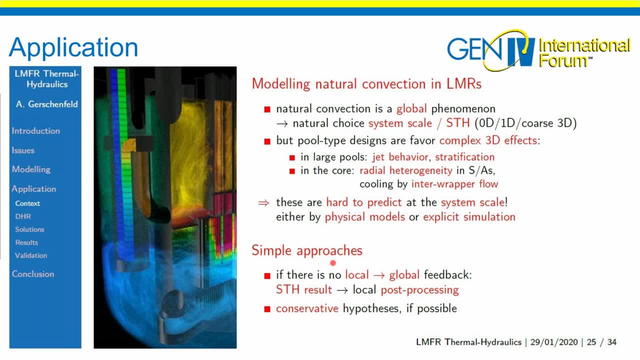 So the natural choice is the system scale, But the problem is that With our reactor designs, with big pools of liquid metal all over the primary circuit, this is something that is hard to describe if you only have volume 0D or 1D components. 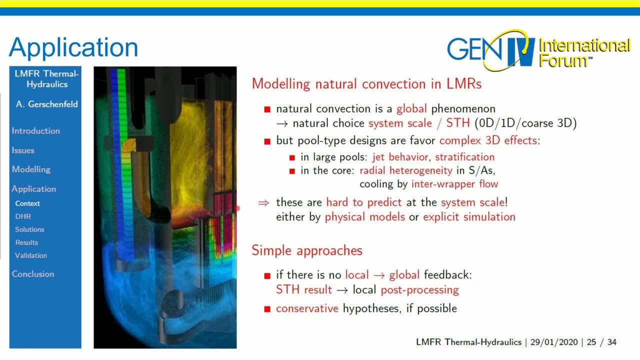 that you network together. One phenomena of interest, for instance, is the behavior of the outlet jet in the hot pool, and if you will have stratification Or maybe the possibility of interoperable cooling between the hot pool and the core, You also have this. 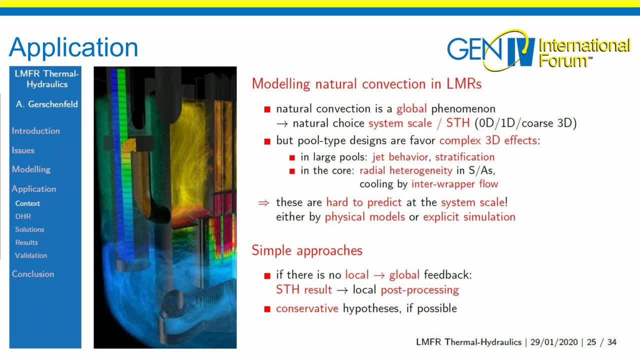 These radially heterogeneities between subassemblies. that would have an effect And you could try to introduce physical models in the system code, but they are going to be very both dependent on geometry and transients And so it's complicated. It's very hard to introduce physical models as well. 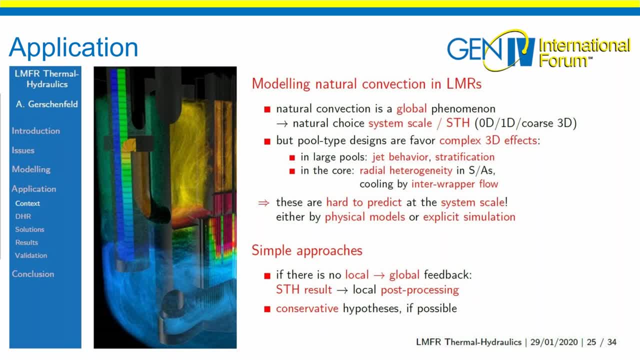 So the first thing you can do- and this was done in the past- is that the first thing is if you are studying a transient where you may have local effects that are hard to simulate, but they have no consequences on the overall behavior of the transient, 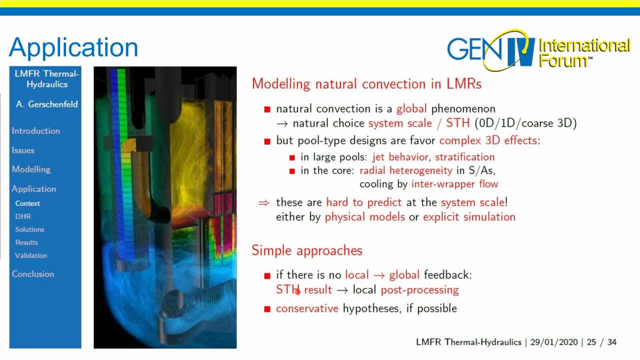 Then you can just do your system scale, simulation, core scale- and then do some kind of post-processing with a finer code. If there is an effect but you don't want to model it or describe it in detail, you can take conservative apotheosis. 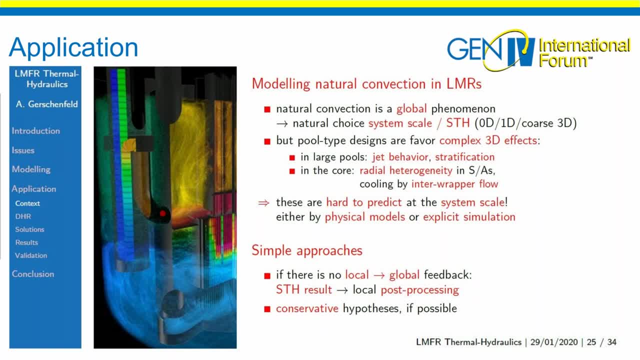 For instance, you can say: I don't really know what the inlet temperature in this pipe will be, but I will take the worst possible value, for instance the one coming out of the core here, and I take that coming into the core. 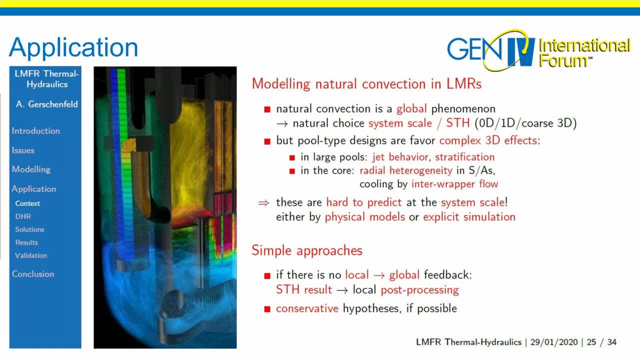 and I will get a conservative model, But maybe with more recent design it would be interesting to reduce this conservative hypothesis, to have some more margins and optimize the reactor design. So it's a big motivation. There is a big motivation to move beyond these two. 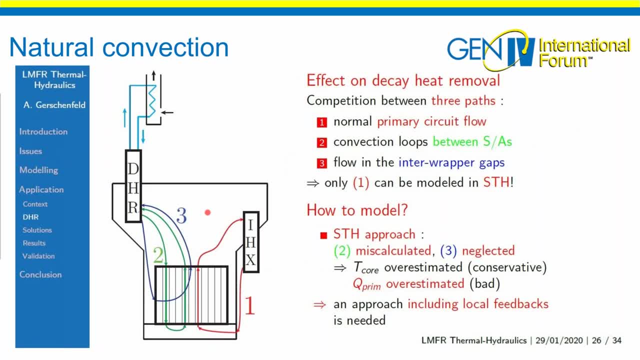 simple approaches. So when you, When you look at the actual situation- so I can, So this diagram comes up again- When you look at these three competing paths for moving heat from the core to this decadal heat removal heat exchanger, you have path one, normal flow path, two, recirculation loops. 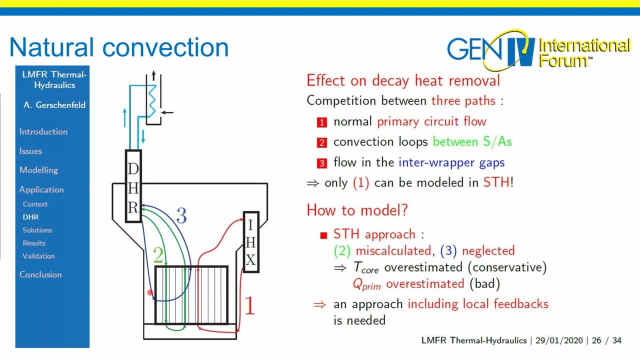 between sub-assemblies and path number three: recirculation loops in the interwaffle gaps. If you have the standard system scale approach, the only thing you can model more or less correctly is this path number one because, for instance, 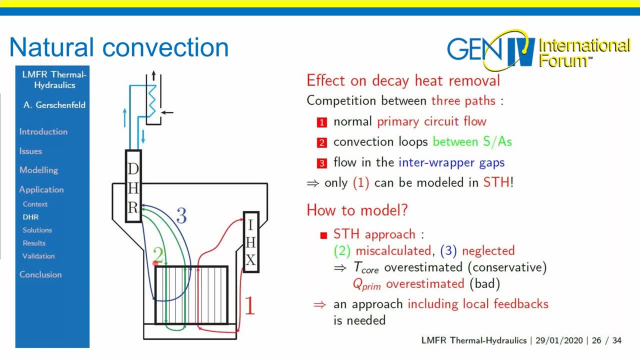 trying to model path number two. you need to know what the temperatures are inside the hot pool. If you have one big average value between this part and this part, then computing the flow here will be completely inaccurate. This path going between the sub-assemblies- 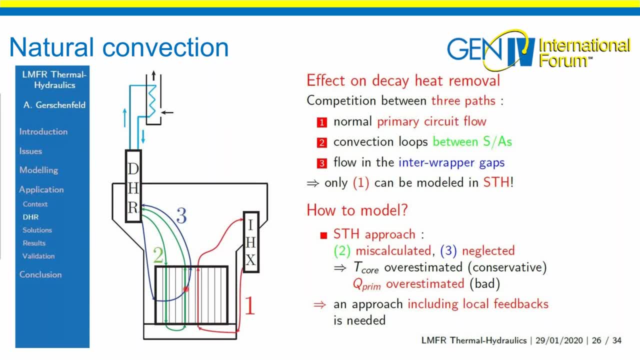 it requires knowing the 3D temperature inside the sub-assemblies and the heat conduction through the interwaffle gap. And same thing it's very hard to model in STH. So usually with the system scale approach you compute this but it's not accurate. 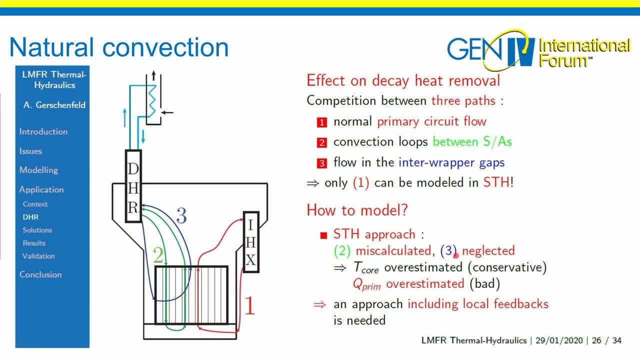 And this one, number three, the interwaffle flow, is neglected. So what's going to actually happen is that, because you have removed some mechanism for decay heat removal, the core temperature will tend to be higher in the simulation than in the real. 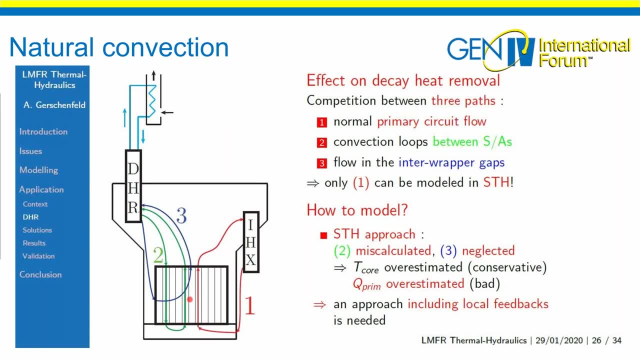 case, which is actually OK. It's conservative- But you will also overestimate the amount of work done by this path number one. This means that you will overestimate the primary flow rate And this will lead you to increasing problems for the average temperature on this side. 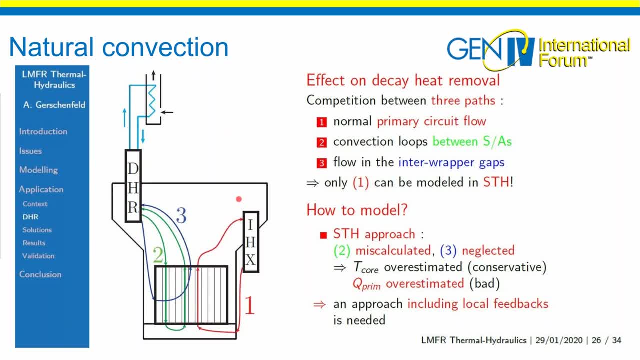 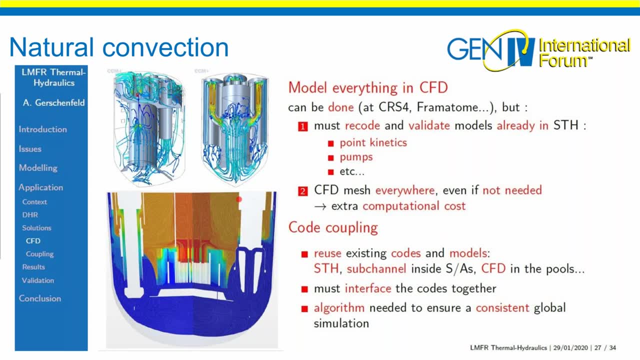 average temperature for this side on one and can potentially be bad, And so you need an approach where you can somehow model these other two paths. So the first thing you can do is that you can say: OK, let's look at all the tools at my disposal. 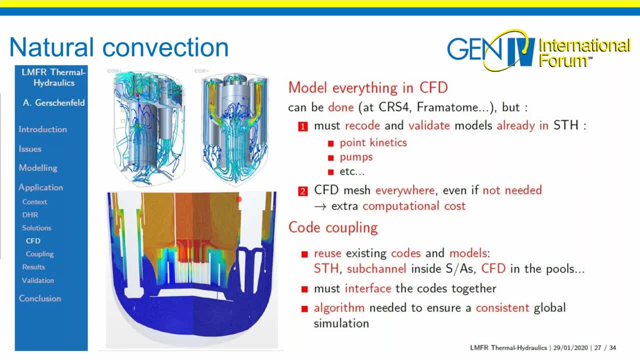 and I will choose the one that can model all these phenomena, And the one that you can use is CFD. This is what is required in the hot pool, in the cold pool and in the core, And what people have done is that they. 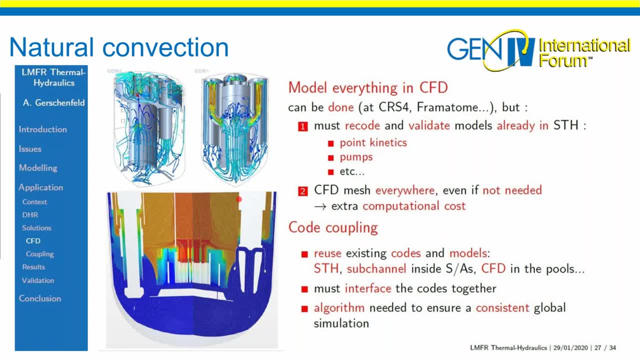 have done models of complete reactor primary circuits using the CFD code, And here you can see an example model of this For the for a lead-fast reactor, And here you can see the same for a sodium-fast reactor, And so this means that you can use the code you already have. 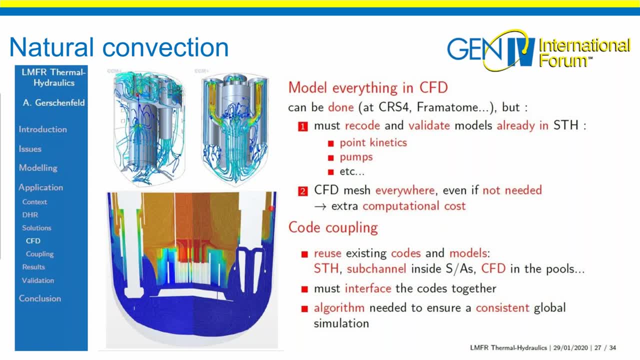 But at the same time it also means that you will need to re-implement the models that you already had in the system scale in order to model a reactor front end. So, for instance, the useful models are the point kinetics in the core. 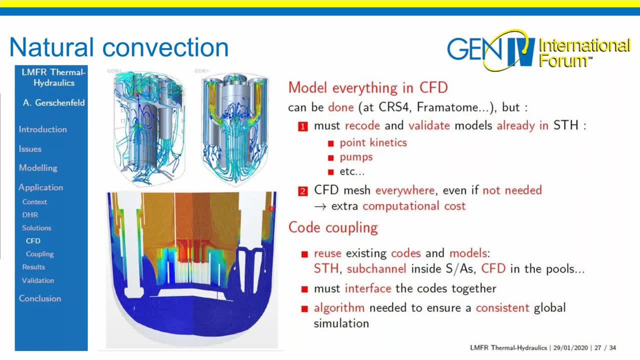 the pumps in the primary circuit and so on, And you will need to implement the models. You need to re-implement that in the transient simulation. Another potential cost is that if you do everything in CFD, you will have fine modeling in the regions that. 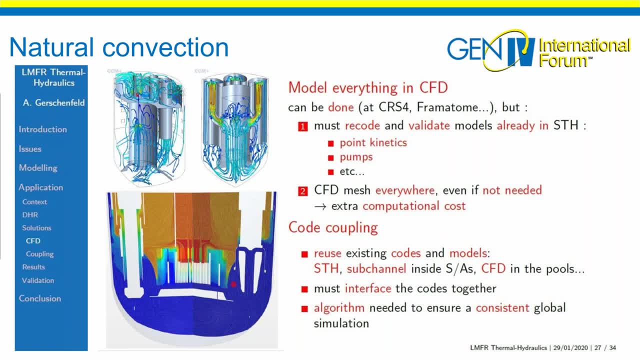 are of interest to you, So, for instance, the outlet of the core, the cold pool, But you will also have a 3D modeling of this diagram. here, for instance- And this is a region where there are no 3D effects- 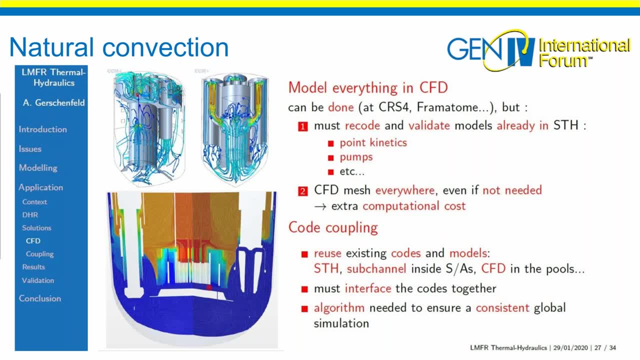 But you will still have a CFD mesh, And so you will pay for computational costs even where you do not need it. Another thing that you can do- and this is what we actually did in CEA- is that you can take the codes you already have. 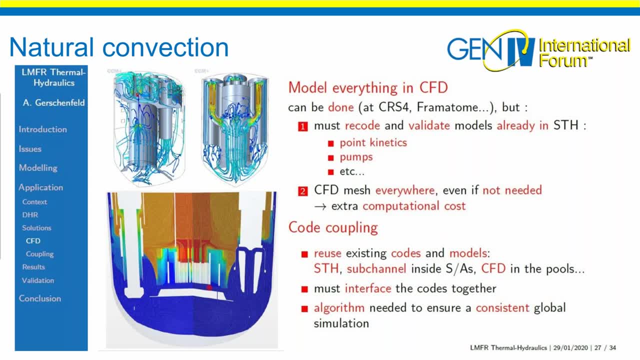 so system, subchannel, CFD and try to use them together. So, for instance, you would have the system scale And then inside the subassemblies you would use the subchannel scale, Inside the hot and cold pool you would use CFD. 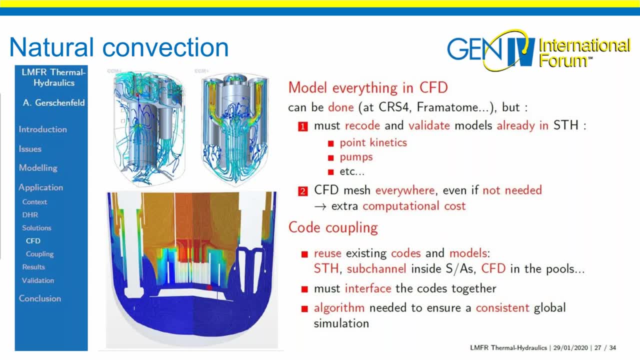 because you want to know the 3D behavior And this means you can have maximum reuse of the work you have already. But on the other hand, you will need to make all these codes work together And you will need an algorithm to ensure. 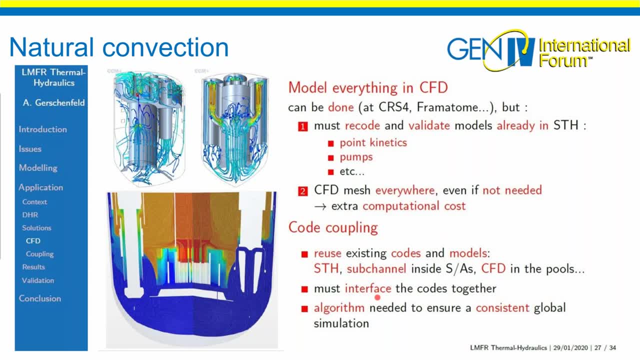 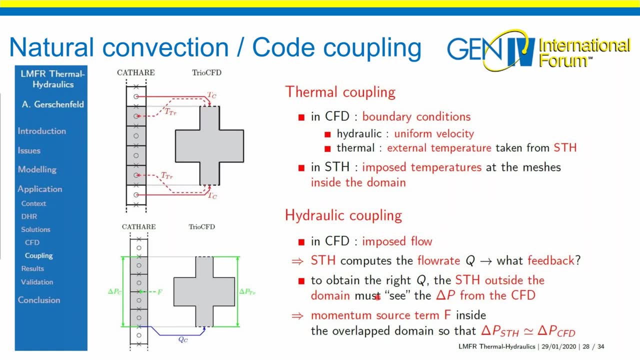 that, when all these codes work together, they're actually giving you three aspects of a consistent global simulation. And this is something you can do in a number of ways, And here I've given you as an example the way we use at CEA. 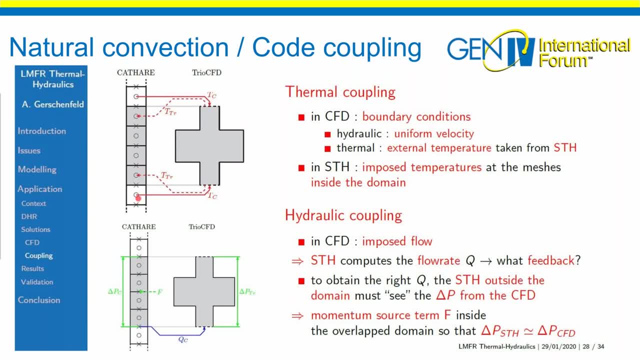 What we do is that initially we've got the system code here, So the course of code is actually present in the complete simulation, And then we decide that part of the simulation, which, for instance, could be the hot pool, is going to be overlaid with a finer CFD simulation. 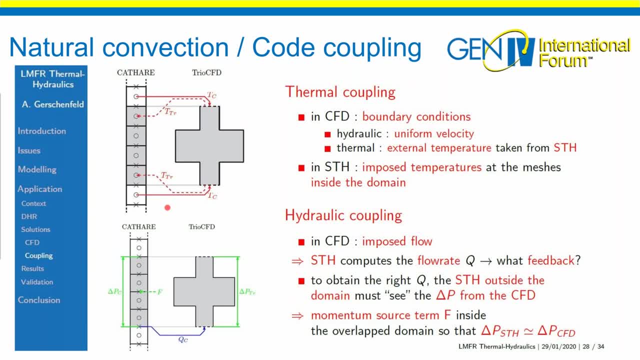 like right here. If you want to ensure that you have a consistent simulation where the system code is computing this part and the CFD is computing this part, what you can do is that, for instance, Once you take the temperature here from the system code, you impose it as a boundary condition. 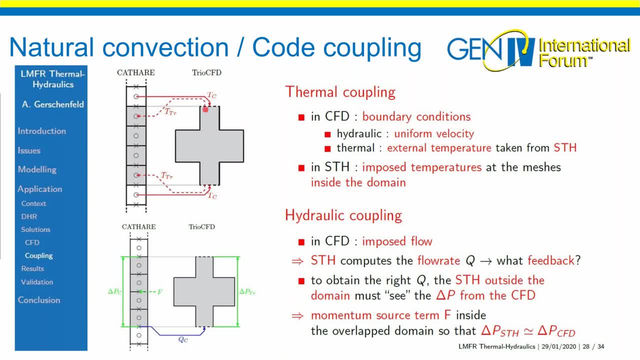 to the CFD and on the other end, for instance, here you take the average hot-tech temperature on the CFD and you impose it right on the inside of the system code And with this you can have a global energy conservation between the core system scale. 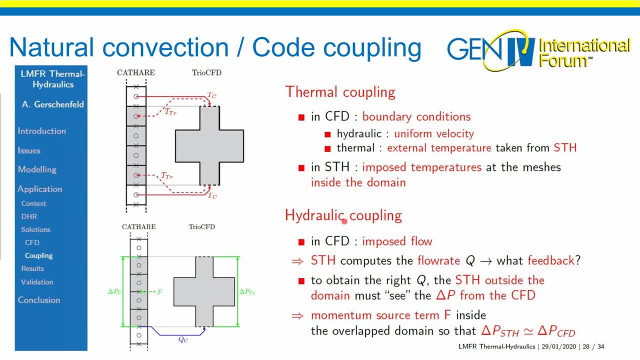 and the fine CFD scale. It's a bit more complicated when you consider the velocities and the pressures. So usually what you do is that you go to the system model, you measure the flow rate at this point and you impose it as a boundary condition to the final scale, the CFD. 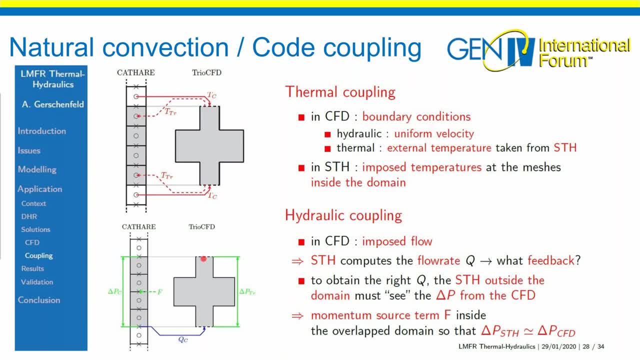 Because liquid metals are almost incompressible. then you will have the same flow coming out and you will not need to do anything. It's also going to come out on that end in the system side. What's interesting? The interesting thing is that 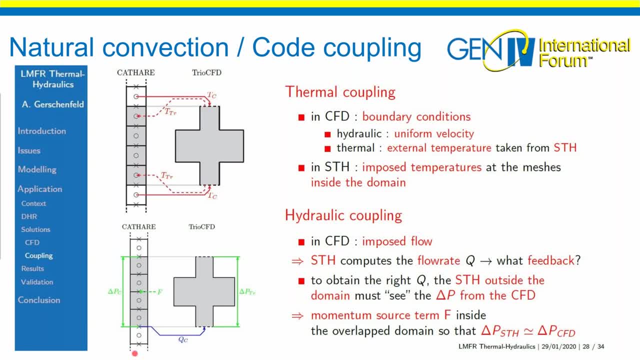 In a simulation like this, if you want to have a consistent picture between this side and this side, you need to ensure that the pressure difference between those two points in the system side is the same as the one predicted by the CFD code. So actually you need to do something extra. 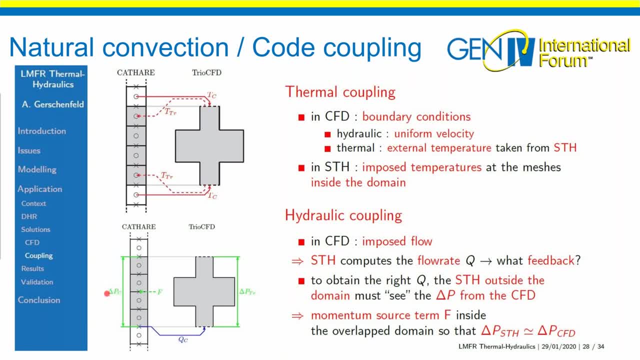 You need to change what the system code calculates for this in order to match the delta P on the CFD side. And this can be done by introducing a little What we call a momentum source term, an artificial force here, And this force, we adjust it in order to change the pressure difference on the system side. 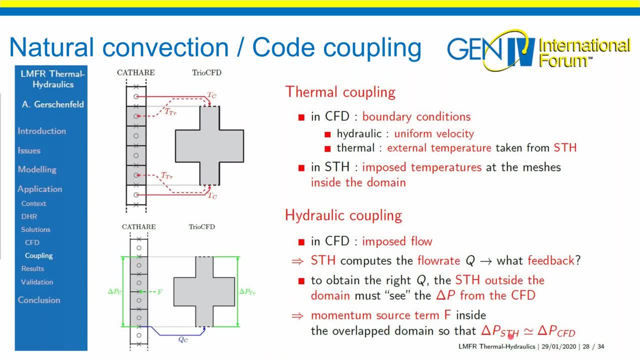 until we've got the same delta P on the system side as on the CFD side, And this is enough to ensure a consistent global simulation. On the other hand, it needs to be done as an iterative process. You need to try different values and pick the right one. 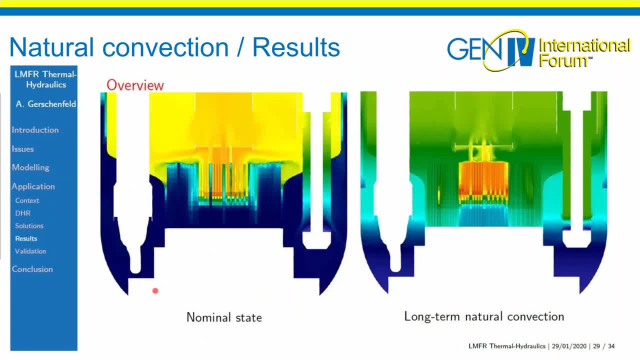 Okay. So once you do this you can do some complicated 3D simulation, complicated coupled simulation of a sodium-fast reactor going into natural convection. So here you have an example from the Astrid project at CEA. So this is the reactor in normal state. 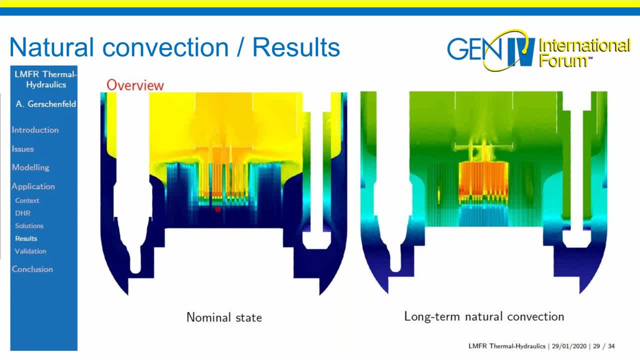 You've got the core at the sub-channel state, at the sub-channel scale Starting from this part. this is CFD. So here you can see The outer jet of the core, for instance, goes into the primary side of the heat exchangers. 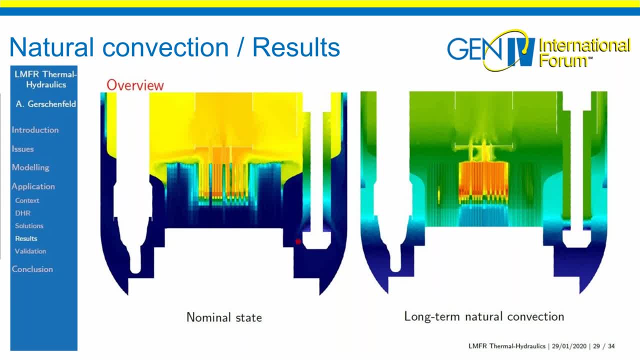 and into the cold pool with this outer jet here and finally into the pumps on this side and below the core. So, starting from the pumps, we are at the system scale with our system code CATAR, and we stay at the system scale until we go back into the core. 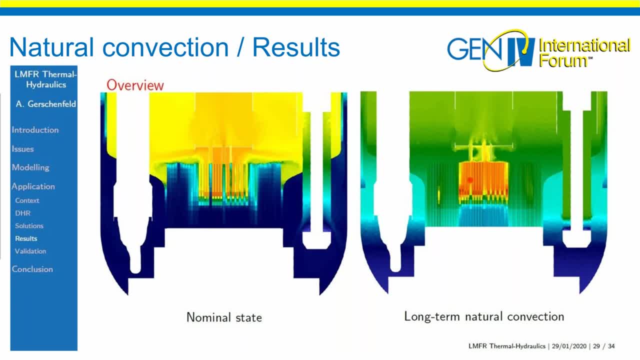 And in natural convection, the picture is completely different. At the outlet of the core, instead of having a strong outlet jet like this, you have a small chimney flow like this: You've got a chimney effect going all the way up from the core. 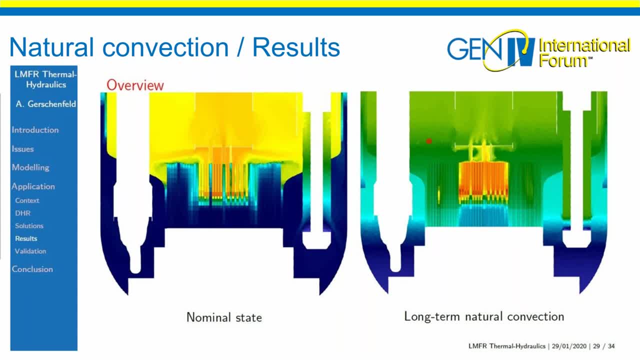 The hot pool itself is stratified. There is some hot sodium at the top, an interface in the middle and some cooler sodium at the bottom, And this is because you have this decay heat exchanger cooling down flow sodium in the hot pool and injecting cooler flow here. 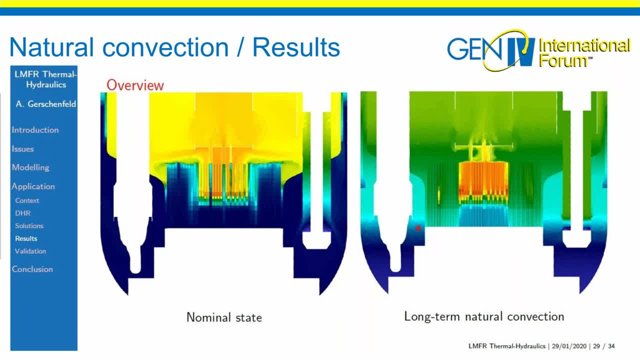 On the other side you have this decay heat exchanger cooling down flow sodium in the hot pool and injecting cooler flow here. Okay, So on the other side, on the cold pool, you also have stratification. The jet from the heat exchanger is no longer present. 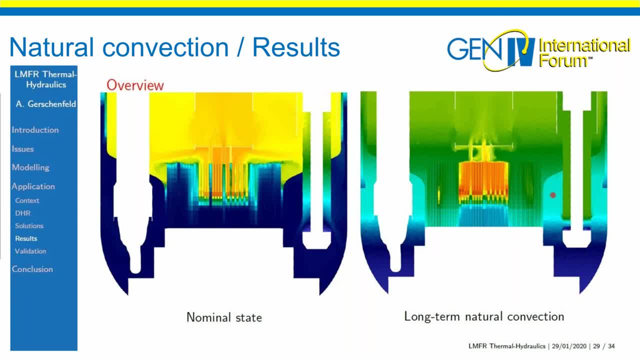 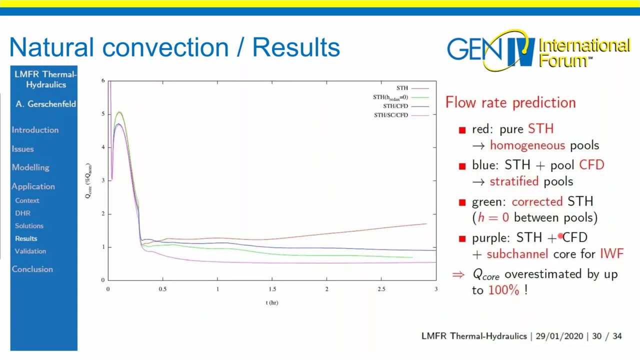 Instead you have this kind of completely stratified flow. The cold pool is not uniform anymore. You've got hotter sodium at the top and cooler sodium at the bottom, with a very strong interface, And in general, the situation is completely different. So when you look at the actual results from this, 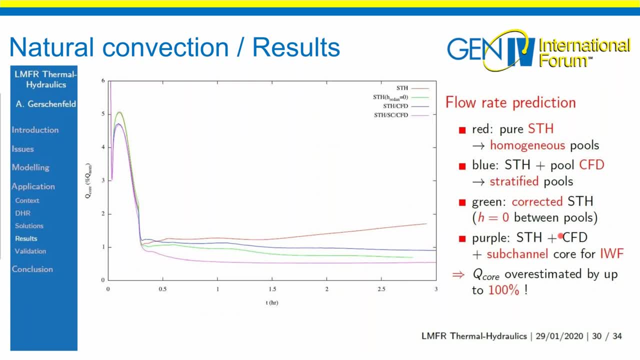 So this is the prediction, The predicted flow rate, in a number of simulations corresponding to this case. If you do an initial system scale computation, you will have a flow prediction like this. It goes down to around 1% of the initial flow rate, the nominal one. 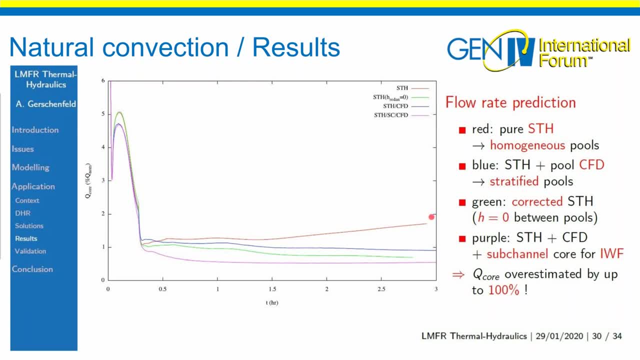 And then at some point it rises up and goes around to around 2% of the nominal flow rate And then, starting from this system scale approach, We did our first CFD coupled simulation with CFD and we obtain the blue curve. 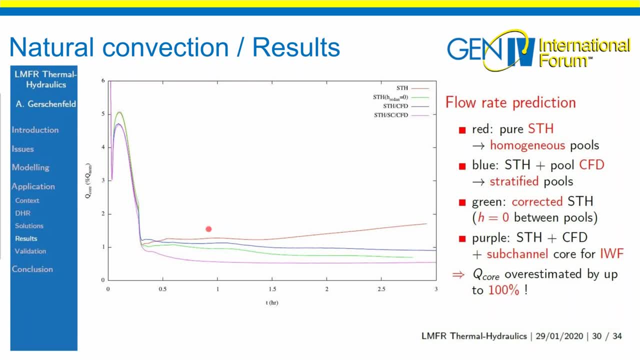 So that was a bit worrisome, because the first coupled simulation predicts a lower flow rate, and it's almost minus 30, 40% at the end of the transit, And so this meant that if you only had the system scale, you would have problems predicting the actual flow rate in a conservative way. 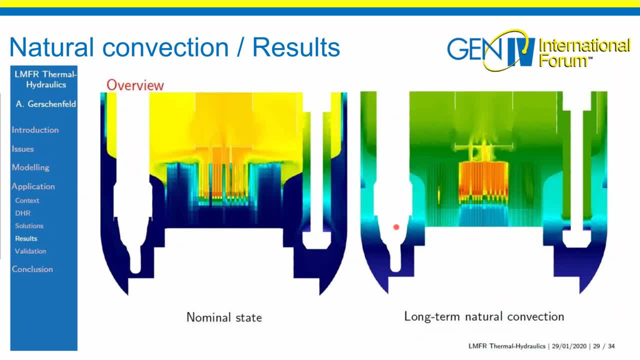 One thing you can do is that, if you read, the main source of this overestimation is that in the system scale, You have usually a formal exchange computed between the hot pool and the cold pool. This heat exchange is computed with the average temperatures. 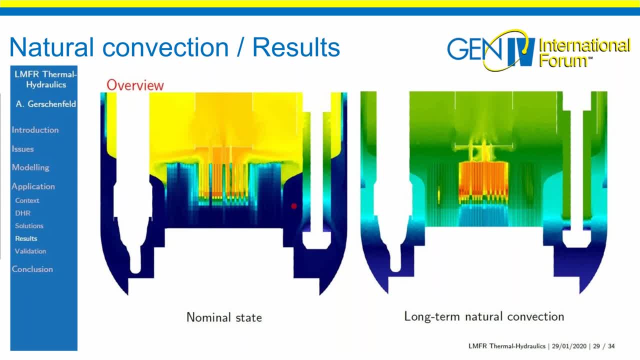 So you will have a heat exchange coefficient times the difference between this average and this average In nominal state. this is a very good approximation because this and this are homogeneous In natural convection. If you take the average of this temperature Minus the average of this temperature, it will be very far from the actual reality. 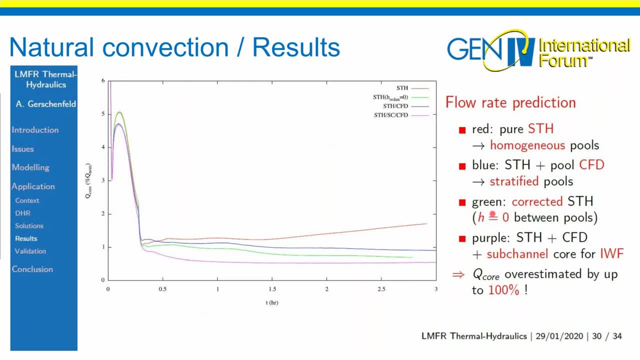 And if you're at the system scale, one thing you can do is that you can say: okay, I won't be able to compute this correctly, So I'm going to remove this coefficient and produce a conservative estimate, And this is the green curve. 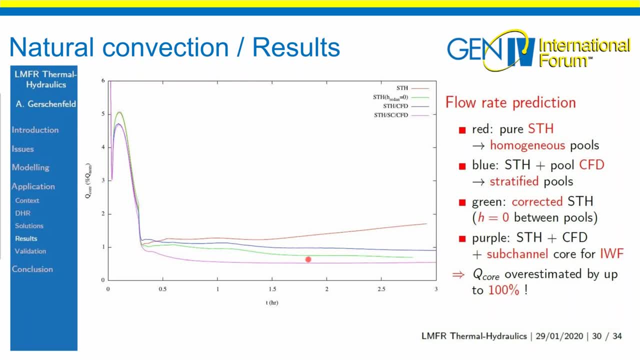 So the green curve is system scale only again, but with the conservative hypothesis, And you can say: okay, I'm back in business again because now I've got a conservative estimate. So this is a conservative prediction of the flow rate compared to the first copper calculation. 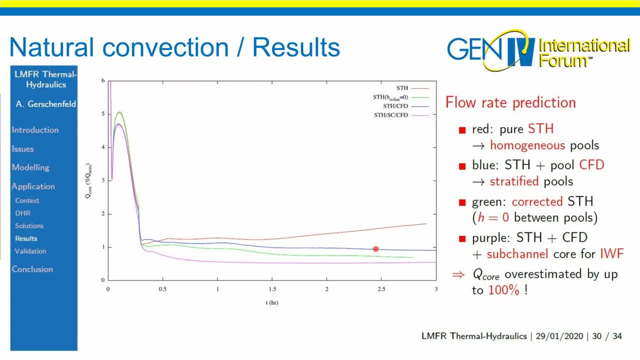 And then the next step is: how about when you do a simulation where you have system scale and CFD in the pools And the sub-channel scale between the sub-assemblies In this case? So this is what you need to do to predict interoperable flow. 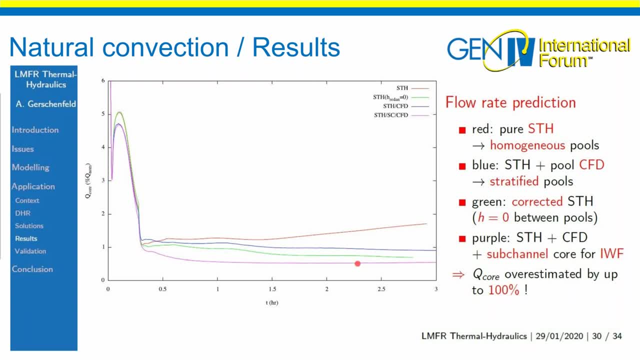 And you end up with the purple curve, And the purple curve is even lower, And then the most conservative system, scale calculation- we can make. So this means that in this case it's very hard to get a conservative prediction of the flow rate without an advanced approach that can model local effects. 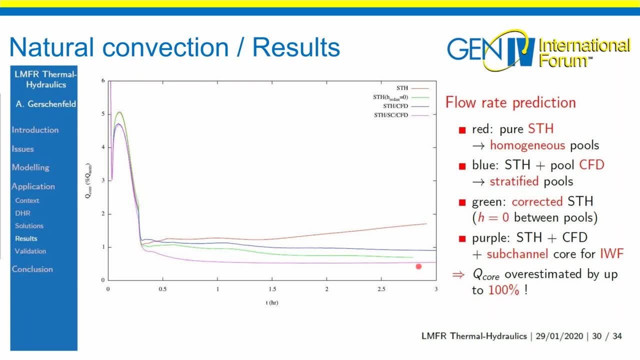 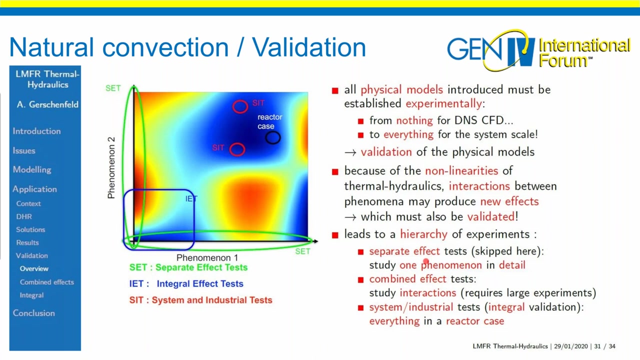 If you compare the initial prediction here to the final one with the coupled simulation here, the difference is more than 100%. So actually for the design we had at the time at CEA, we really needed to have these advanced simulation tools With sub-channel and CFD in order to get the correct prediction of our flow rate. 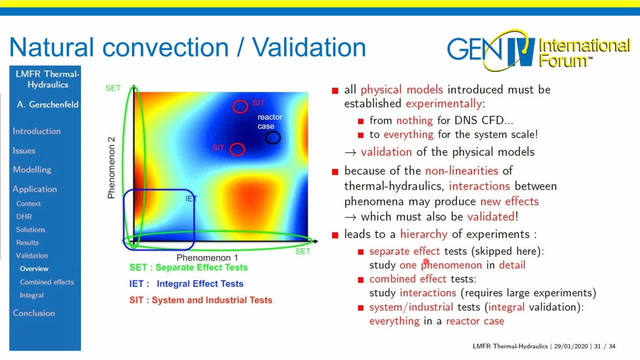 So then of course you've got. the next issue is that once you've done your simulation, you will have introduced a lot of physical models. So, for instance, in CFD you could have turbulence models In the system scale, you could have friction and interest for models, and so on. 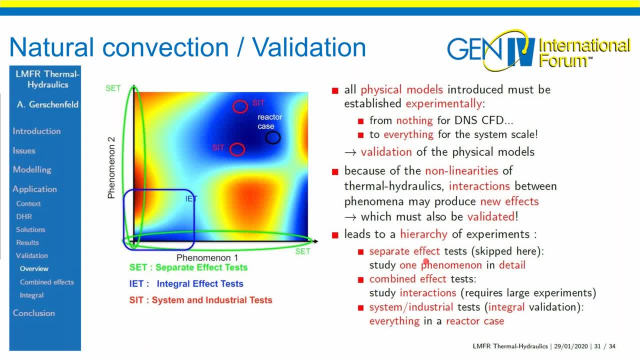 And all these models must be established From experiments. If you have a DNS CFD, you do not need anything, And if you have a system scale simulation, you need a model for every physical phenomenon, And this is what we call validation. 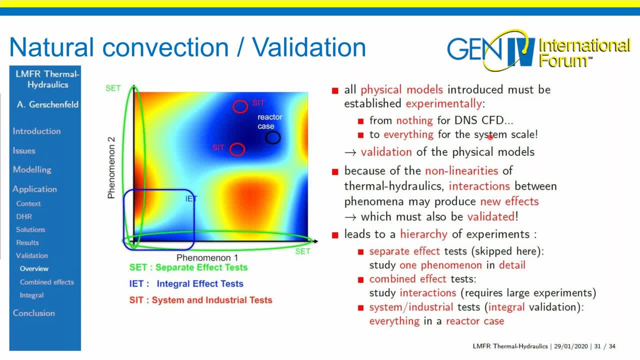 But because thermal hydraulics is non-linear. one potential thing is that if you have, for instance, a phenomenon like this one- And it's a local phenomenon, like heat transfer in a sub-assembly, And you validate it using a local experiment, 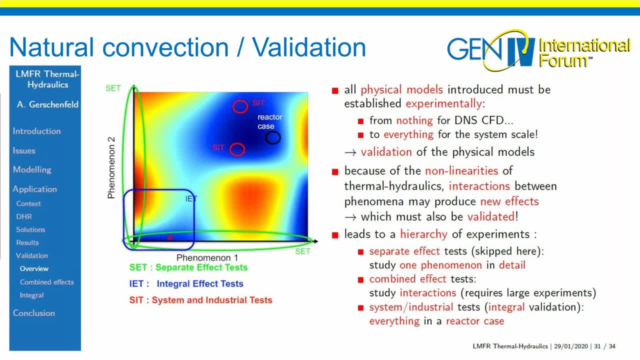 On this whole range of parameters, The same as in the reactor. When you combine it with another phenomenon, you could have interactions between them and new effects, And in this case, what you need to do is that you need to not only have experiments over the whole range of parameters from one phenomenon. 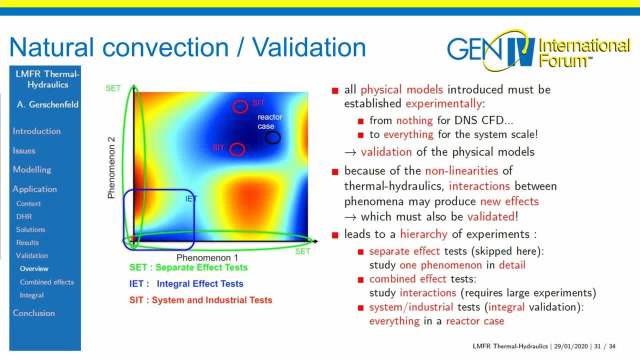 But you also need experiments that combine these parameters to have some idea of this behavior. But because of course you cannot do something as big as the reactor Before you do the reactor, you will have a size limit on this experiment. You will not be able to go all the way to reactor scale. 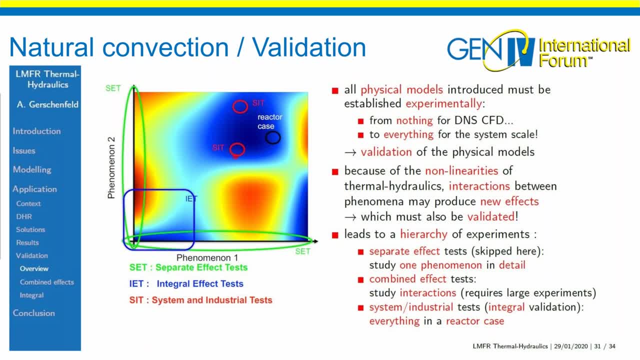 And you also need what we call system or industrial test, Integral validation Tests that are done on existing reactors, that you predict with the modeling tool of choice And you check that you are consistent with what was actually measured, And then you will actually try to predict your own reactor case right here. 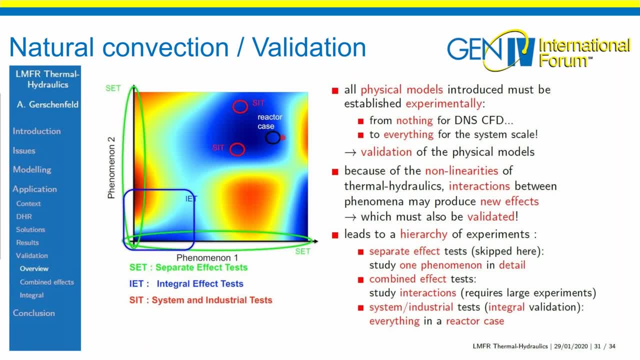 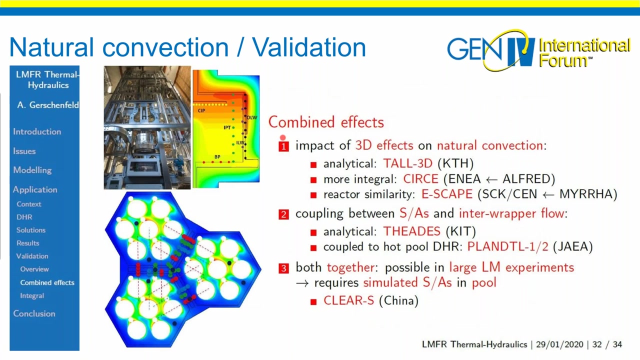 So this is what we call the hierarchy of experiments. You've got separate effect experiments- One phenomenon, but in detail Combined effect experiments, Several separate phenomena all together inside the large experiment, And then integral validation reactor cases. So if we look at some examples of experiments, 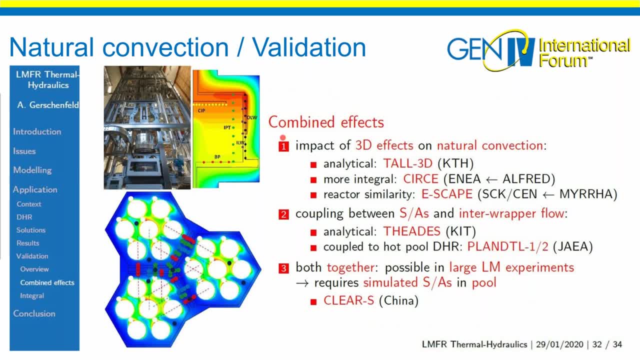 You need when you want to model this natural convection issue. The first thing that you need to model is natural convection And its interaction with 3D effects in different parts of the reactor, And for this there is a range of lead and sodium experiments. 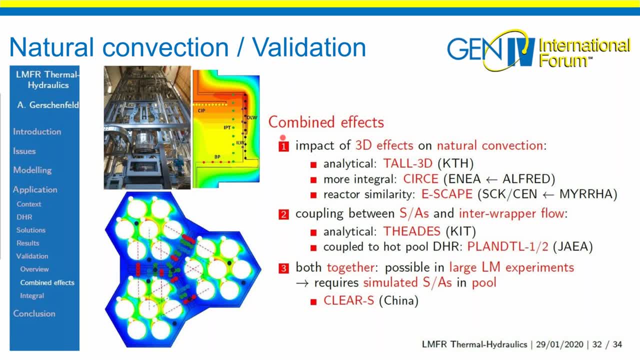 Especially, a lot of them have been performed in European projects with names like fins or sesame, And so, for instance, at KTH in Sweden, You have an experiment where you have a loop in lead-based meteorotactic And in the middle there is what they call a 3D section. 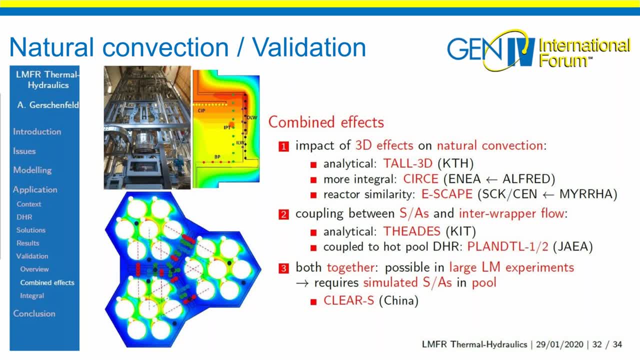 A little cylinder of hot lead And this cylinder will stratify like this And there may be a jet at the bottom that can either go all the way to the top or get stuck on this stratification. And this is something you can use to model to check if you are modeling correctly the interaction between 3D effects and overall natural circulation. 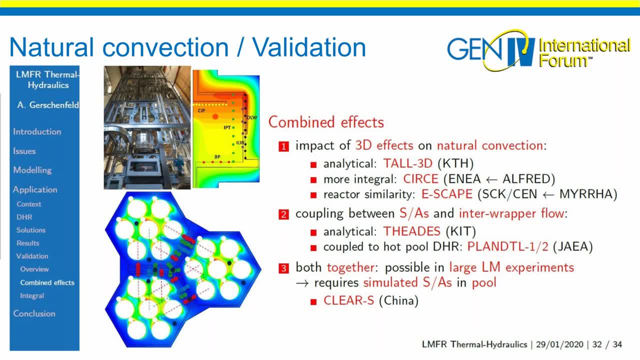 At ENEA in Italy, there is an integral experiment called CHIRCHE on the same issue, And there is a scaled-down experiment of the MIRA reactor project called ESCAPE, being done at STKCEA in Belgium. There is also the issue of the thermo-hydraulic coupling between the inside of each of the assembly and the interoperable flow. 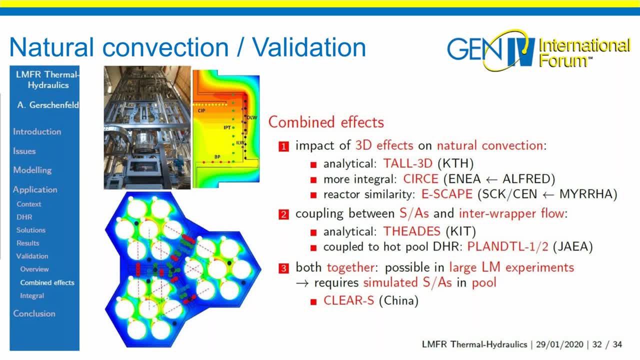 And for this one you can do some small scale analysis. You can do some analytical experiments like this one in KIT in Germany where they had three sub-assemblies with seven pins each, A model, the thermo-hydraulic transfer with the interoperable flow in the middle and a lot of thermocouples to check that the codes can predict it correctly. 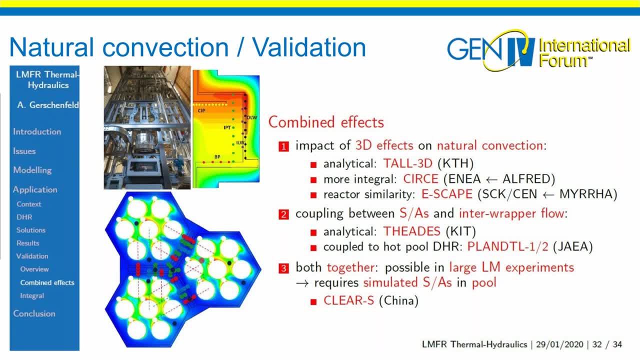 And then, at a larger scale, you have Japanese experiments, PLANTEL and GIEA, which can model both the core itself with as much as 55 sub-assemblies And it's coupling to the overall hot pool, And these experiments are actually of very high importance to show how much heat interoperable flow can remove from the core to the hot pool and then to the decay heat exchangers. 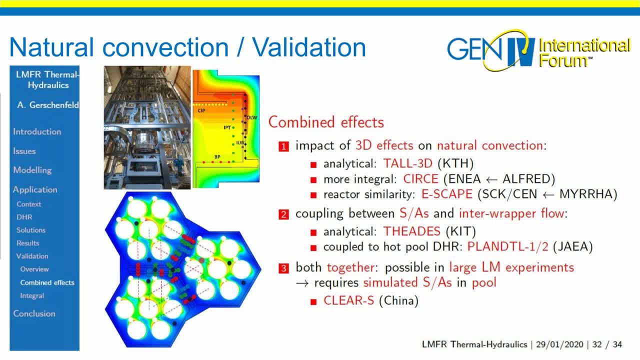 And finally, there is a possibility that in the near future, we could have a large experiment where you have both the core, with interoperable flow, and the rest of the pool, And this is something that, for instance, could be used in the future. 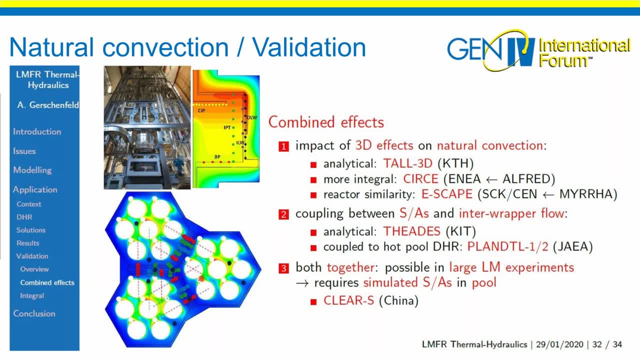 And this is something that, for instance, could be used in the future, So these experiments could be experimented on the ClearRES facility for a lead-Bismuth pass reactor in China. And then, going at the larger scale, we have integral tests. 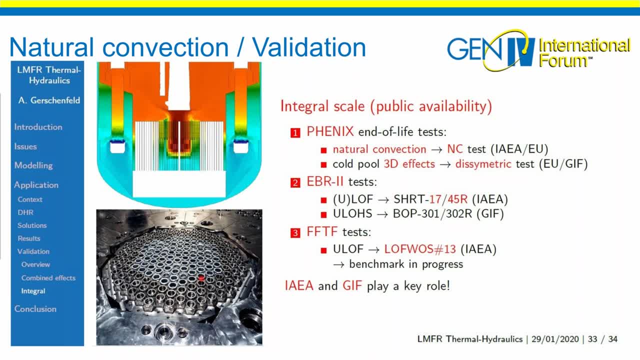 And so for this one here I've put a list of interesting liquid metal tests for validating liquid metal for our LLC codes. Most of these tests, All of these tests, are on sodium pass reactors. Most of these tests are on sodium pass reactors because we've got the integral test for the Day Us and the Pneumatic Festynenum. 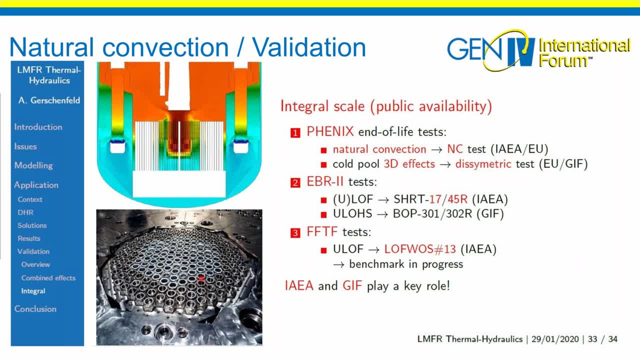 Most of these tests are on sodium pass reactors because we've got the integral test for the Day, Us and the Pneumatic Festynenum, the, the integral, the reactor scale experience of this one and, for instance, we've got tests that were performed at the end of life of the of the phoenix reactor right here, so for instance, at the 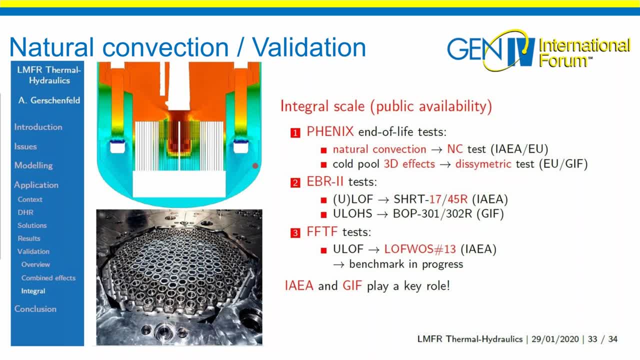 end of light, of at the end of life of phoenix in 2009, 2010, we did the natural convection tests. so first we stopped the heat sink- actually we started with what we call a loss of heat sink- and then we shut down the pumps and we did a protected loss of flow- plof- natural convection. 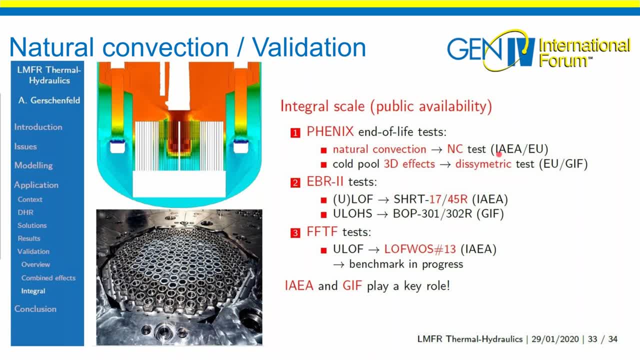 test, and this is something on which we did both. we did public benchmarks in the iaef, in an iae crp and in european project framework, and here you you can already see the importance of international organization in sharing this reactor scale data. more recently, we also shared data on a. 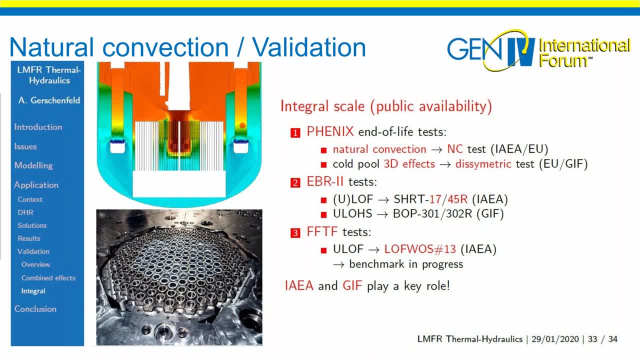 dissymmetric test, a test where we shut off one of these two intermediate loops and not the other, and then- and this allowed us to measure 3d effect in the cold pool, and we shared data on this test for a new eu benchmark in the in the sesame project and it is currently being shared in the jeep sfr safety. 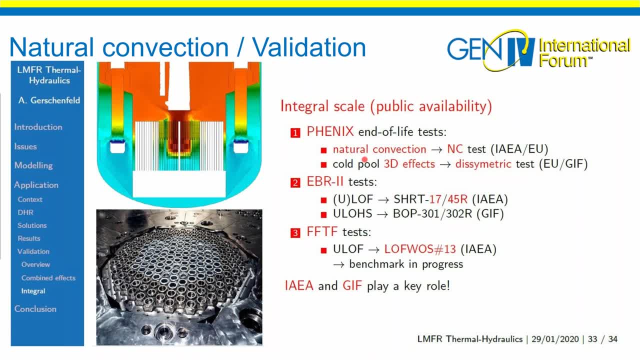 and operation working. so i think this is a really big incentive to join this sfr as a new working group. and then we've got tests on ebr2, so from from the ue. so in the past there was an iaes crp on two- loss of protest, so natural convection 17, which was protected, loss of flow, and 45- air, which was 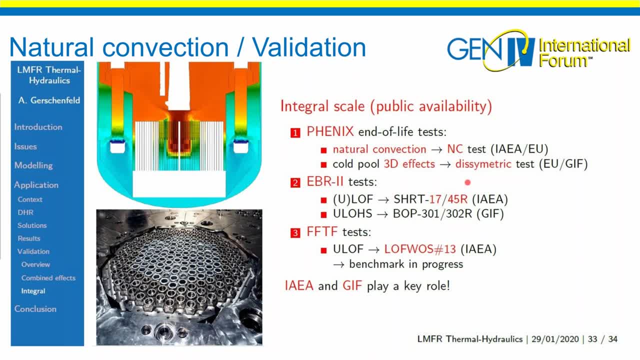 which was unprotected. so today, two public tests for my through iaea, and then more recently doe has proposed two loss of heatsink tests. so the pumps keep operating but the heating is is lost in the same gif, sfr safety and operation framework, so these ones are. 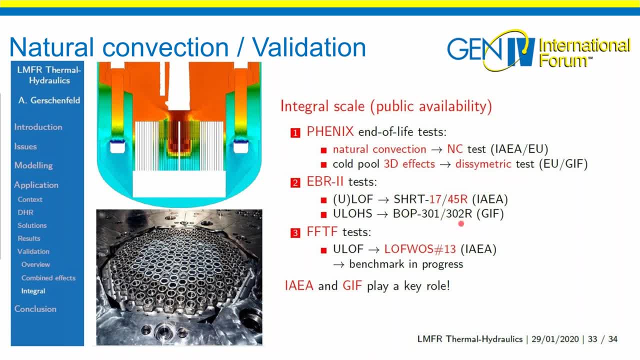 called bob 301 and 302r. and finally, so since the, since the- let's see- september 20 2018, we have had the uh benchmark on the fft loop type sodium paste reactor at the oe as well, and this was a non-protected loss of flow test cause called the lakwas, and this one is actually in progress. and 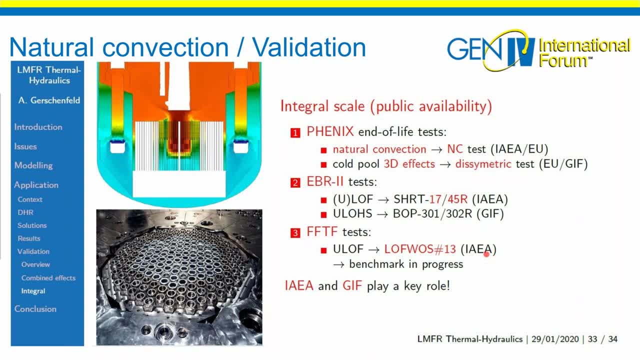 this is an iaes crp and the first, the first meeting, with the presentation of the blind results and so on, will be next april, actually, and this is an ongoing benchmark. so, as you can see, if you want to, to obtain integral validation, check and share reactor data, iaea and the gif play a. 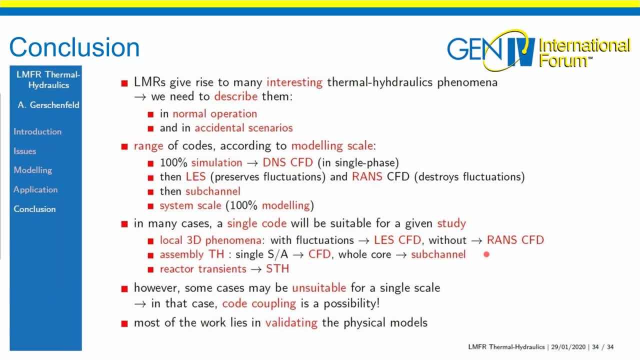 very important role and so moving and so moving on from this application to natural convection, i i've got a little conclusion right here. so the first one is that in liquid metal reactors, as i showed you, there are a lot of interesting from from my hydraulic phenomena and we need to. 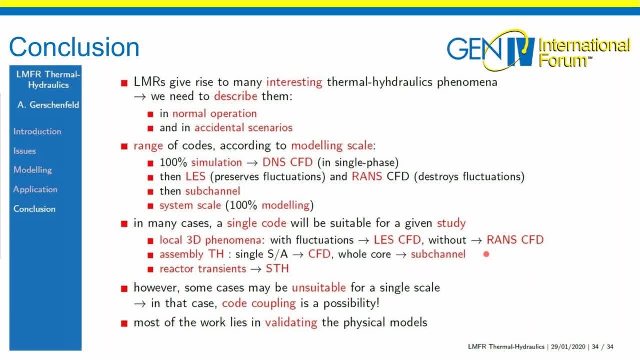 describe them. so some are related to normal operations, some are operated, are related to accidental scenarios, but we we usually end up needing to model them and in order to do that, we have developed a range of codes with different modeling scales. so we've got cfd- computational- 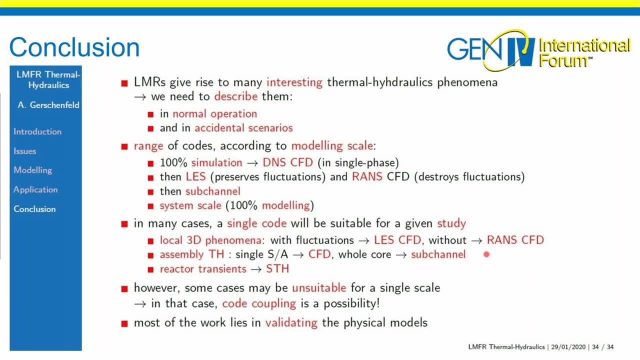 fluid dynamics, both dns, direct numerical simulation, where you simulate everything and you need no physical models, although then to les some fluctuations and then runs. all turbulent fluctuations are modeled with a, with a physical model. then the sub channel scale, a bit coarser, and finally the system scale, where you need physical models for everything. 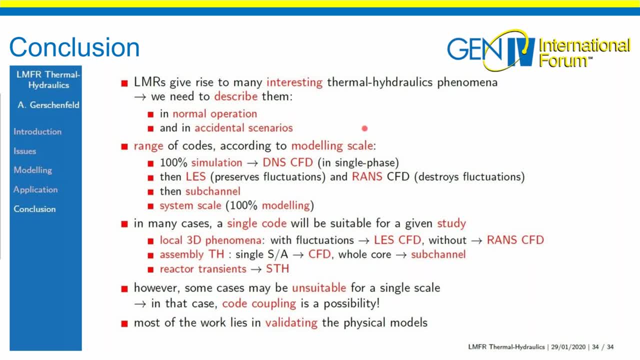 so, for example, in some cases, given a problem of choice, one of the one of the scales here will be what you need. so, for instance, for local phenomena, if you have, if you need to account for fluctuations, you need to use les. if you don't care about fluctuations, runs will be all you need if you. 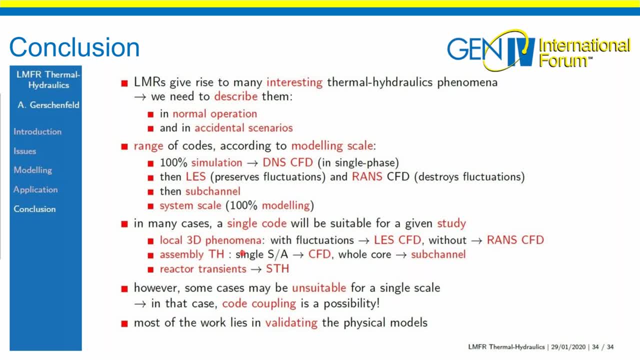 need a subassembly from hydraulics at the level of a second sub-assembly and locally you can use cfd. if you need to do it over the whole core, then the sub-channel scale will be a bit coarser and then a be the one of interest, and if you want to model reactor transient you will need the system scale. 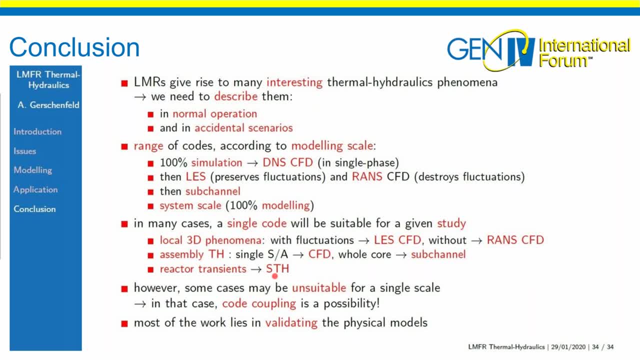 the courses one, and in some cases this may not be enough and you may need, and you may need to do something more complicated, for instance coupling between different codes, and in all cases, a lot of the work, and actually the majority of the work, will be actually in the, in the an. 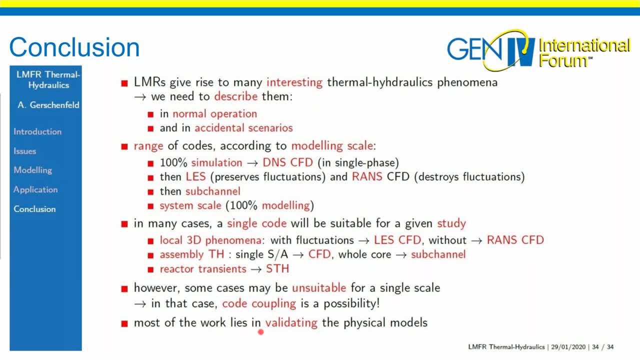 aspect that we don't think about at the beginning. it's in it's the experimental validation of all these physical models, and for this we need experimental data at small scales all the way to a real, actual reactor. and this is where international collaboration is extremely important. and that's all from me. thank you from you for your attention. 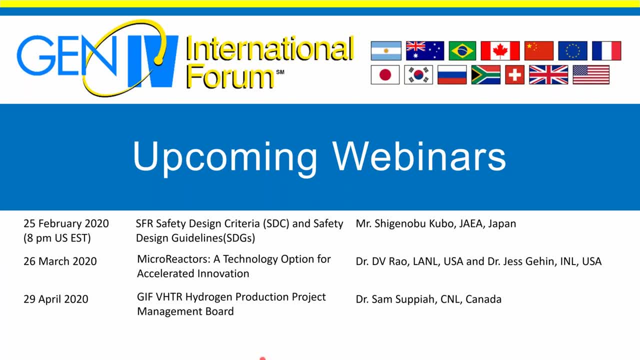 thank you. thank you, antoine, very much for your presentation. um there have been several questions posed. we'll give people just another second to type in questions that they may have. um that you're following your conclusion and in that time we'll just take a peek at the upcoming webinar presentations. um in february there's a presentation. 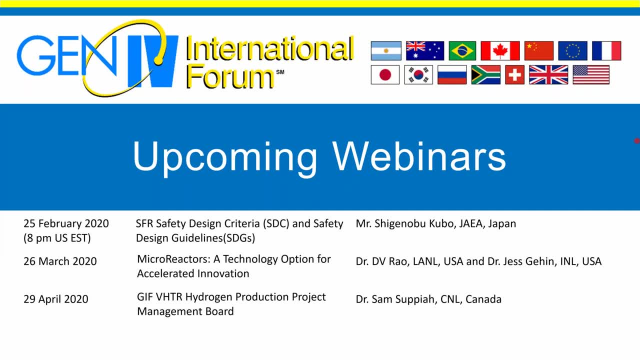 on sfr safety design criteria and safety design guidelines. i'd like to draw your attention to the shift in time scheduling for that presentation, rather than in the morning, us eastern standard time, we're going to shift that to 8 pm us eastern standard. 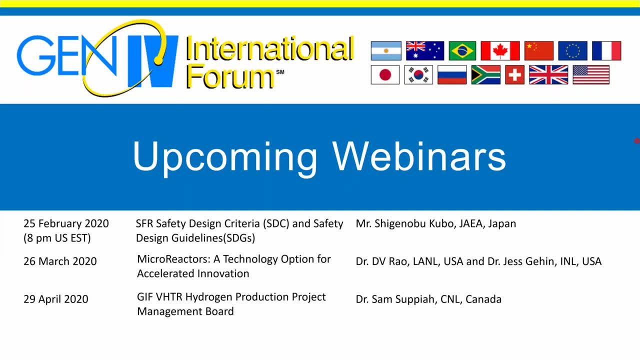 time to more um align better with the japanese presenter. in march we have a presentation on micro reactors, a technology option for accelerated innovation, and in april the gift vhtr hydrogen production project management board, and they will be able to provide you with a link in the chat box. 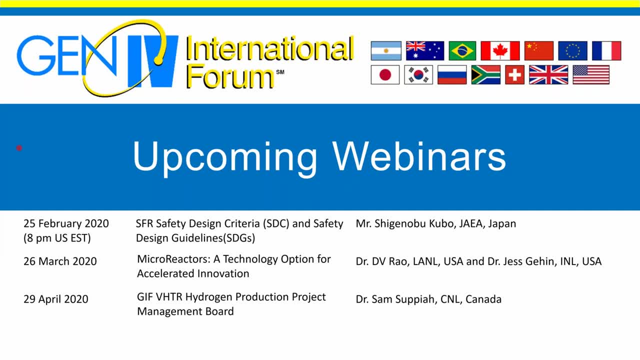 that will give you a little bit of information about what they're doing in order to make sure that they're, uh, making the right decisions, and how they're going to use that information and how they're going to use that, and i'll be able to answer those questions in a few minutes. so i'll see you in a couple minutes. 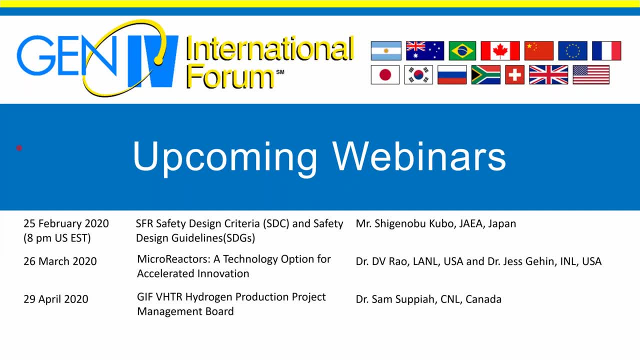 thank you a lot. thank you very much. so the first question on the list is: shouldn't the lmr reactor group include solid fueled but clean molten salt cooled reactors as well? it's just another high-tech question, another high temperature, low pressure coolant. So of course molten salt is a very interesting 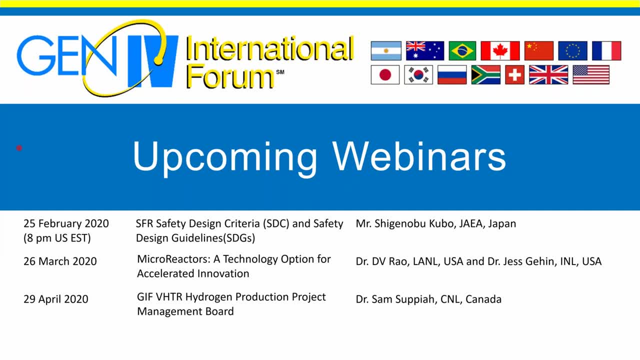 option and actually even in even in CA in France. so, as you may know, our big sodium fast reactor project, Astrid, came to a stop at the end of last year and since the beginning of this year, we have started to look into molten salt as well, mainly as a as a as a liquid fuel. so 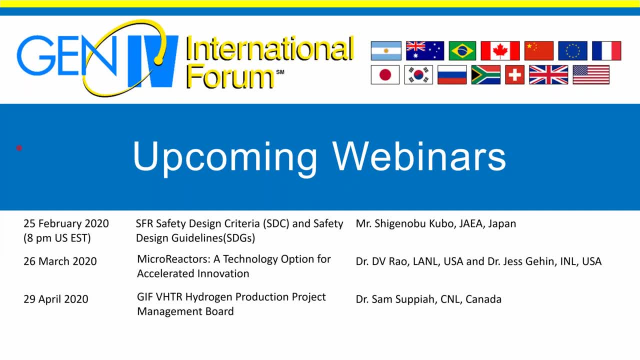 with the, with the fuel inside the coolant, and there is also the option of having solid fuel but molten salt as a liquid and in this case the. the main issue will be both for the material problem like corrosion- corrosion and the radiation and things like that- and the, the main advantage of 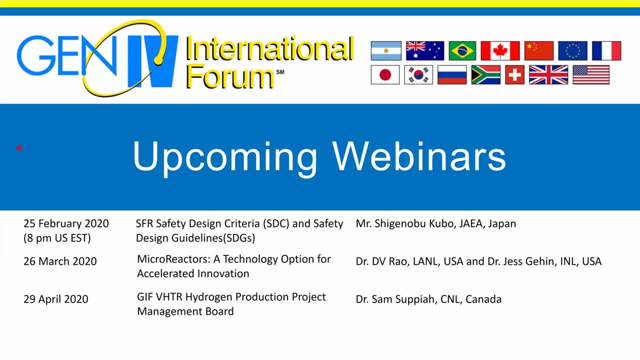 liquid metal, in this case, for sodium for instance, there is almost no corrosion issue if you control for oxygen content. so you can use standard stainless steel and be convinced that these materials will last the lifetime of your reactor. and of course, if you, if we, if we do the material R&D, we may find. 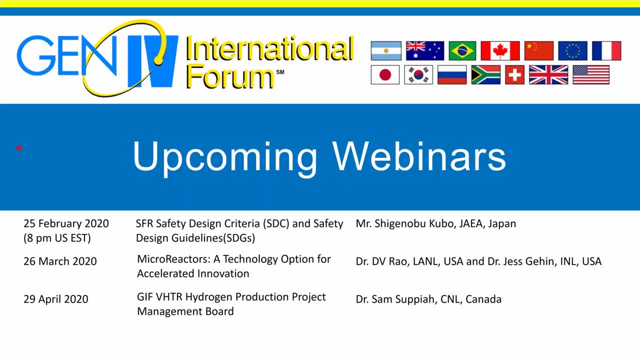 a material that does the same thing for molten salt. but if you, if you, ask me to design a high temperature molten salt reactor right now, I would have big issues with the material, but it's a very good choice. but this may change in the near to medium future, and this is something 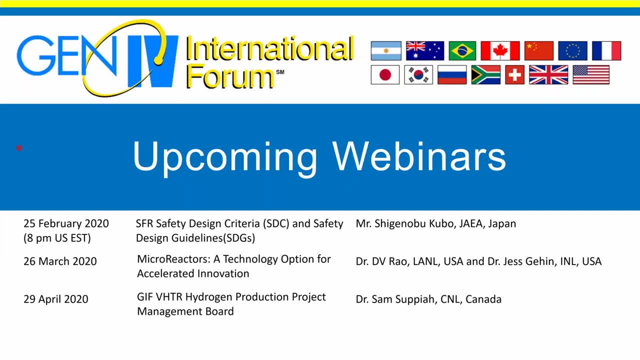 that I agree should be looked into for lead it's. it's more or less the same you, you. there is. there are a few more issues with corrosion of corrosion of thinning lead. you need some oxygen content in order to to have an oxide layer on the steel to prevent lead from somewhat corroding it. 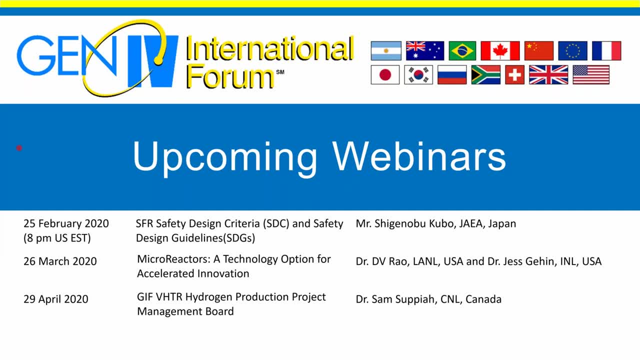 but still it's a way easier materials problem than molten. so for me. so I think, as, as an option we need, we need to keep investigating the two liquid metal reactor concepts, because these ones, more or less we we know how to make them, without consider even, for instance, we we know the choice of material, with all the issues and so on. but if, if, 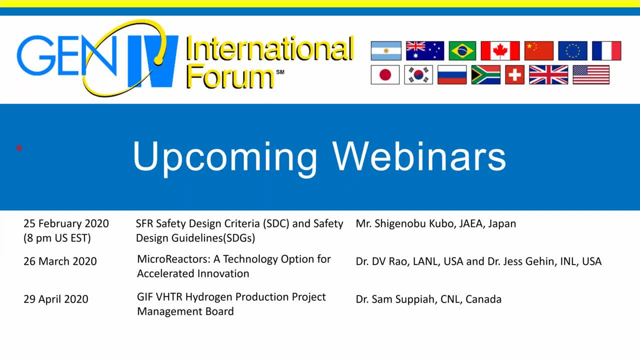 we're considering a project for a bit of a longer term, then everything is interesting, of course. great, thank you. the next question: please describe the function of the core catcher and flow patterns when the core catcher is catching the melted core. so so this is something that we included in the street project and we we also see in a few sodium. 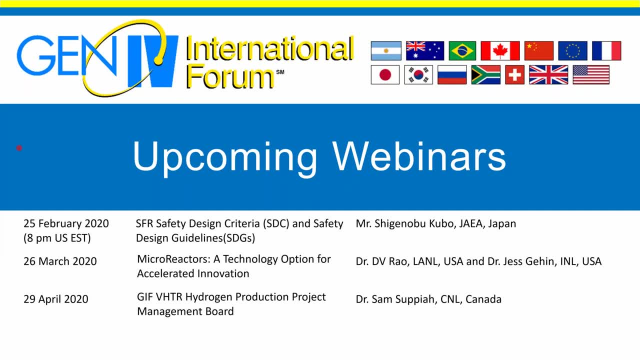 fast reactor design. so, of course, if you have a severe accident in the in a sodium fast reactor, in this case you so what the fuel is is going to melt in the core and at some point it comes down right. so so both, for instance, going into the console, water assemblies and all the way- 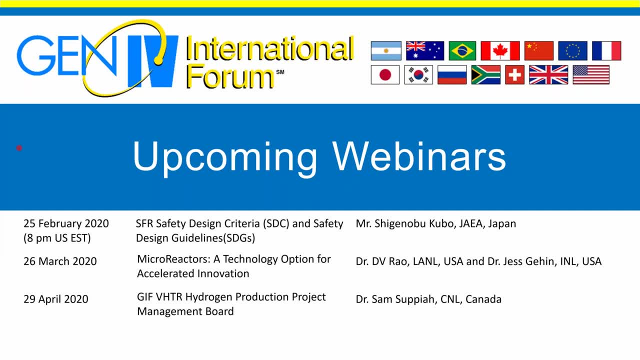 down and of course, you've got the. you've got the main vessel at the bottom, and so you you can choose two things: either to keep the corium inside the primary vessel at all costs, or you let the. you let the corium go down to the main vessel, cause a leak and catch the corium below. so in a street, our 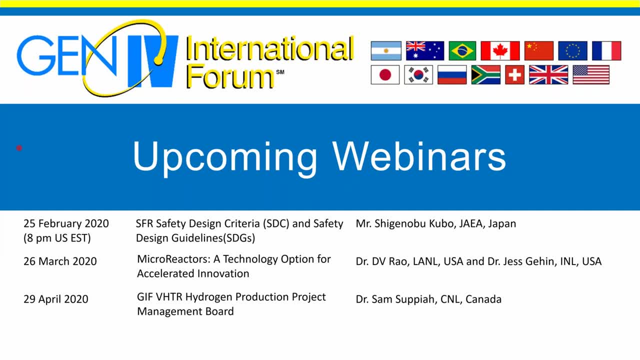 choice was to say that we will coach the core careful test of our system. so in a street, our choice was to say that we will coach, we will catch all the corium inside the main vessel all the time, and the advantage with that is that there will not be a leak and once the the corium is on, this core capture. so the thing that 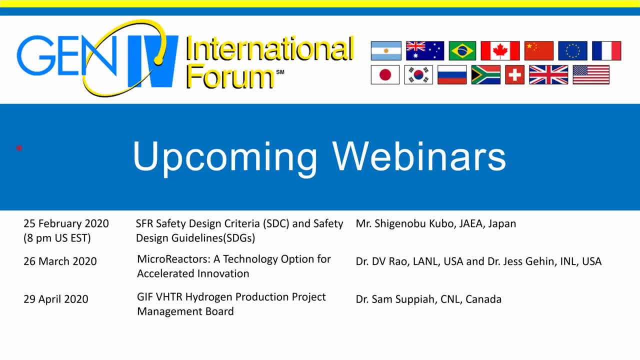 will catch the, the corium going down and stop it. finally, then it we will be in a position where we can cool it more easily because we will be in, we will be in sodium. we can use one of the decay one of these decay heat exchangers to remove it from the top of the pool and there will be. 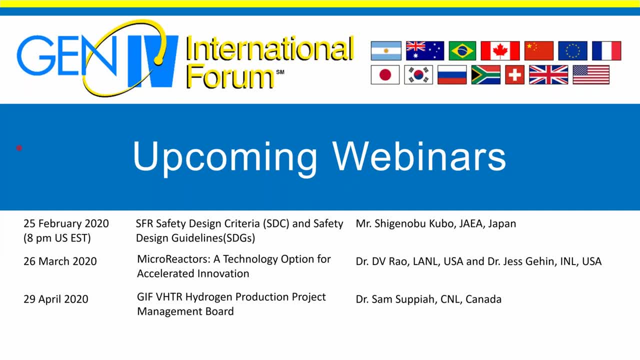 natural convection flow from the core capture at the bottom to the heat exchanger at the top. and, of course, the big question we had was: what material? what material can we include for this cold capture? and we were considering, we were considering things like zirconia or other. 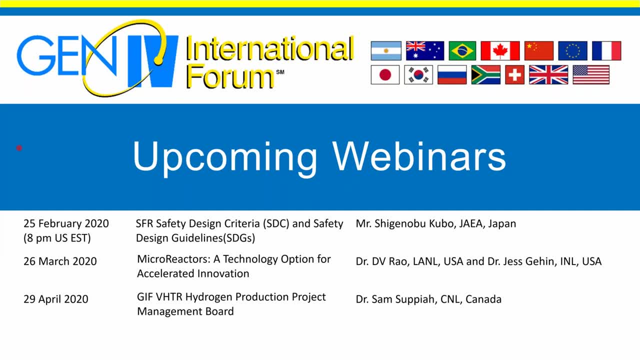 materials like that, and the big issue is that: can you find the material that will both be able to catch and dissipate the corium and will also last for the 60 years of lifetime of the reactor? so will it work if there is a core disruption accident? 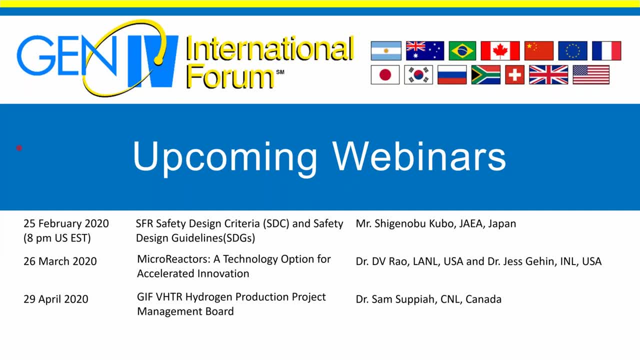 and if we don't need to use it, can we at least check that it will be there, for it will not cause problem during the 60-year lifetime of the reactor. so the function of the core catcher is that, if corium manages to come down from the core, we need to have a material that. 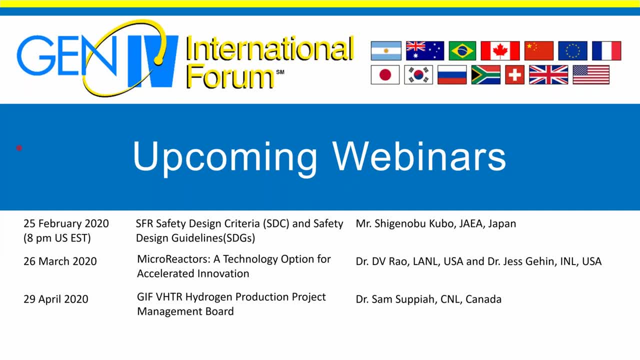 cannot. that will not be ablated by the core. so usually your ceramics or zirconia, ㅎㅎ, thank you. there's a question about the ihx design, specifically why the aspect ratio of ihx is so high. if more heat transfer tubes are used, the height of the ihx can be reduced. is there any restriction? 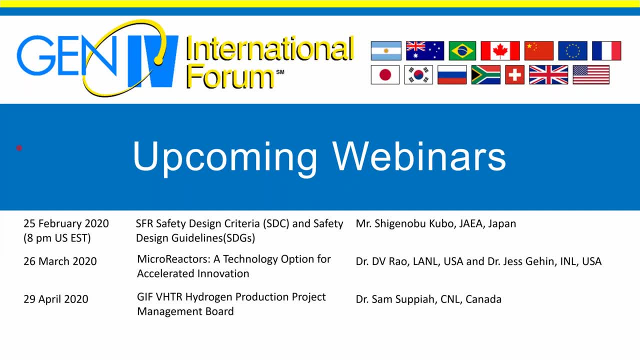 about the ihx design regarding to its height or aspect ratio. so so this is actually something that we did in the in the asprey project reduce report, so in the in the french sfr designed, and i think this is also valid for the russian sfr. 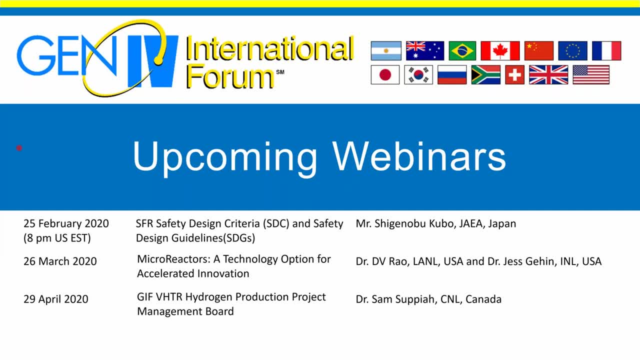 designs. we have the core in the middle and then we have the heat exchangers and the pumps on the outside, and so if we want to have the smallest vessel we can, we need to. we need to make our heat or heat exchangers as small as possible in the horizontal direction. and because we are trying, 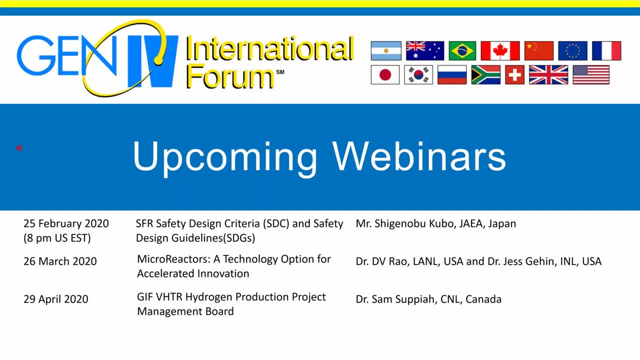 to make them thinner if we want the same heat transfer. we we tended to make them longer, and so they end up going all the way down, as you can see in the picture, and this is actually something that, um, this is related to our complicated flow behavior in natural convection. it's because our 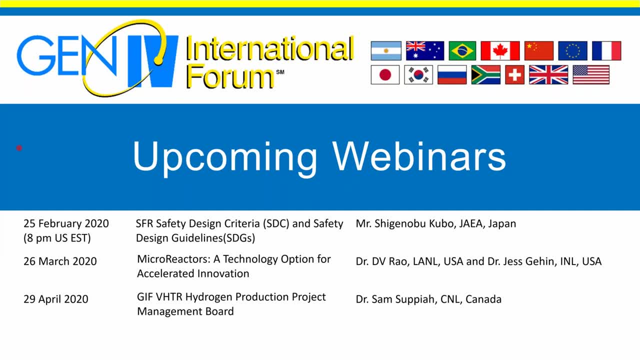 heat exchangers are so long that we have low natural convection flow rate. as you can see, on one of the sides it's slower than the that it would be if the heat exchanger was short and at the top of the reactor. nevertheless, it's- uh, it's a thing you can do if you want to obtain. 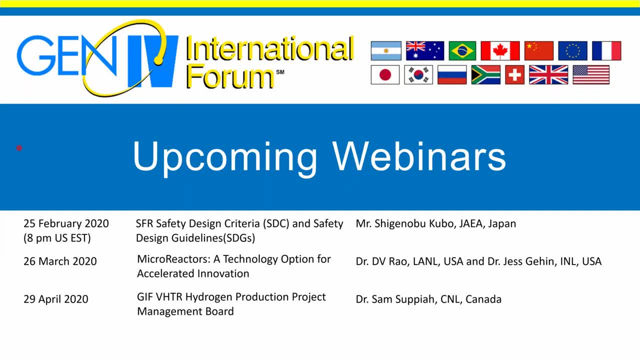 more heat and then you can optimize your reactor design as much as possible and you can. even with long heat exchangers like this, you can still have good overall core cooling if you, if you model all the possible decay heat removal paths between the core and the final heating. 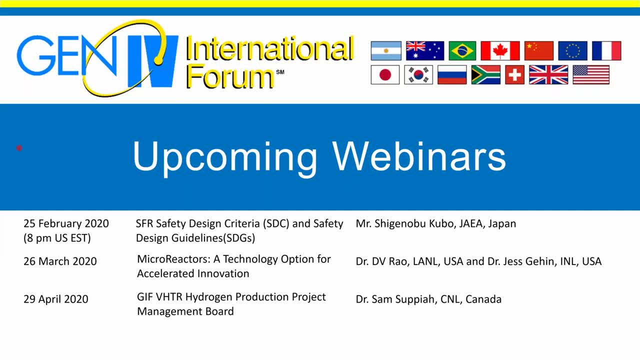 thank you. gilet has also had a question about extending the code use to molten salt reactors and i'm not sure, but i believe you've answered the question. so if you want to get more information about that, please back question. do you have any more thoughts on that? so, normally, if you go. 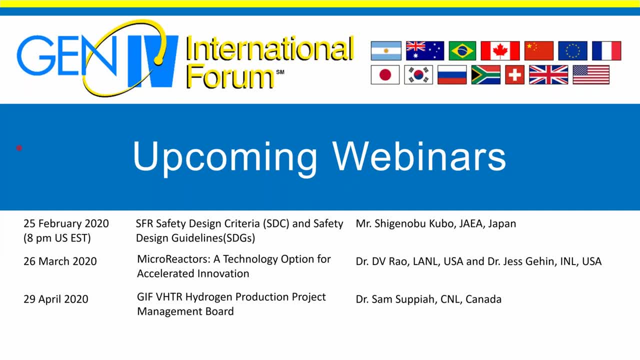 from liquid metal to molten source from the. from a very point of view, the big difference will be the heat transfer modeling in, for instance, CFD code or system codes. so in liquid metals we have, usually they have a very high thermal conductivity and so you you are in the case where the turbulence as an effect 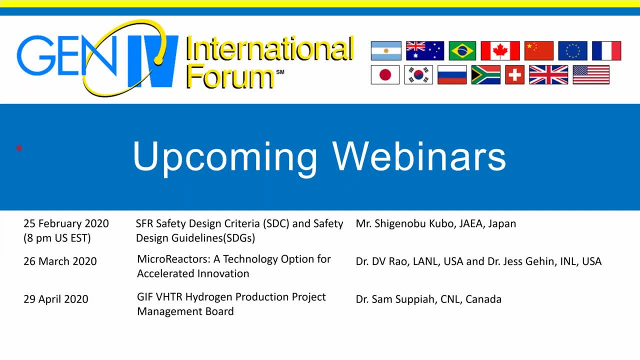 on momentum but does not affect the heat transfer itself very much, because the heat transfer is being done by the very high thermal conductivity and in molten salt. on the other end, you have a very low thermal conductivity, actually lower than water, for instance, and so you need- we need- different turbulence models for 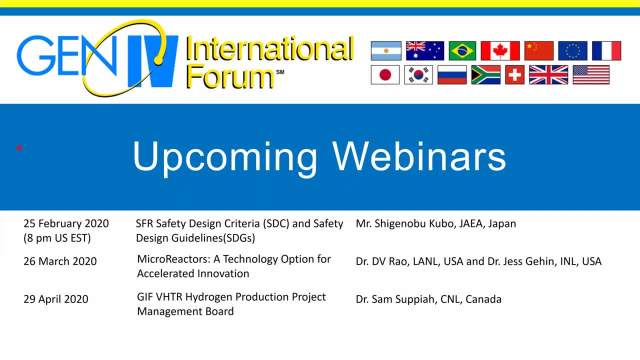 instance, who correctly predict the behavior in the molten salt reactor? another thing that needs to be done is that if you have, if you have liquid fuel- and you know you will have this- the delay neutron precursors, so the, the sorry, the delay neutron emitters. so 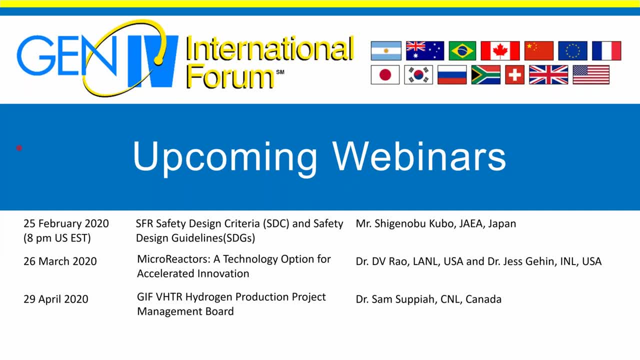 the radioactive elements that in that emit the delay neutron fraction, will be moved around by the fluid, and so we, in this case we really need both to predict where they are going, with the, with the thermal hydraulics, so with the CFD code, and we need to couple it with 3d neutronics to get the actual power distribution in the. 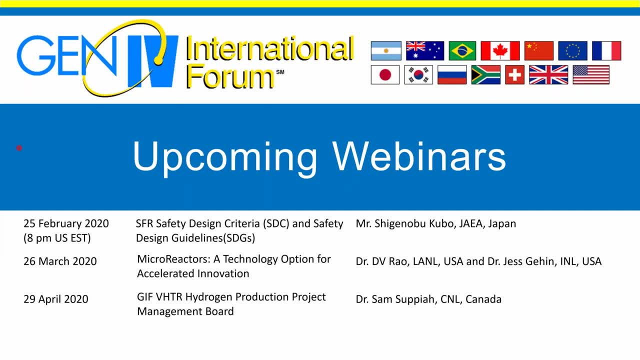 core. even so, currently for molten salt, we have tools, were working on the coupling between our CFD code and a 3d deterministic neutronics code in order to be able to correct the model and open such reactor, for instance. thank you, do you let is on with the university mathematics departments, for example, the 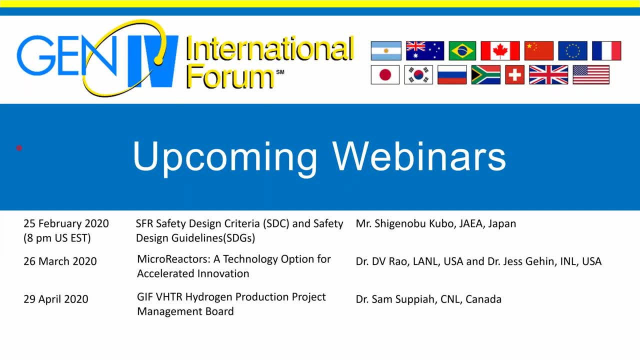 application of group 30 and geometrical mathematics department, for example, studying quantum physics, research in mathematics, the application of group 30 and geometrical methods to the solution of differential and difference equations. the emphasis combination of analytical and numerical methods and also the use of symbolic. 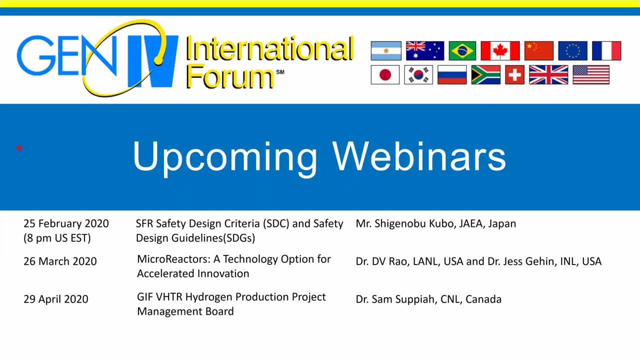 computation. So on this part, there are a range actually of computational methods that have been tried in each of the scales of modeling we have. So, for instance, one of the system codes, so the one with 0D and 1D models, the German version of this, they use direct methods of. 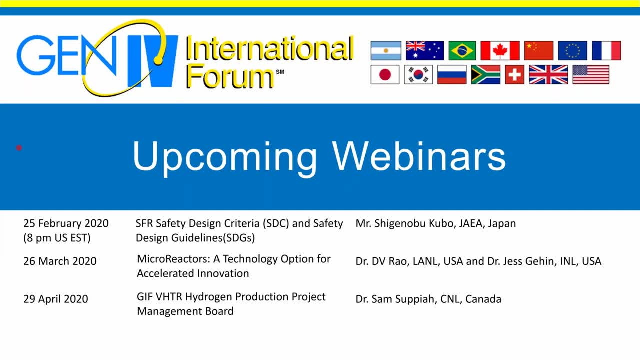 characteristics to solve their differential equation. Usually the main thing that we see used in these codes are finite volumes, because physicists have made them and so they are interested in conservation relations, and myself I've worked on the numerical scheme of this sort and for people that really want to have a very 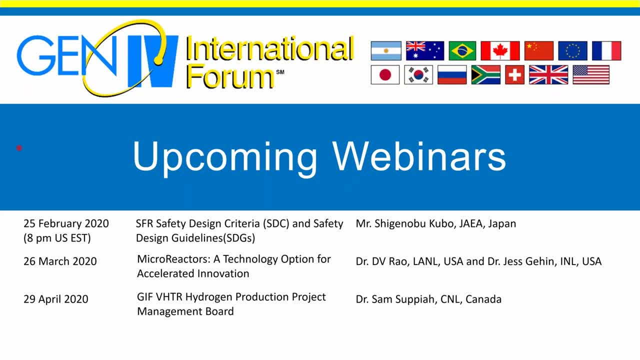 good conversions rate on their differential equations, mainly for the DNS direct numerical simulation. the DOE uses a code with spectral elements, So finite element methods where you increase the degree inside each element as you refine and so you get exponential convergence to the analytical solution. But I should say that the main thing you see is finite volume methods with first, 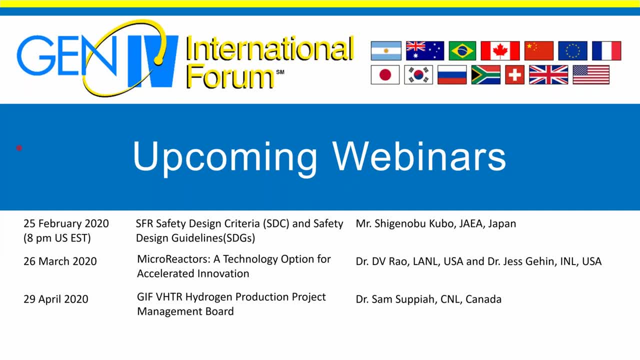 order, discretization both in time and space, and this is because usually you see physicists behind these calculations and so they're interested in some very down-to-earth conservation properties, even on the discrete solution. There's a couple similar themed questions. I'm going to go ahead and skip through Boyne a little bit. 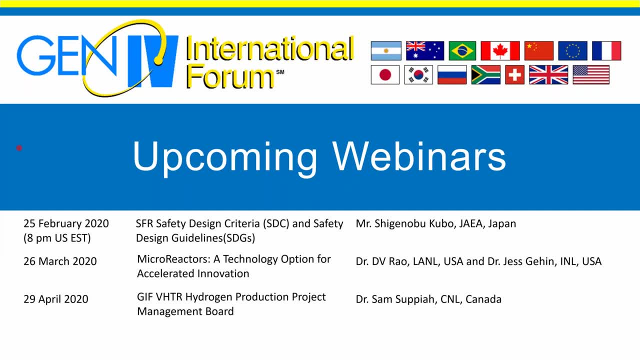 The non-dimensionalist. I apologize, Francis, So I'm going to start with the non-dimensionalist. So the question is: how do you know that a non-dimensional number has a very high probability? So you know, this is a very important question. 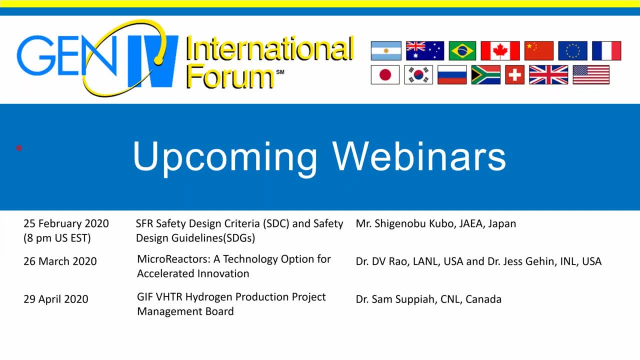 I'll just give you a little bit of a brief answer to the question, So you know if you're studying. a typical operating temperature is very low. what's the significance of this? And then there's one more on how do you explore the parameter space. Do you conduct probabilistic, such as Monte Carlo analysis? So first for the parental number. the practical consequence in sodium is that if we, for instance, look at how you could, how you can perform a CFD simulation- you know you want to be- 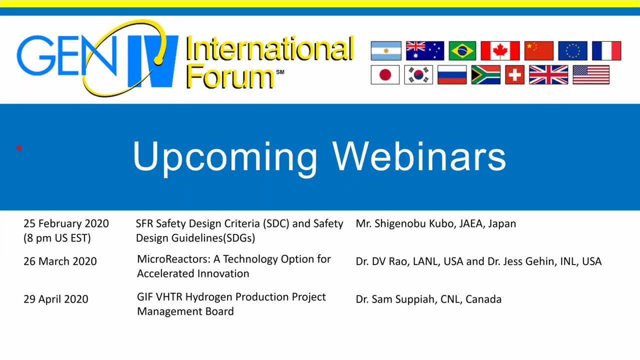 of a sodium reactor, then we will use a turbulence model for the momentum, for the velocity, but on the thermal side, because of the five, ten to the minus four quantum number, on the thermal side we can just use the naive laminar conduction rate and this actually accounts for all the conduction you need. 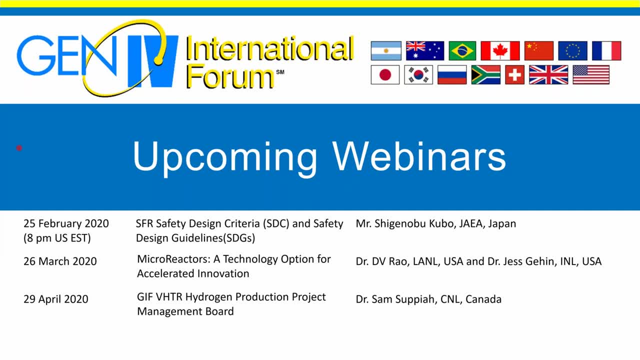 same thing at the system scale in the. so the, the non-dimensional number for format for heat transfer, is what we call the Nusselt number and it's it's around four in laminar flow and then it goes up with turbulence and in sodium you can. 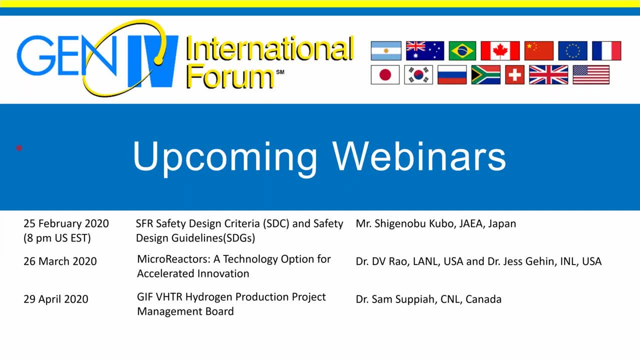 take constant Nusselt number equal to five and it will predict the whole, the whole interesting range of parameters. so in so the this very low frontal, actually in sodium, in solo, that it simplifies things a lot. you can, you can model heat transfer as if you. 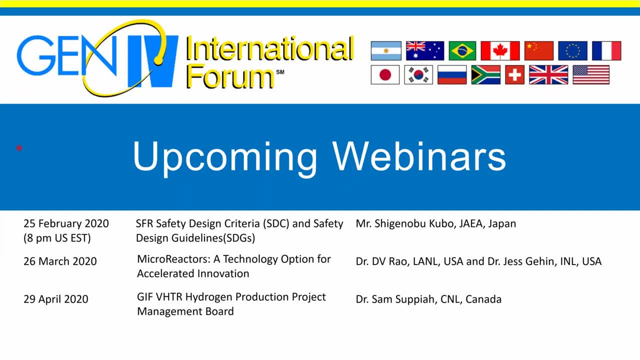 were in laminar flow, almost in lead. it's a bit less guaranteed because the frontal is a bit higher, but still you have this type of phenomena. for the second question, so for the, the non-dimensional parameter range. so in when we do validation and experiments we try to cover as much of the actual 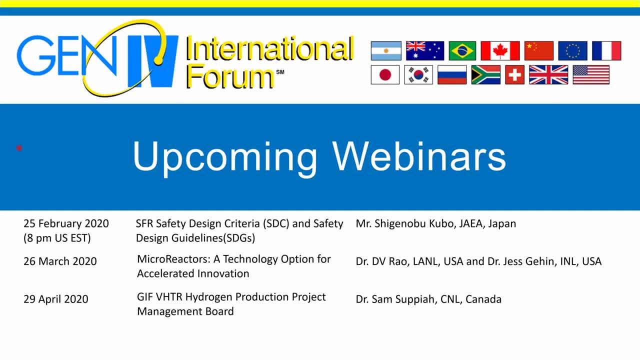 parameter range as possible, as possible when we are doing our experimental tests. and then there is an interesting point when we perform reactor simulation. so in this, in this simulations, one thing that is very common today is that we may want to do uncertainty propagation or what uncertainty analysis of our reactor. 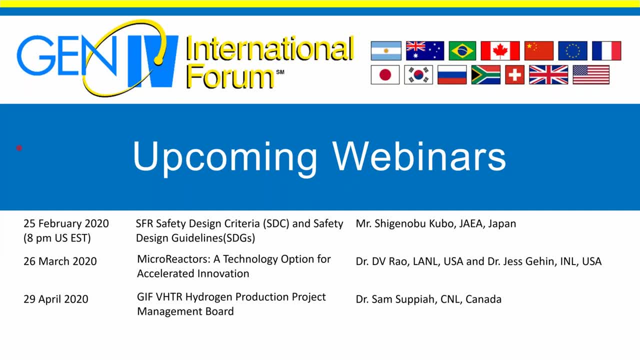 calculations, and so we will have a range of input parameters. for instance, what was the power of the reactor at the beginning? we may have some, some uncertainties on the physical models as well. so, for instance, we know the friction coefficient somewhere, but not with 100 percent accuracy. we have some, we have some uncertainty on that, and then we 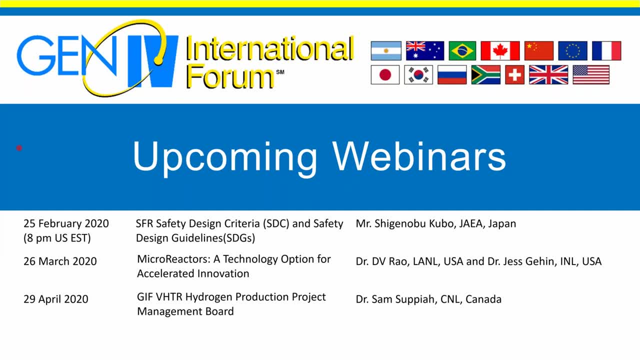 will propagate these uncertainties and assess their effect on the final output result. and this is something we do well sometimes, usually in a naive way, with what we with the Wilkes method, where you do 207 calculations and you do some statistics. but what's also really common is to use Monte Carlo. 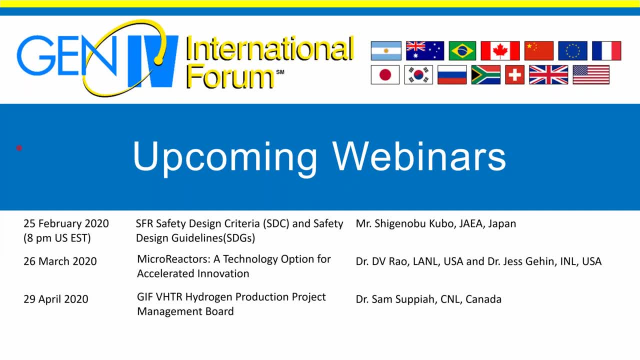 sampling of these parameters, build the metamodel of the simulation on top and then do our uncertainty analysis on the metamodel. so actually we- it's a. it's rather common to use Monte Carlo propagation at some point. thank you, how would you couple STH with CFD when there is local or temporary boiling and 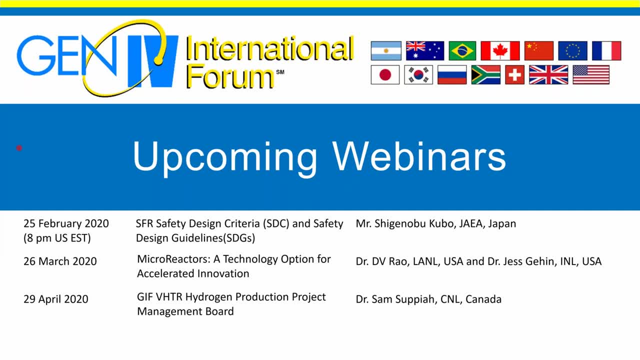 voiding in the core. in this case, the core exit flow rate can be different from the inlet flow rate and the inlet flow rate can be different from the inlet flow rate and can be even be reversible as the voids collapse. so yeah, so the, the, so the. 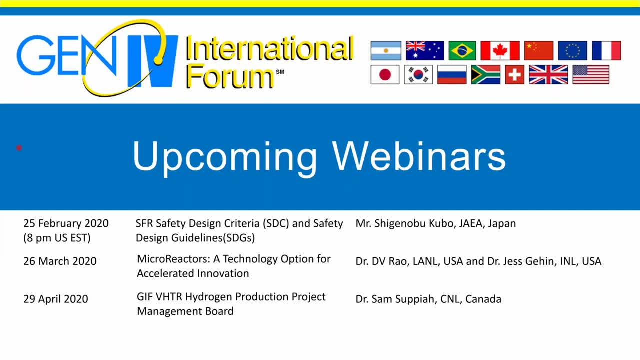 method I showed in my in my earlier said, actually only works with single phase flow and we we actually tried it in a situation where you have boiling on one of the side and not on the other, and of course it doesn't work at all. so what we? 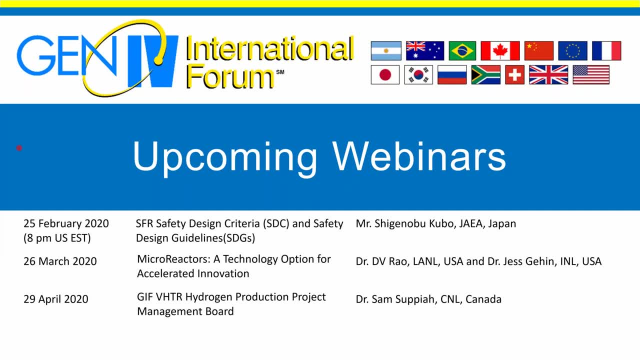 are working on right now is we want to move from this overlapping coupling you saw here to a, to what we call decomposition coupling. where you are, you take out the gray part. on the system side, you have the CFD, and then we want to use what, what? 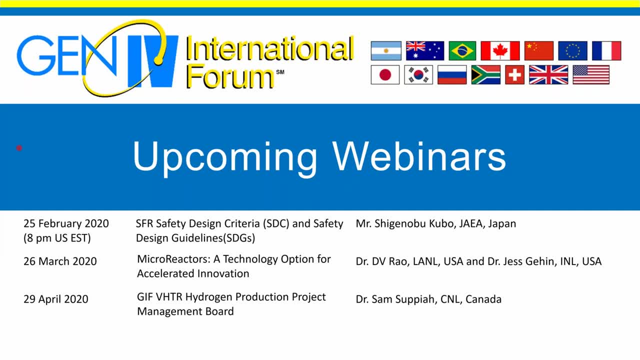 we want to use. we want to use, uh, what we call a monolithic or complete Newton coupling. so what we want to do is that, on the CFD side, we compute both what the flow would be at the next time step and we compute the derivative of this flow. 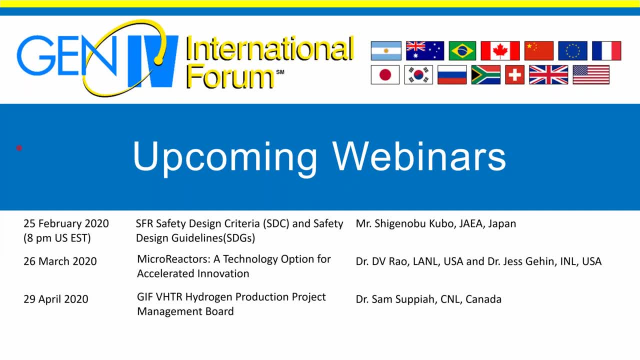 relate with the input and output pressure, and then we put both as an into the system code. we input both the numeric, the result itself and its derivatives, and so then we can do the solution on the system side and come back. so the answer is that this type of the type of coupling I showed does not work. 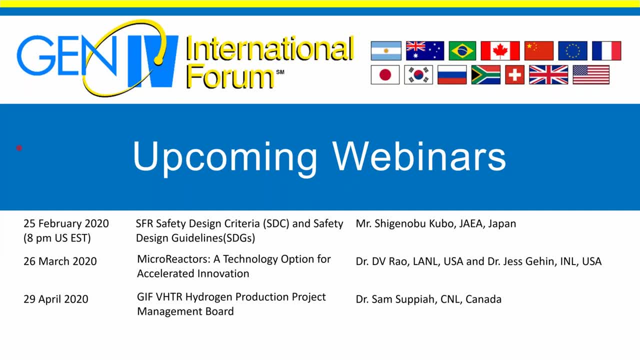 in two phase flows and the. the thing we are working on this a coupling where you you do not have overlapping between codes like this and, at the same time, you need more monolithic, tighter procedure to couple between the codes. you need to exchange more data, thank you. there's another question, similar, please, with a simulation issues. 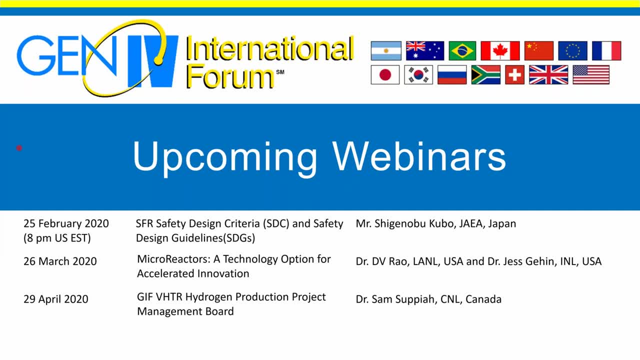 when there is two phase flow due to metal boiling. but I believe you've just addressed that. do you have any additional thought? excuse me, so this was so. these were the issues related to cut coupling for two phase flow, but of course two phase flow also need to be modeled on the thermal hydraulic side. 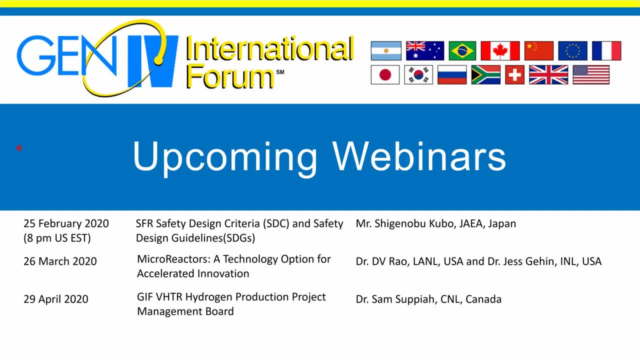 and this is very complicated. so the first, the first thing, is that the usually the, the models we, the models we have initially come from our physical understanding of water flows, and so we need to change them completely in order to do so. to do a boiling sodium, so, for instance, 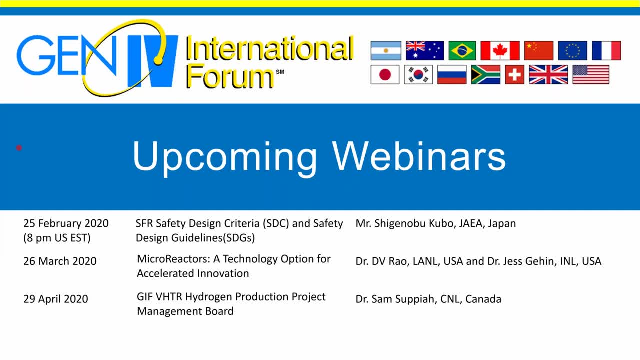 in sodium there is almost no critical heat flux. it's very rare to encounter critical heat flux and at the same time, because the liquid to vapor density ratio is very high, around 2000. it means that almost as soon as there is boiling somewhere, immediately you will have some very large pockets of gas taking all the 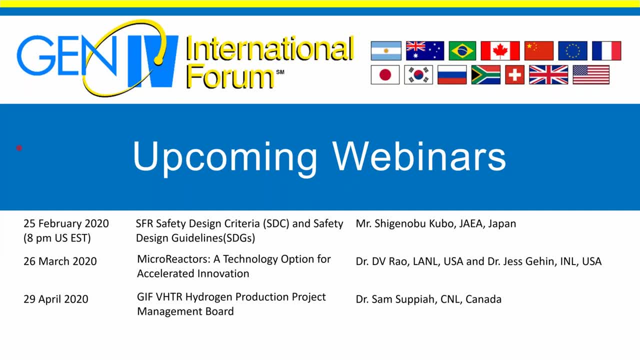 space in the sub assembly and so all the physical models for this- so to face friction, to face it, transfer, the flow map and so on- needs to be read on and actually, for in this part we are. we are collaborating as much as we can with IPP in Russia on our understanding of two-phase flow, and this is because they 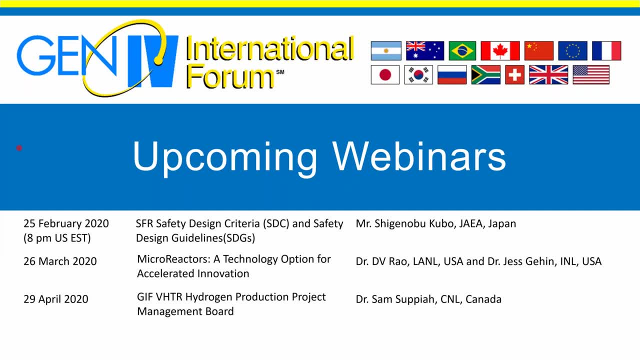 have an ongoing experimental phase flow in IPP and another. another point important point is that if you have boiling sodium in the core, then there will be a very large effect on the neutronics. so nobody if you, if you are the, know the type sodium fast reactor or 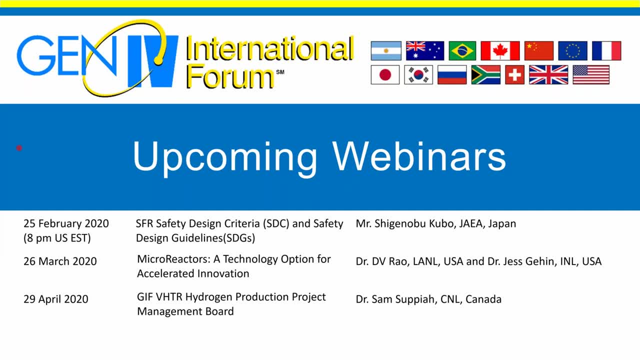 like super Phoenix or super Phoenix in France, the. these reactors have a positive but reactivity effect. so as soon as the coolant starts to boil, the reactivity increases, the boiling accelerates and you have a power extrusion in in less than one second. on the other end, in in some more recent 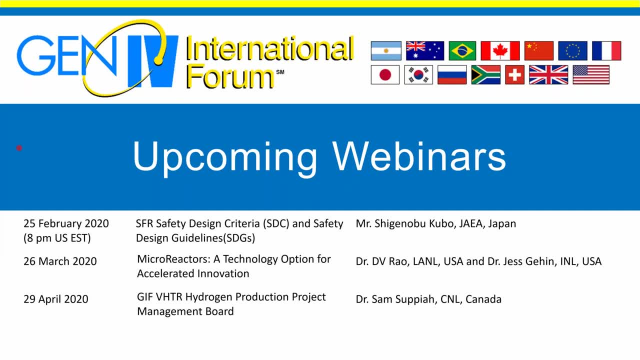 reactor design. like you, be a VN 800 or a street was also of this time being 1200, sorry- or a straighter you. we use the, we use the. this is like liquid: a sodium plenum above the core and in this case, when the sodium burns, this plenum will be replaced with with vapor, and this will 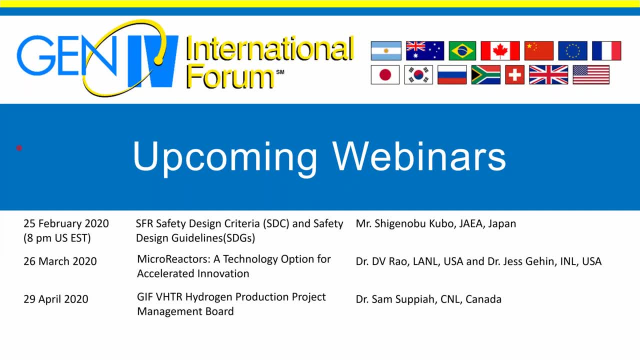 increase neutral leakage, and with this you can add: instead of a positive global void effects, you can get to a negative global void effect, and this means that as soon as the boiling starts, the power will go down, and so- but it will not go down the same way everywhere. 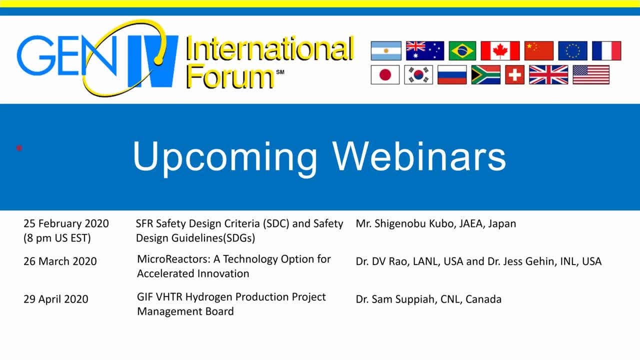 it will go down faster in the areas where the sodium is boiling, so it will be localized in a few sub assemblies, for instance, and so we need to account for very complicated coupling effect, coupled effects between neutral nicks and fiber hydraulics, usually including 3d effects, and the final one is that the 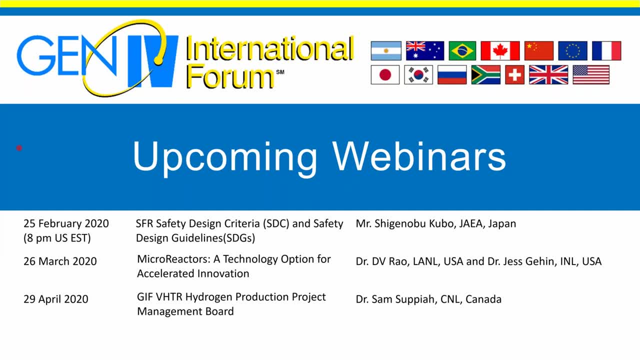 fuel mechanics will also be impacted because the fuel mechanics determine. it determines the true temperature and then the Doppler effect. you need to know what's going to happen to the fuel, to the, to the fuel thermal mechanical properties during the transient and this is also a very big issue for correct modeling. your 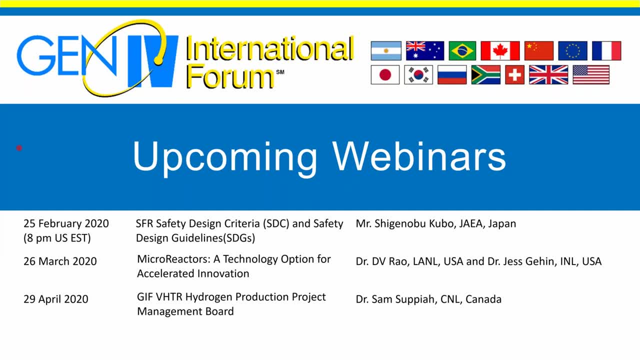 transient while the sodium points. thank you. as for the load following mode, what are the conclusions of your studies for SFRs? are material issues different than those with lwr's? well, our main experience with SFRs is that they are very short term, and so these large 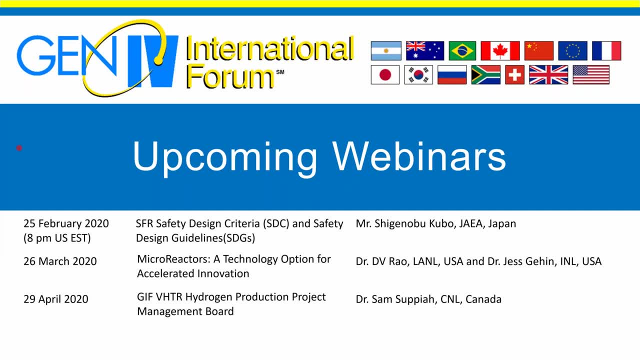 interim issues can be very long time-cancelling for FFRs when they are very short term, for that usually it's simpler than an LWR. The big difference are because of so, for instance, in all, for instance, when you look at the physical models. 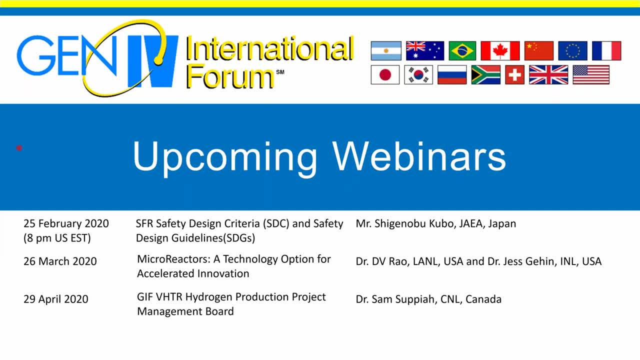 the complexity in them and so on. they are actually simpler for SFers or LFers. The only complexity comes when, because of the pool type design, you have complicated 3D phenomena and then you need to do something more. But, for instance, when we were considering 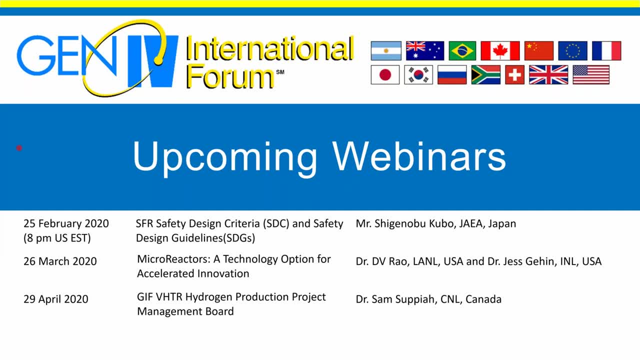 all the safety-related transients for the street project. you have all these transients where you still have the pumps operating either at nominal or on diesel power, And for all these situations we could use our system code and get good results and have validated physical models and so on. 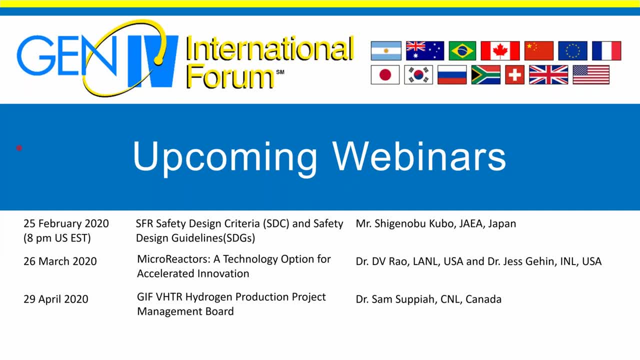 A big issue was that the models are simpler, but you still need validation experiments, right? So you need to. we needed to do a lot of literature reviews to get the best model we could, And although sometimes end up with the idea that we needed to commission a new experiment. 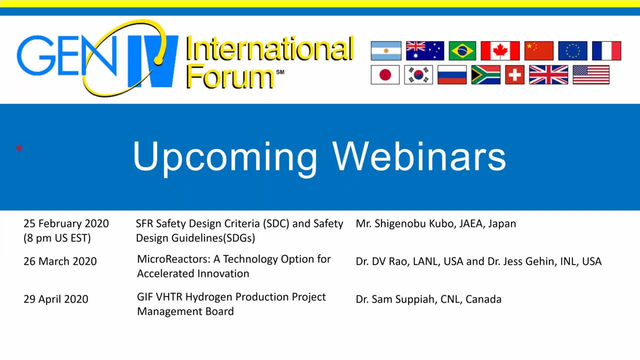 for one part or another, But overall, coming from LWR to SFers, on the system side, the big issue is this: pool type design And this is actually something you see as well in water type in modular reactors, Like if you. today we have designs for water-cooled pool type SMRs. 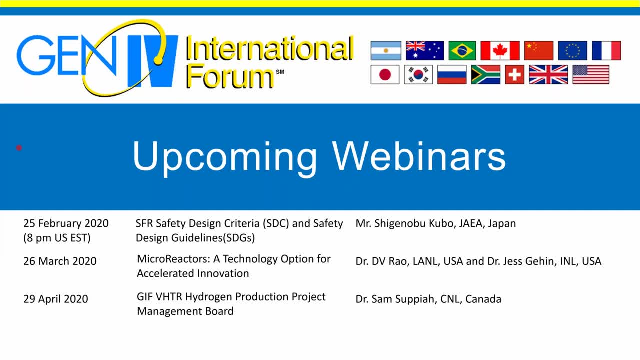 So the same idea as an SFR, actually, except you have water in the middle. And if you use a pool type design in water as well, you encounter the same problems with complicated 3D plots. So it's been an interesting journey. 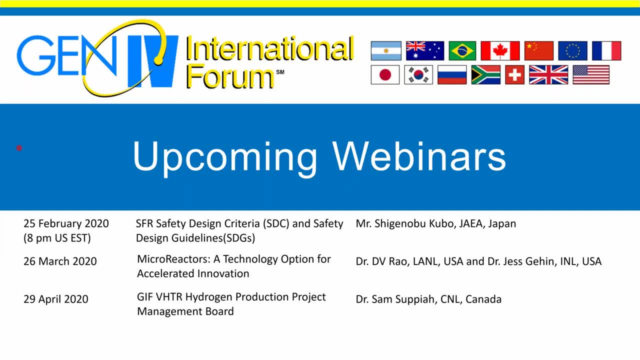 Thank you. What is the current status of validation of physical models? So at the, let's see at the in our current status, I would say that we have had the satisfactory, like what we call separate effect validation, So validation of each physical model individually. 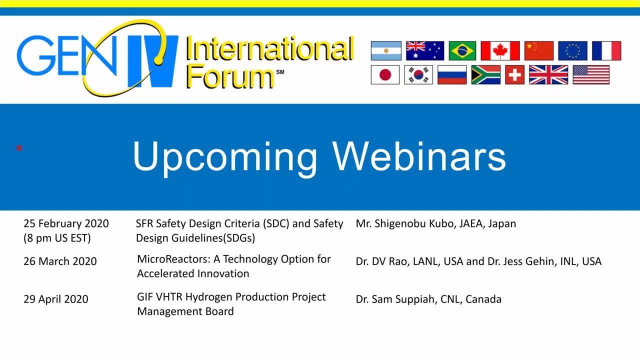 It was. we managed to get good coverage in the system code and so on. The big exception from that was, if you are the system scale, if you introduce a new component design, then we would have needed a related experiment, a scale dome experiment, of this particular geometry. 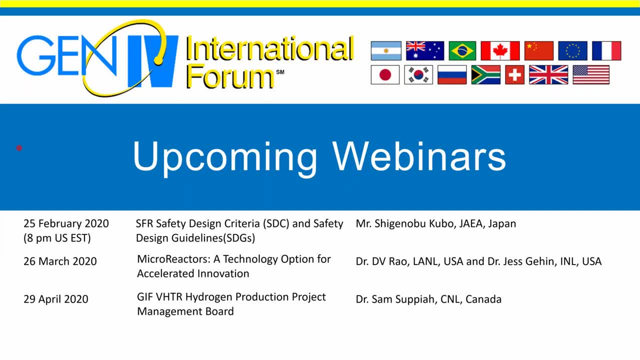 So there was the idea that we had good general validation but maybe we need some design specific validation if there was some geometry change For the validation of CFD and coupling. I think at the using all these different experiments and reactor validation and so on. 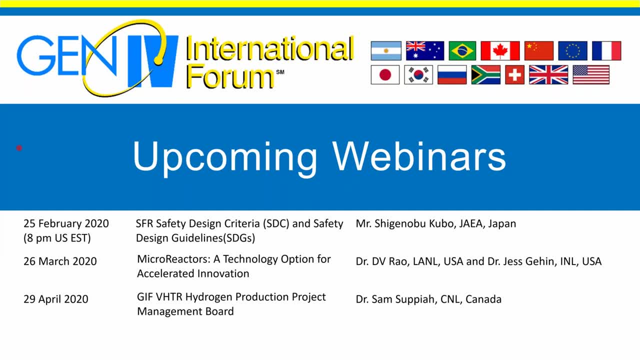 we had reached a good level of validation for a reactor scale application of this coupled simulation And actually this type of coupled situations were our reference choice for the safety report of Astrid, for instance. We would have needed more. especially, we would have needed more in case of reactor changes. 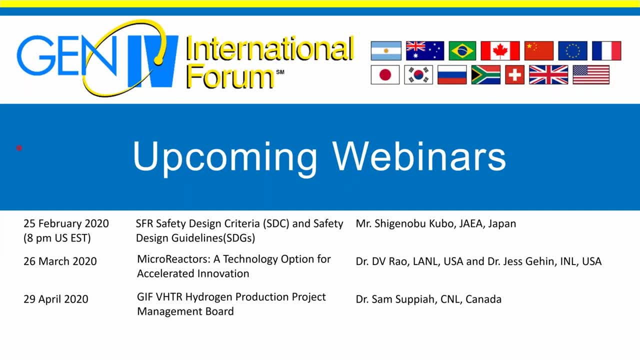 or things like that. maybe, but I don't think it would have been much. And then, of course, the- as we receive more reactor validation, it's always good to add it as well. And the big point where we need to do predictions. 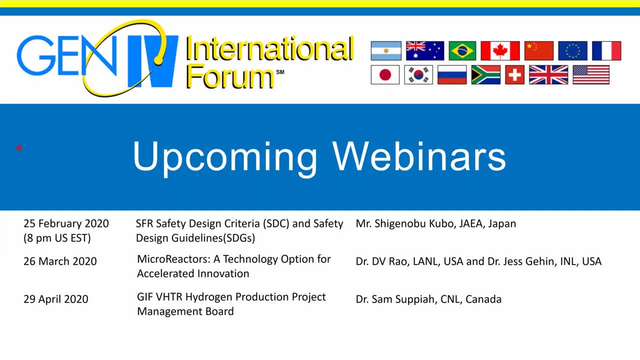 and we do not have enough validation at all. is this two-phase flow? So, on two-phase flow, we need more experimental data for the physical models, And so we have done a lot. we have done as much as we could. we need more. 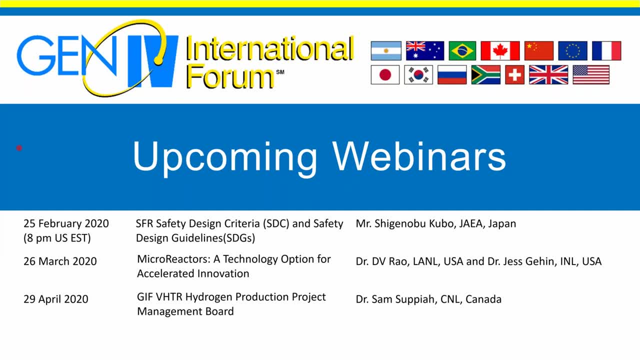 We need experimental validation for the coupled effects between formaldehyde release and neutronics and through mechanics, And we need to and we need to have the. we need this to be able to justify that in a future sodium-phase reactor, if the coolant boils, it will not lead to a severe accident. 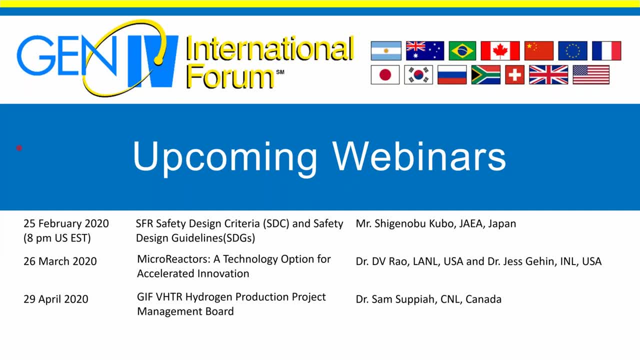 And actually for this the FFTF benchmark is very useful, because in FFTF you add an oxide core, like Astrid for instance, and oxide core have a very unfavorable Doppler effect in case of a loss of flow And in FFTF they did an unprotected transient anyway. 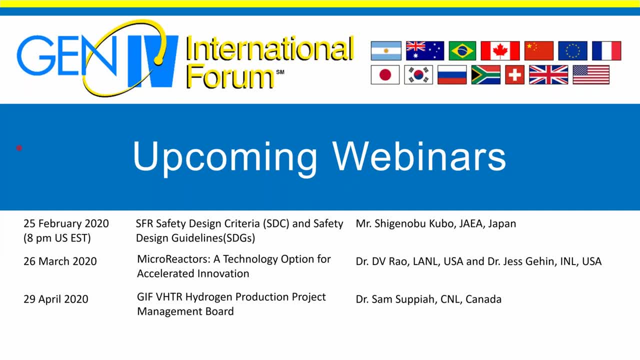 and the power. that's right, And the way they did it is that they added some extra devices on the outside of the reactor, And so these devices could mitigate what would have been otherwise a power excursion, and instead the reactor power went down all the way. 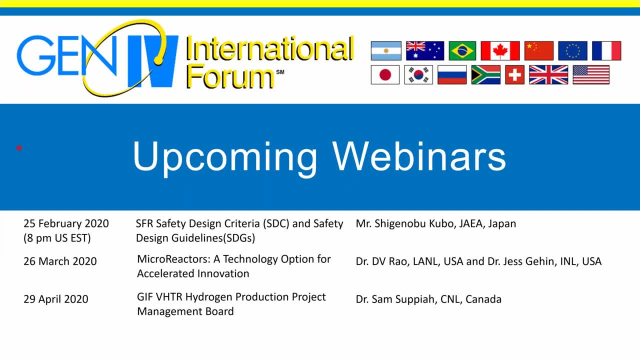 And so with this type of reactor scale multi-physics validation, we may reach a situation where we can have validated to phase flow simulations. But this is the big, the big, yeah, the big work area for the next few years. Thank you, Antoine, I forwarded you some discussion. 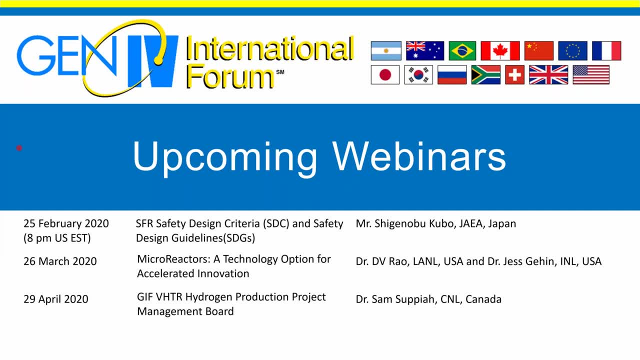 that's been posted. I don't see a question in there. is that we can have it broken down? Yeah, Can we just read and share folks? I see a question on the Yes, I see a remark from someone on the question. 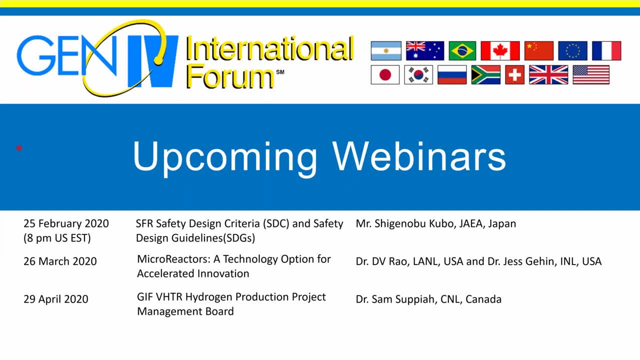 on the question side, and it's true that if you're- if you're looking at at molten salt as a, as just a coolant, that's not a fuel, the corrosion problem will be much easier. okay, i've posted it. yeah, um, and it looks like the last question i see is: 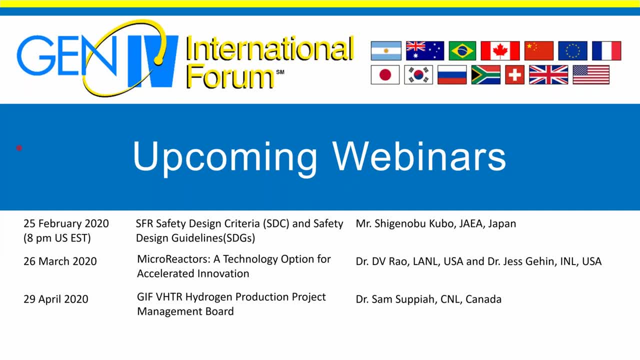 i've heard of sodium heat pipes and nasa reactor. is there any opportunity to remove decay heat using heat pipes? well, in in our case, i would say that actually, if you so, for this decay heat removal circuit, actually just using the liquid sodium, you, you, you already get a very high 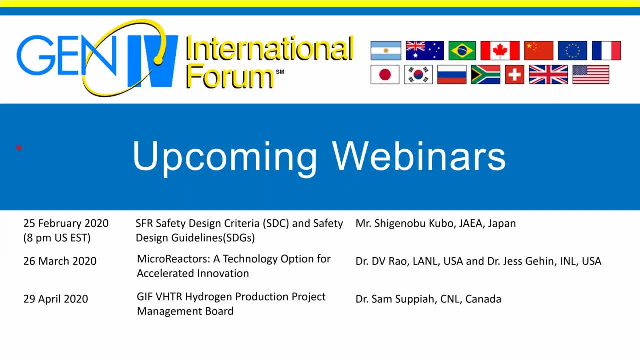 performance heat exchanger. so if you add the, i guess if you add the like a sodium cooled smr, so something smaller, then there would be an event the be an advantage in using a single pipe between the, the core, between the, the primary pool and the heat sink. so this is something you could do with a heat pipe instead of a full circuit with two. 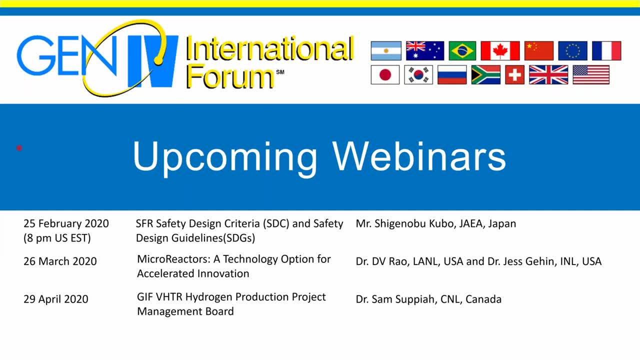 with two legs. on the other hand, for instance, even if you have a very large sodium fast reactor, like if you have, like the esfr smart project in europe, so that's a project for a 1.5 gigawatt sodium fast and you only need i think, um, yeah, you, you can remove something like six or seven megawatts. 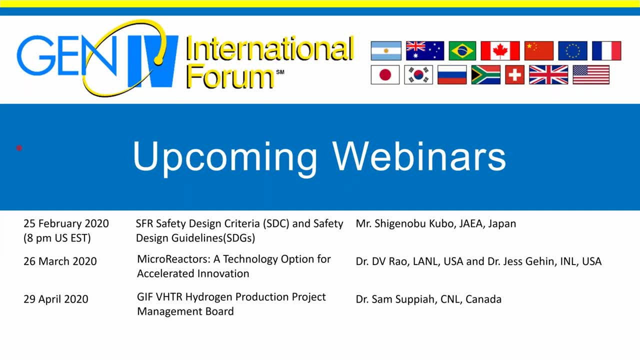 per heat exchanger in the chimney and in this case it's it's easier to just do two legs and keep liquid sodium. a thing that may be complicated with a heat pipe is that if you want liquid sodium on the primary side and you put a heat pipe in, you will need to. 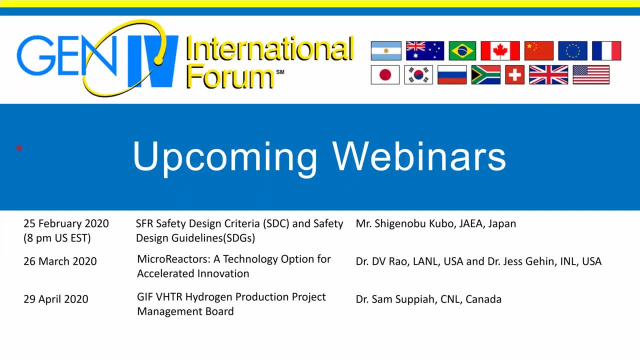 to put the sodium at less than ambient pressure and you might. you may have issues of about coming while ingress- ingress of air inside the pipe, something like that. so i think it would be it's easier to just have a liquid circuit and its own little purification and sodium, but it's uh, for a smaller reactor it could be interesting. 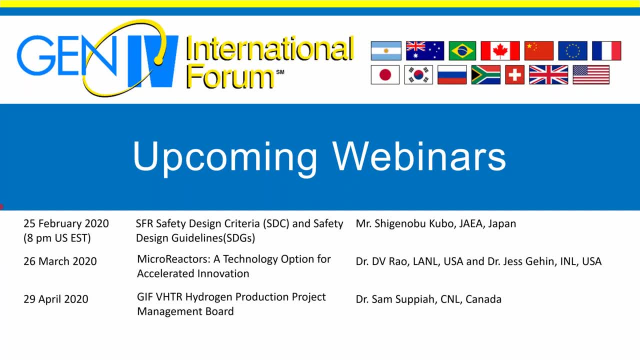 you've received lots of accolades and thank yous- was a wonderful presentation today. thank you again for your um sharing your expertise with us. uh, it's always. it's always good to see so many engaged participants with the number of questions very interesting topic. thank you. 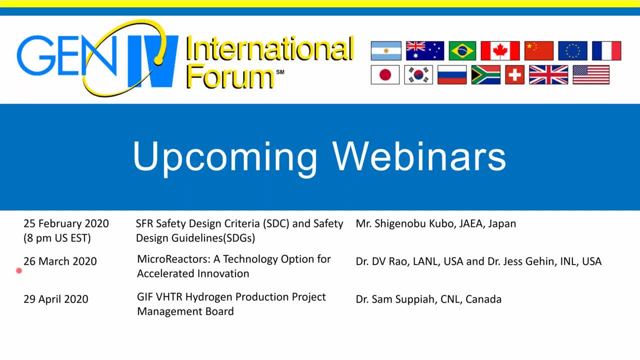 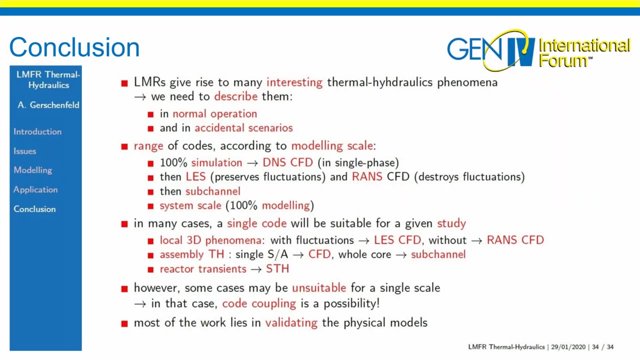 yes, thank you again, antoine. it was really good, and what is really interesting is this: q a station, a strong momentum, good dynamic. thank you, antoine, thank you, and so, with that presentation, thank you all for joining, thank you, bye-bye, bye-bye. 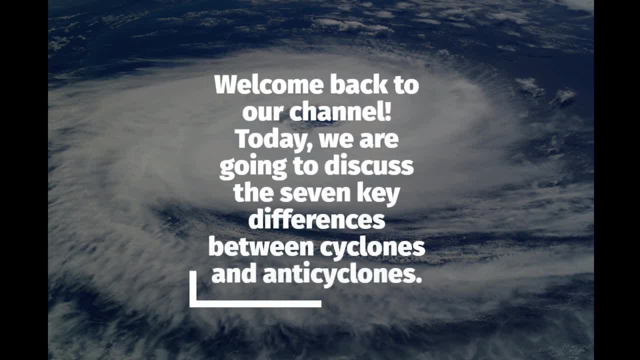 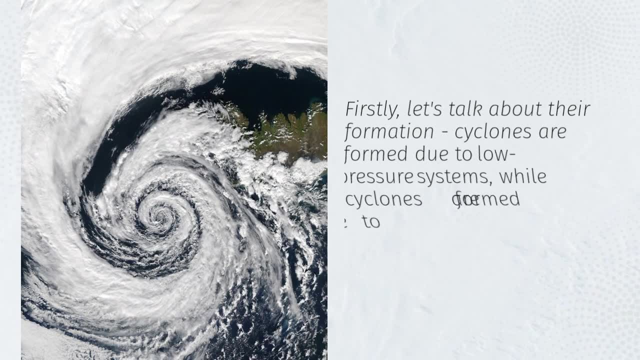 Welcome back to our channel. Today, we are going to discuss the 7 key differences between cyclones and anticyclones. Firstly, let's talk about their formation. Cyclones are formed due to low-pressure systems, while anticyclones are formed due to high-pressure systems. 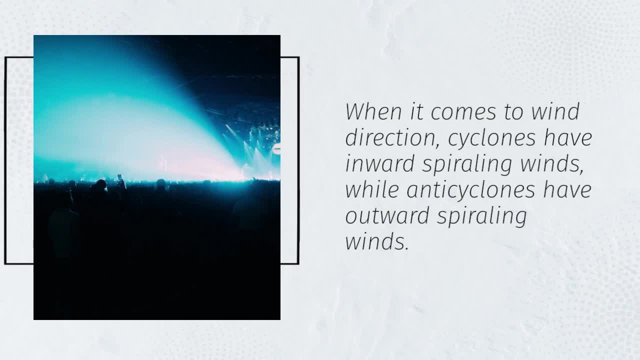 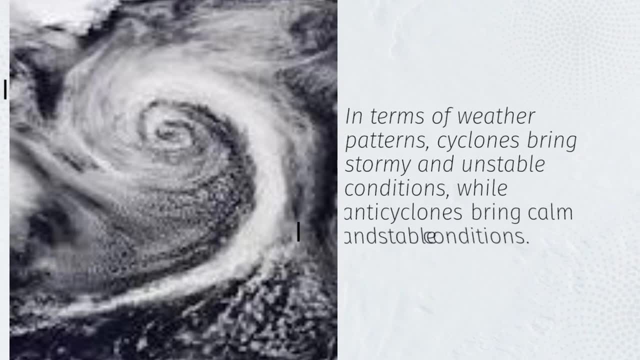 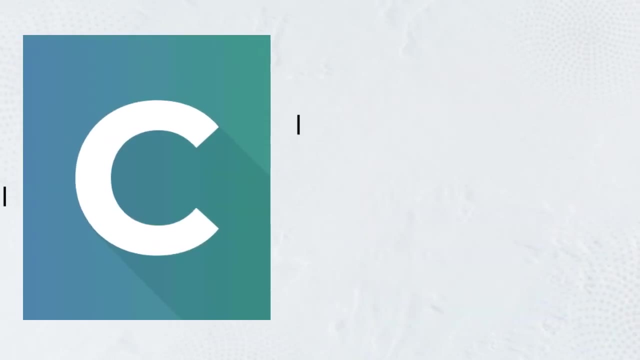 When it comes to wind direction, cyclones have inward-spiraling winds, while anticyclones have outward-spiraling winds. In terms of weather patterns, cyclones bring stormy and unstable conditions, while anticyclones bring calm and stable conditions. Cyclones are associated with 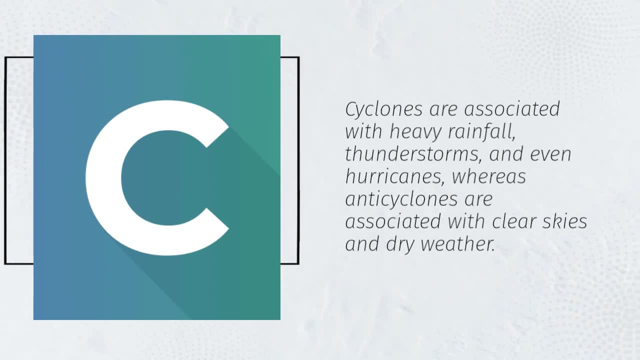 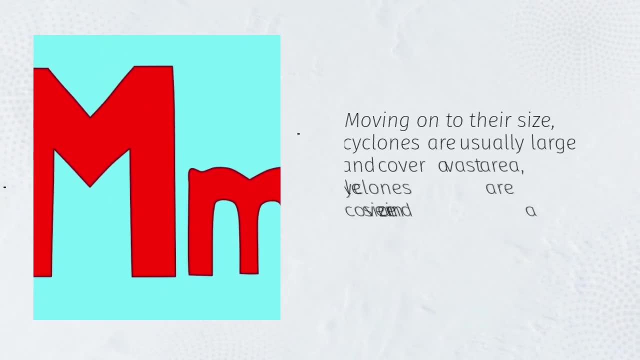 heavy rainfall, thunderstorms and even hurricanes, whereas anticyclones are associated with clear skies and dry weather. Moving on to their size, cyclones are usually large and cover a vast area, while anticyclones are smaller in size and cover a relative 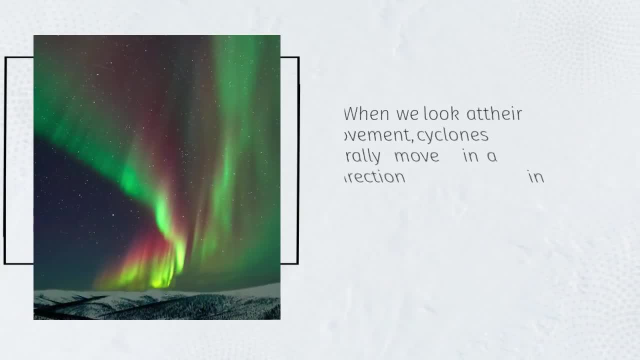 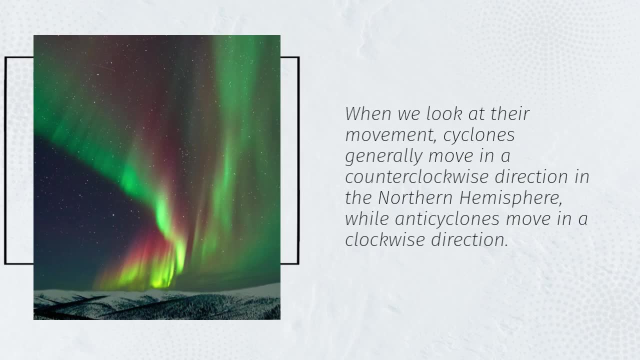 smaller area. When we look at their movement, cyclones generally move in a counterclockwise direction in the northern hemisphere, while anticyclones move in a clockwise direction. Cyclones tend to have a low-pressure center, while anticyclones have a high-pressure center. Another important difference is in their air masses. Cyclones have warm air rising and cold air sinking, whereas anticyclones have cold air descending and warm air rising. Lastly, cyclones tend to have a low-pressure center, while anticyclones have a high-pressure center. 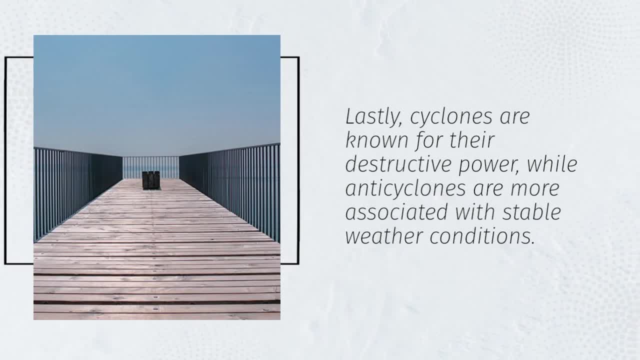 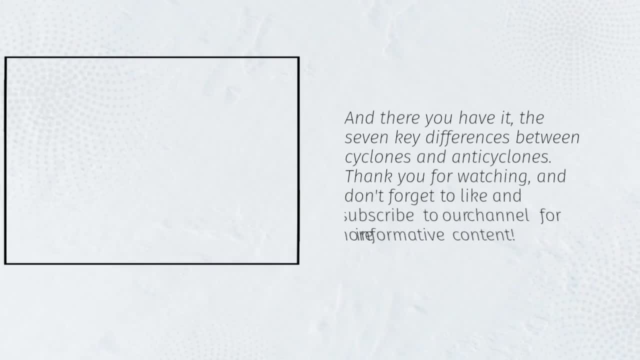 Cyclones are known for their destructive power, while anticyclones are more associated with stable weather conditions. And there you have it: the seven key differences between cyclones and anticyclones. Thank you for watching, and don't forget to like and subscribe to our channel for.